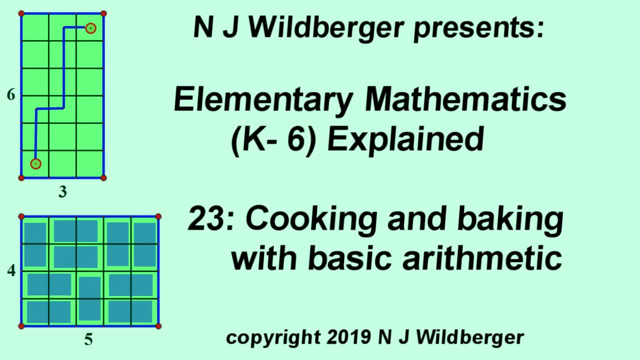 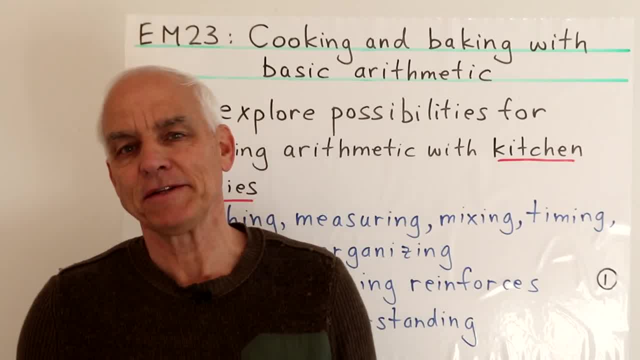 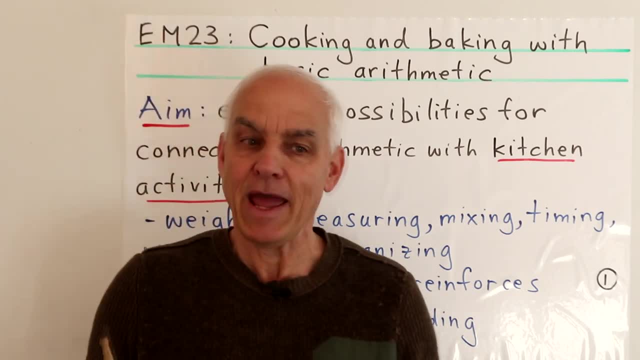 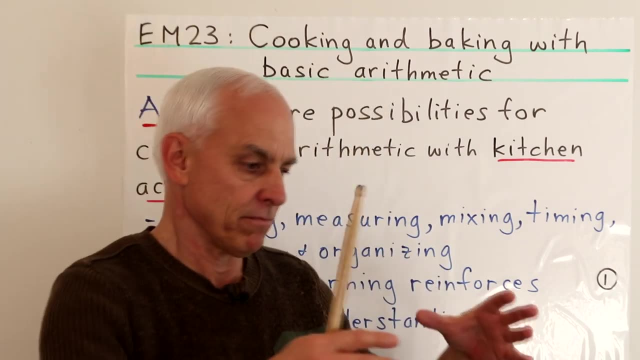 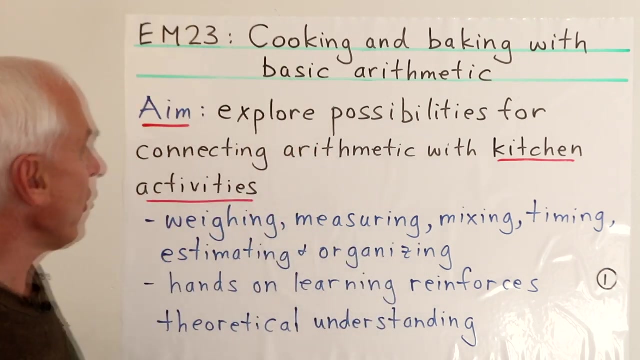 Welcome everyone. I'm Norman Walburger, and today we're going to explore how mathematics and activities in the kitchen, like cooking and baking, can be brought together to strengthen students' understanding of somewhat theoretical arithmetic, connecting it to practical activities which end up with tasty and interesting results. So we're going to explore the possibilities of 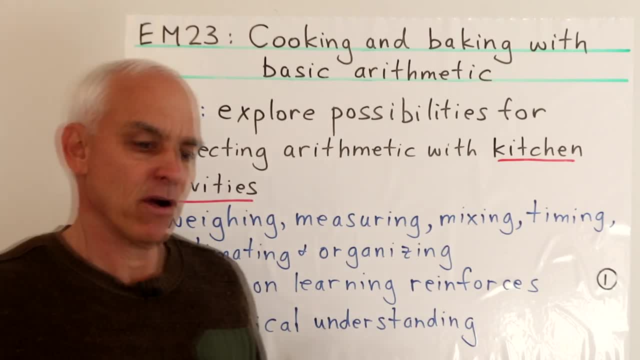 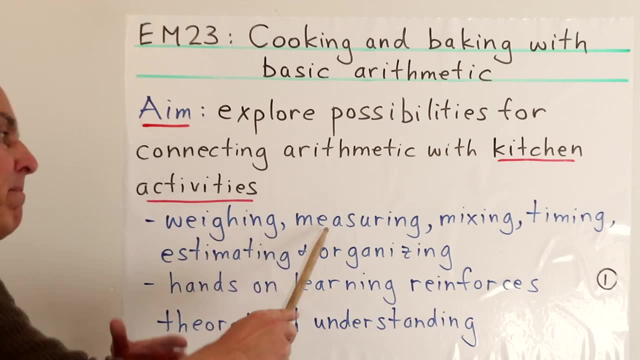 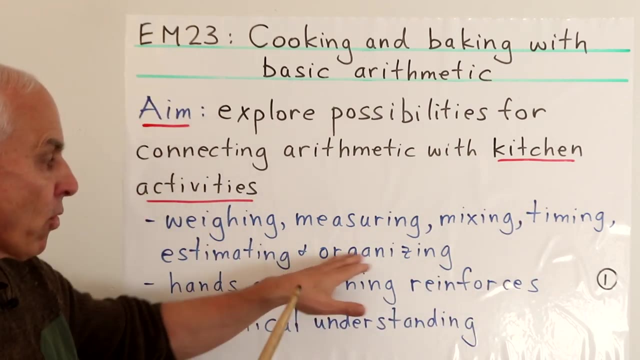 connecting arithmetic with kitchen, and involved in that are various processes that naturally have an arithmetical or mathematical aspect, For example weighing things, measuring things, perhaps volumes, mixing, timing, estimating and organizing. So these are hands-on learning. 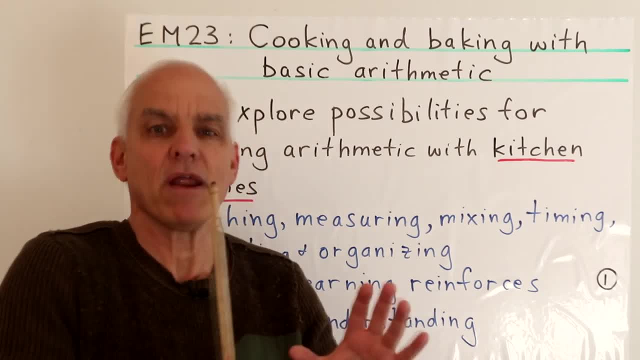 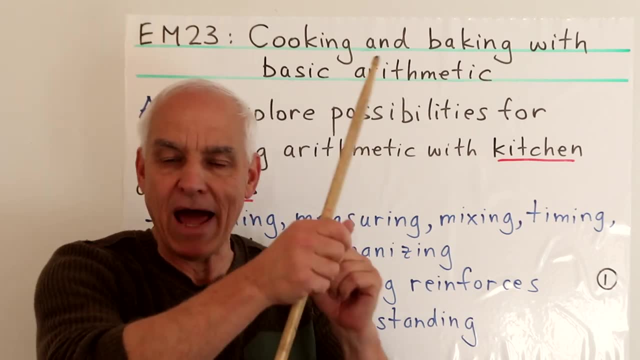 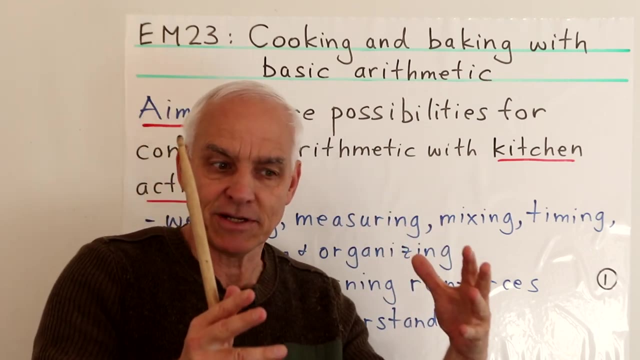 activities, and this is a great way of reinforcing somewhat theoretical understanding. It's one thing to learn arithmetic with flashcards or blackboard exercises and so on. It's quite another to see those abstract concepts directly applied and in fact sort of necessary for something important. 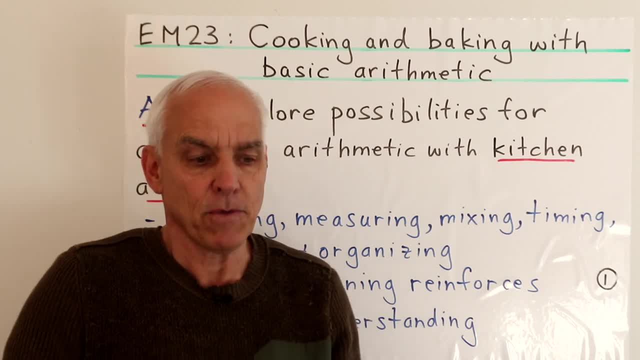 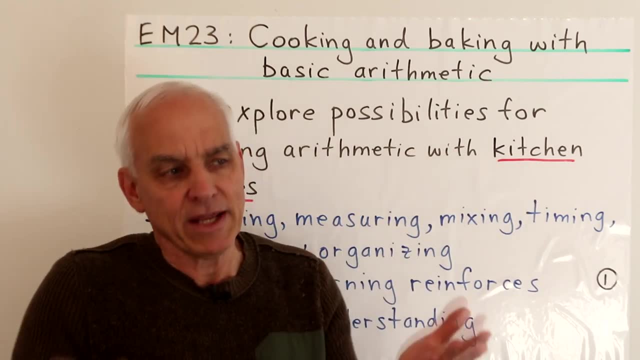 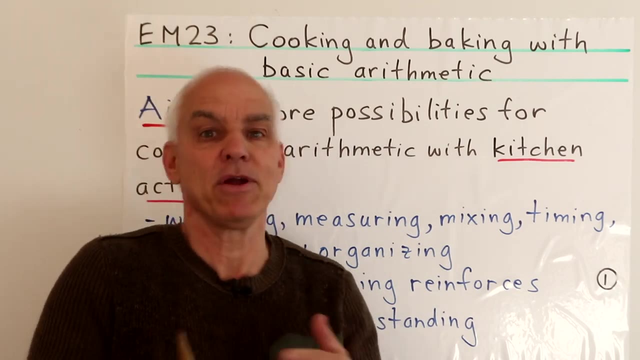 like preparing food. Okay, so this is a little bit different from some of the other lectures. I'm going to be contacting ordinary life a little bit more, hopefully getting you to think about other ways in which really ordinary daily activities can be connected with mathematics. to illustrate: 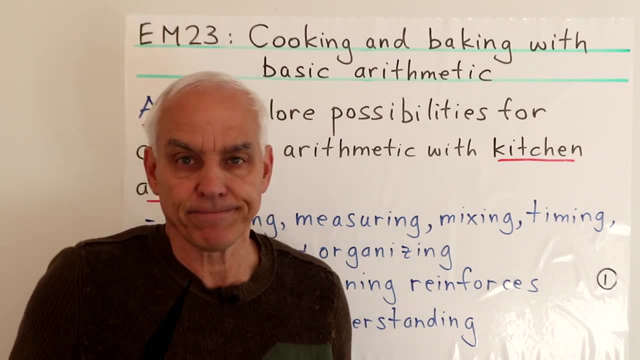 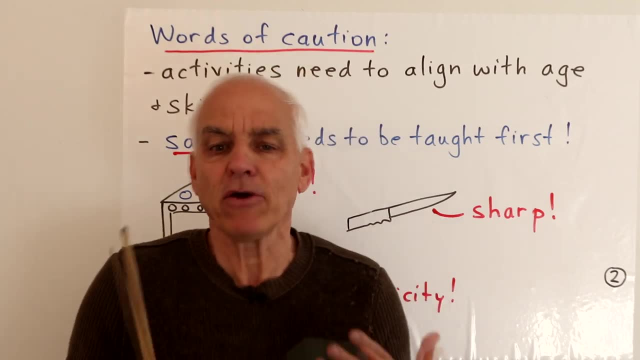 the power of the subject for everyday life. Now, most of what I'm going to be saying today really applies more, perhaps, to parents than it does to teachers, because parents can more readily implement the ideas that we're talking about, because you can get your child in the 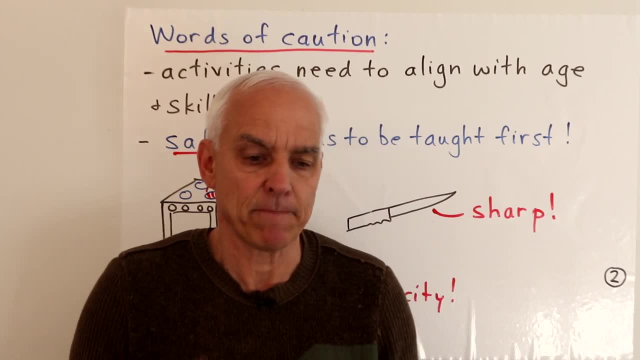 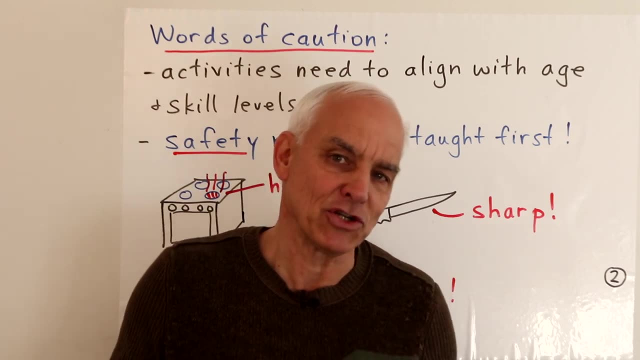 classroom, helping you to cook things or to bake something In a classroom. it's not so clear, at least to me, how to implement these ideas, but it seems like an interesting challenge and perhaps some of you will have some ideas of how we might do that sort of with a larger group. 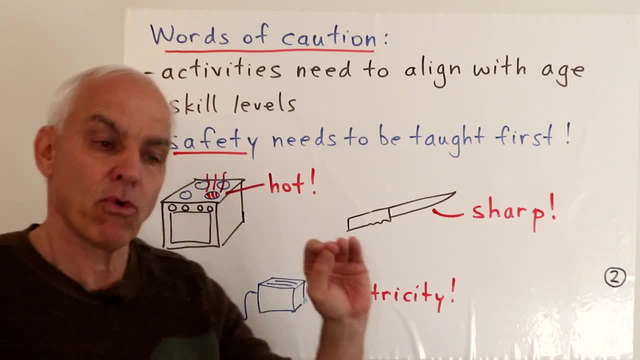 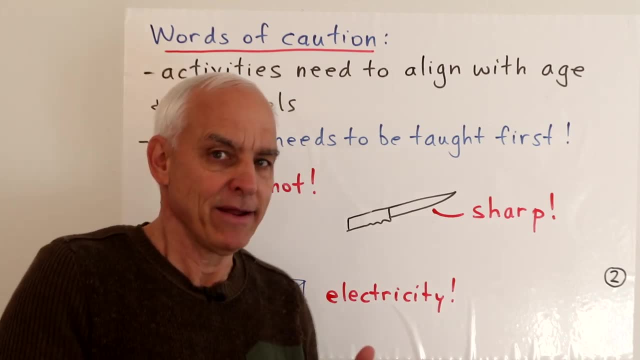 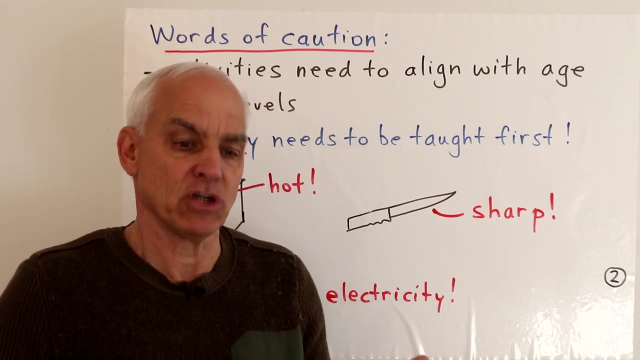 of children. But before we start, probably some words of caution just to remind you are useful, That in the kitchen there are some potentially dangerous things, so safety concerns need to be foremost in our minds. We have to teach young children, especially very young. 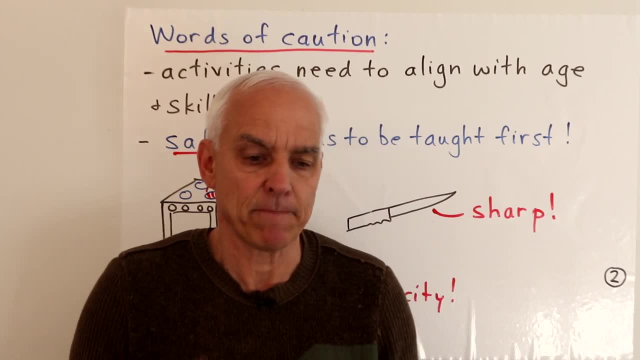 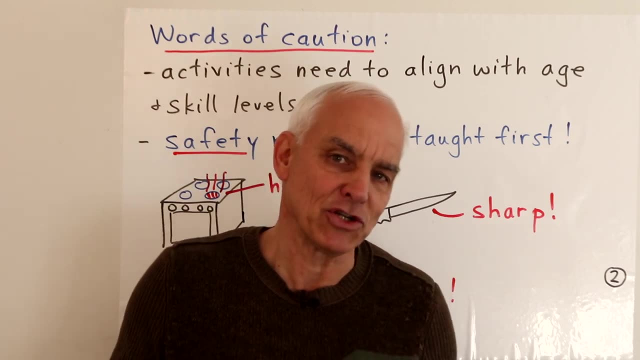 classroom, helping you to cook things or to bake something In a classroom. it's not so clear, at least to me, how to implement these ideas, but it seems like an interesting challenge and perhaps some of you will have some ideas of how we might do that sort of with a larger group. 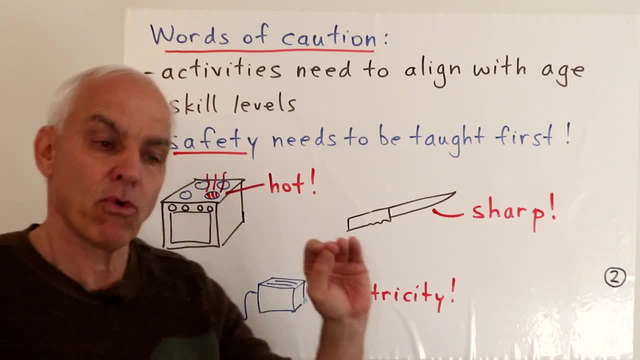 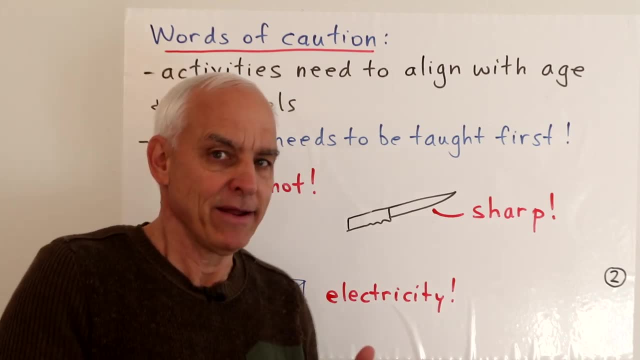 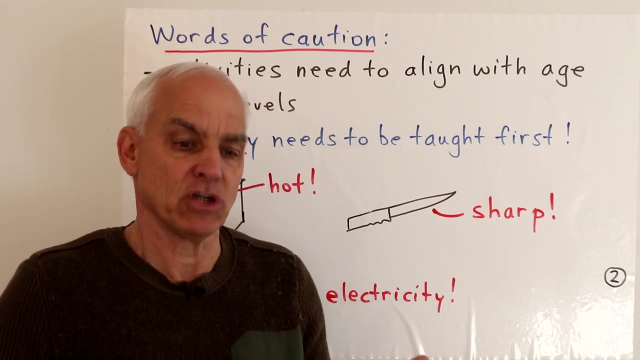 of children. But before we start, probably some words of caution just to remind you are useful, That in the kitchen there are some potentially dangerous things, so safety concerns need to be foremost in our minds. We have to teach young children, especially very young. 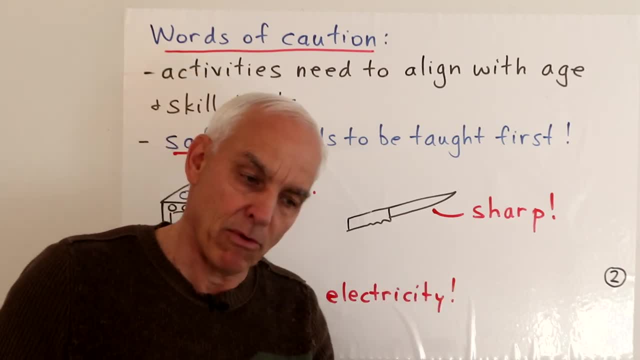 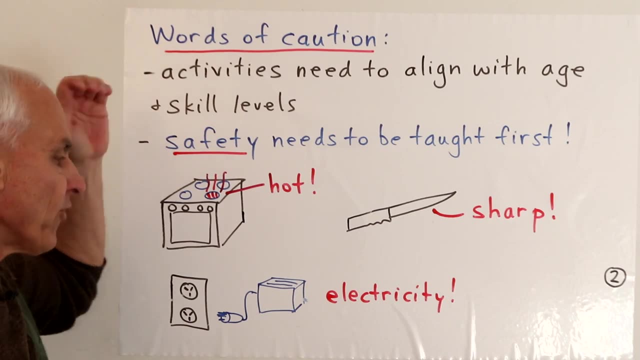 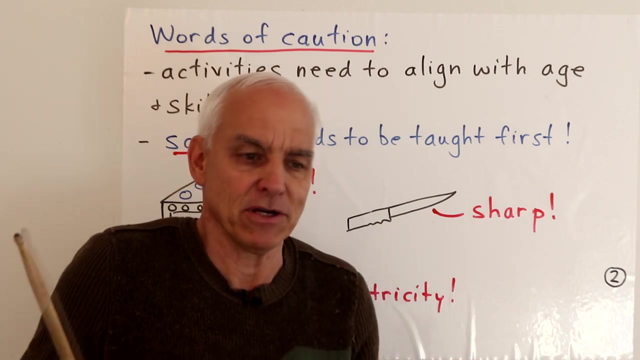 children about the potential dangers in the kitchen, to make them aware of it, to make them careful in contact with things. And also it's useful to say that we're covering K-6.. It's quite a wide range of children's ages, maybe from five years to 12 years, something like that. 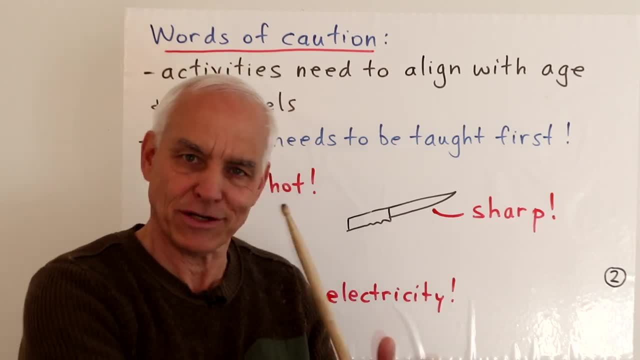 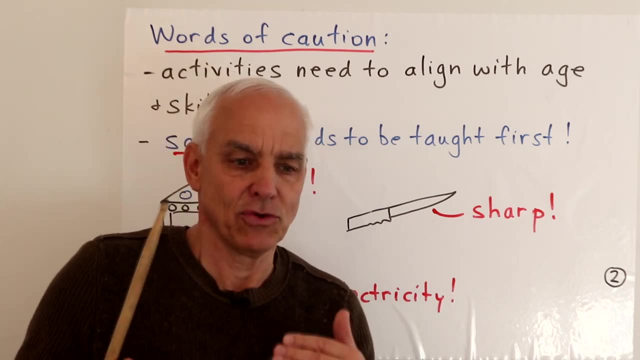 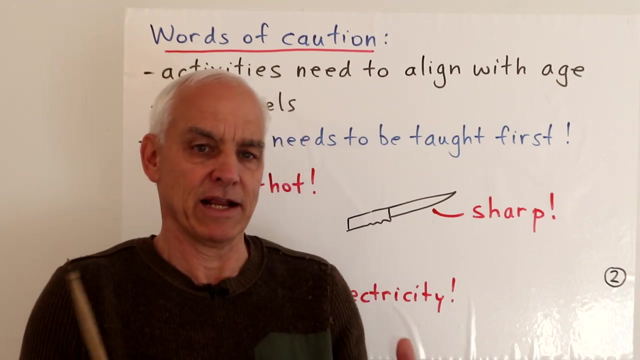 And so some of these activities are definitely more oriented towards the younger cohort, while others may be more suitable for the older cohort. So you'll have to use your judgment as to the level of sophistication or age or maturity of your child in terms of what kinds of things would 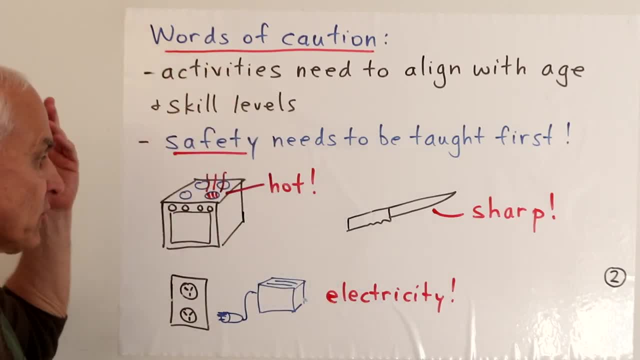 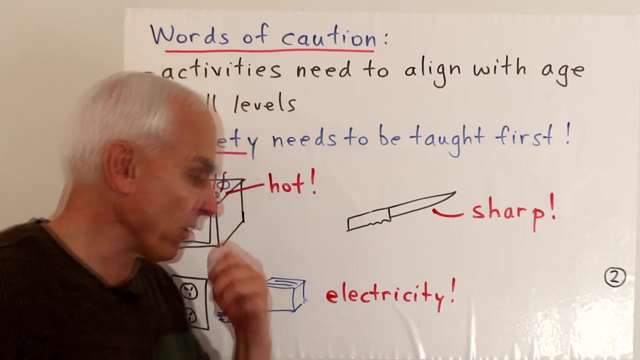 likely be successful for them. Okay, so safety issues. There's really sort of three things that sort of spring to mind immediately. First and foremost, that when you're cooking or baking, there's hot things around: hot stoves, hot ovens or maybe just hot pans or boiling water, et cetera. 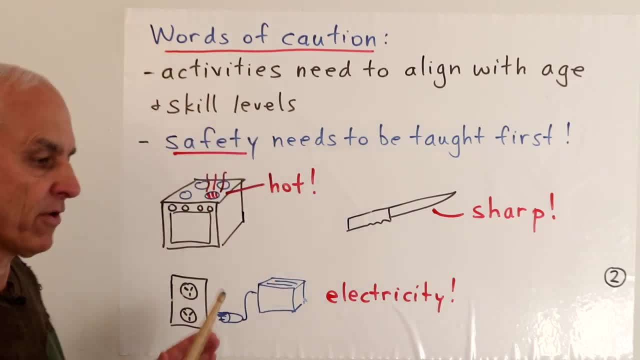 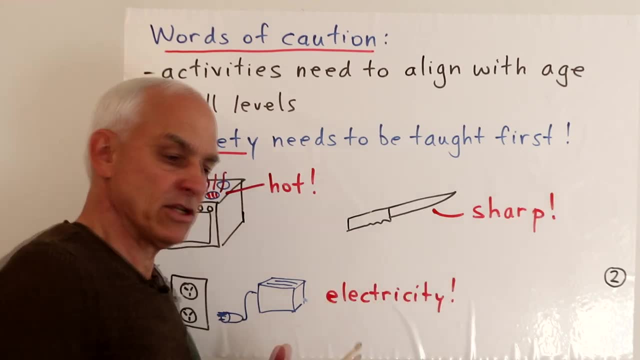 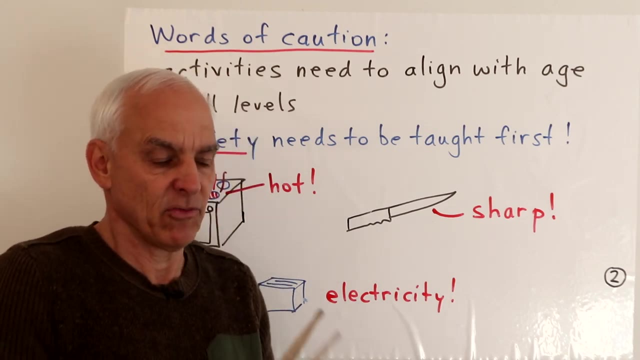 So kids need to be made aware of the dangers and potential dangers of hot things. Another obvious kind of safety issue is using knives and cutting things. Knives are sharp, so students have to be taught how to use knives in a responsible and careful way, And there again, you may want to judge. 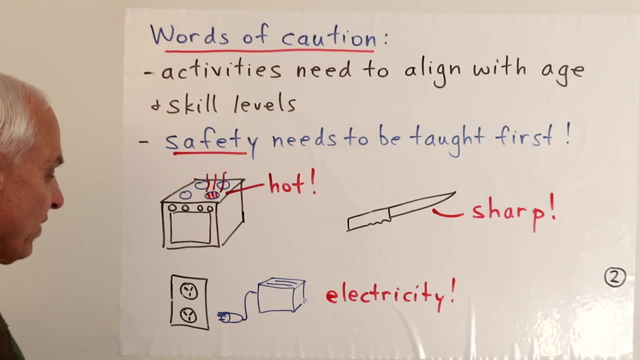 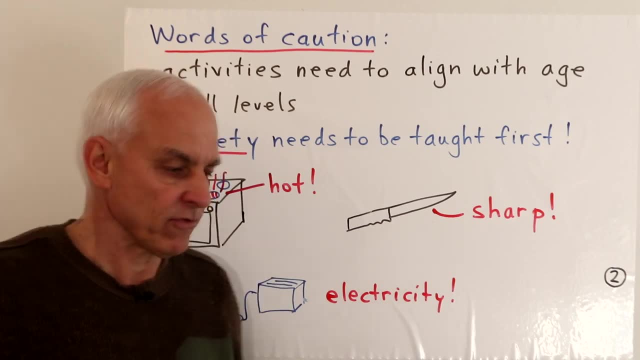 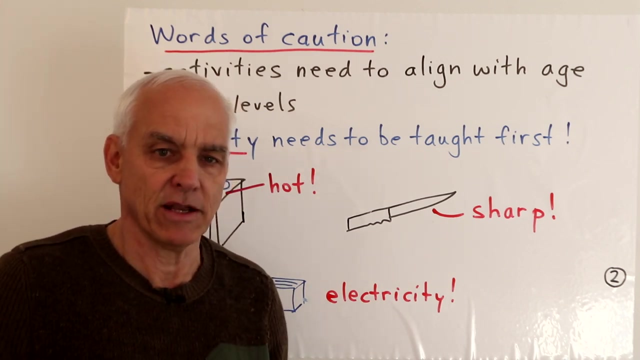 depending on the age of your child. A third, maybe less obvious but still important issue is connecting things to electricity, So we have to be careful about outlets. We also have to be careful about ensuring that liquids et cetera don't spill onto things which are plugged in And 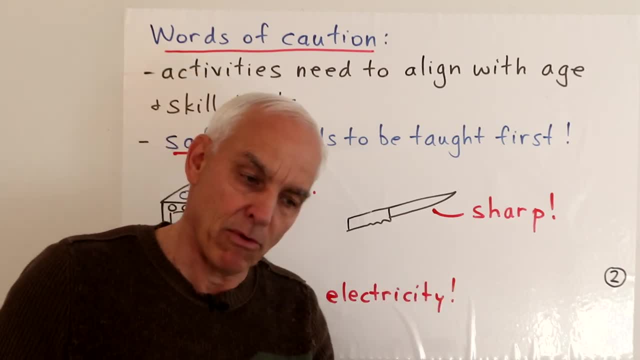 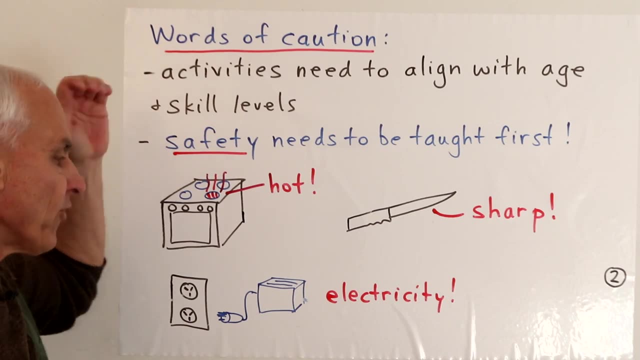 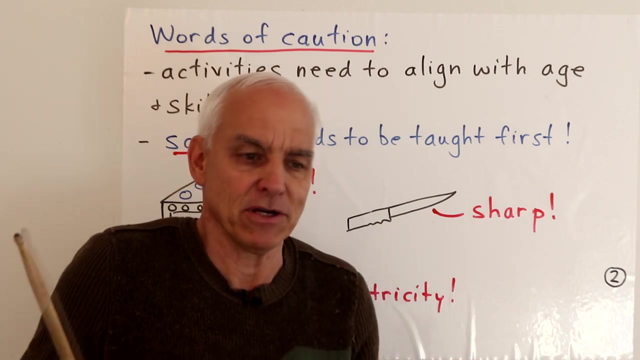 children about the potential dangers in the kitchen, to make them aware of it, to make them careful in contact with things. And also it's useful to say that we're covering K-6.. It's quite a wide range of children's ages, maybe from five years to 12 years, something like that. 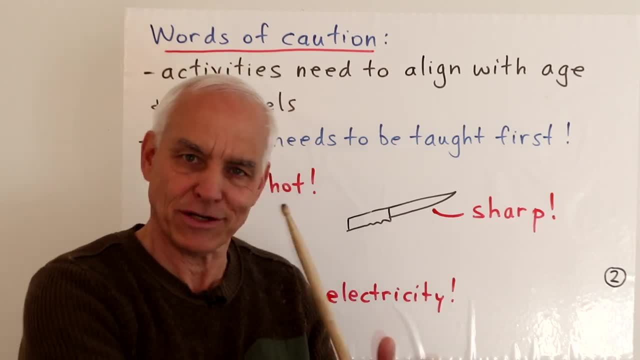 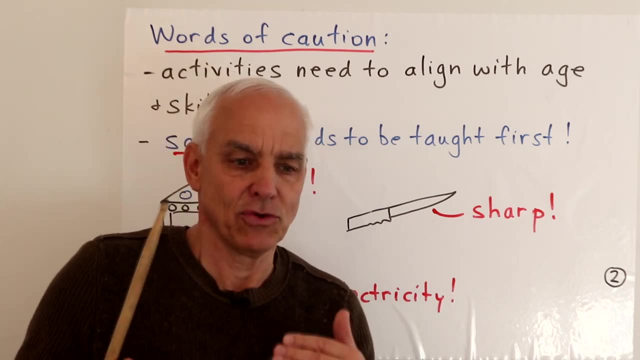 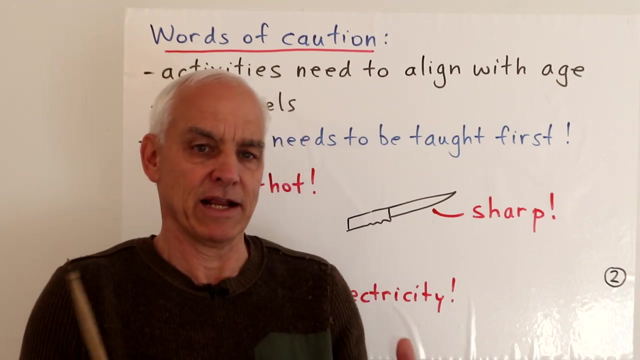 And so some of these activities are definitely more oriented towards the younger cohort, while others may be more suitable for the older cohort. So you'll have to use your judgment as to the level of sophistication or age or maturity of your child in terms of what kinds of things would 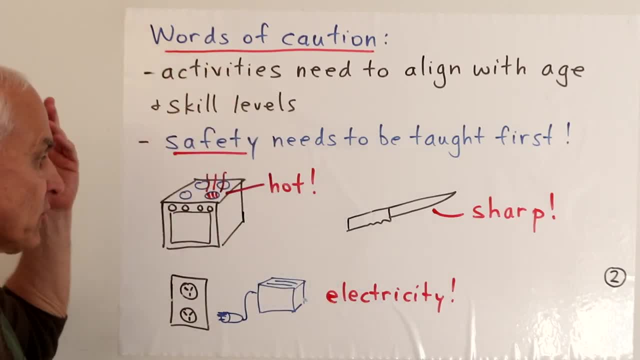 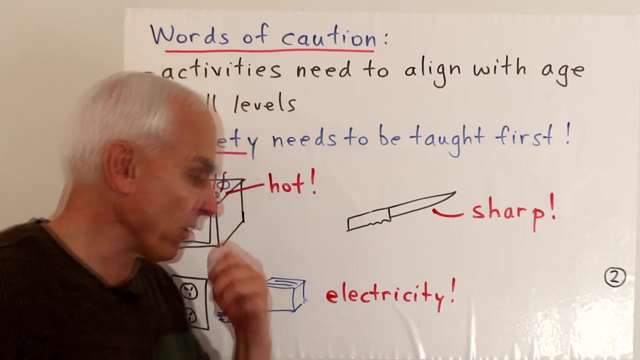 likely be successful for them. Okay, so safety issues. There's really sort of three things that sort of spring to mind immediately. First and foremost, that when you're cooking or baking, there's hot things around: hot stoves, hot ovens or maybe just hot pans or boiling water, et cetera. 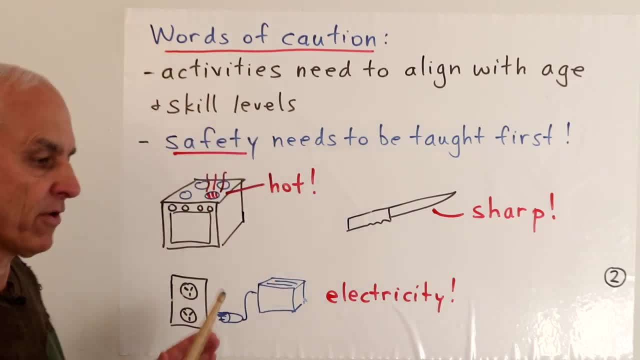 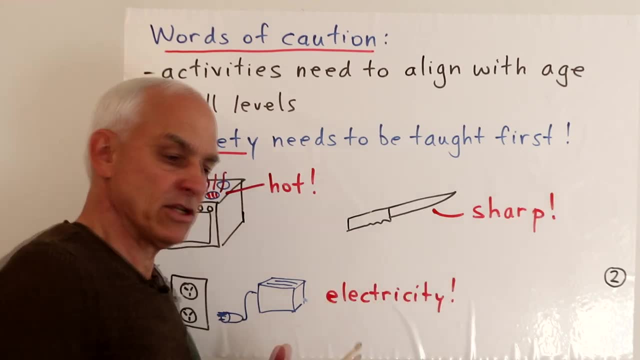 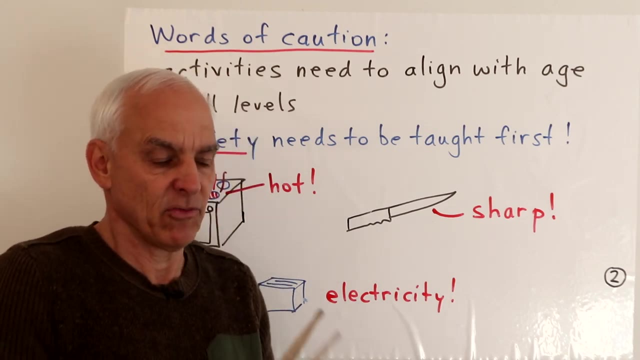 So kids need to be made aware of the dangers and potential dangers of hot things. Another obvious kind of safety issue is using knives and cutting things. Knives are sharp, so students have to be taught how to use knives in a responsible and careful way, And there again, you may want to judge. 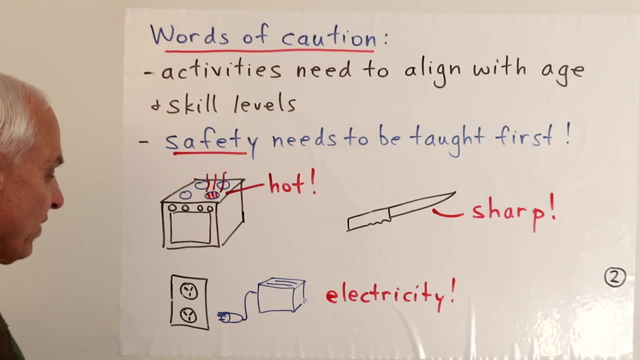 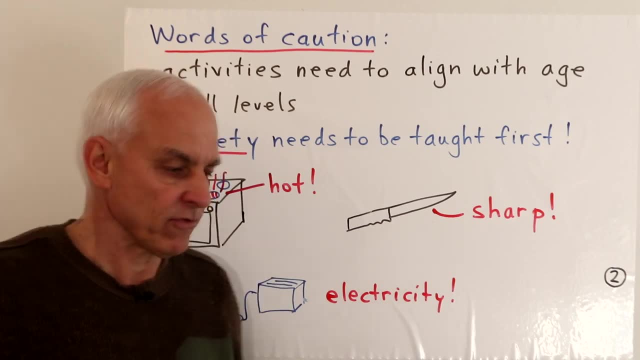 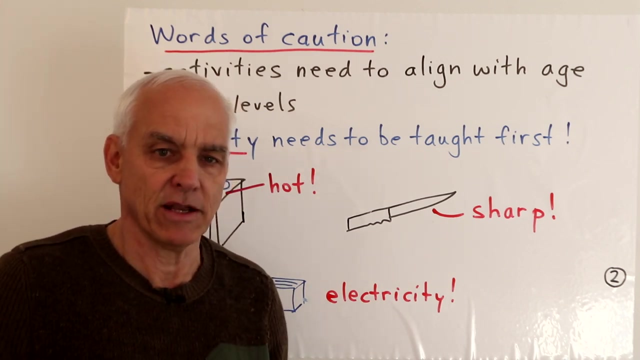 depending on the age of your child. A third, maybe less obvious but still important issue is connecting things to electricity, So we have to be careful about outlets. We also have to be careful about ensuring that liquids et cetera don't spill onto things which are plugged in And 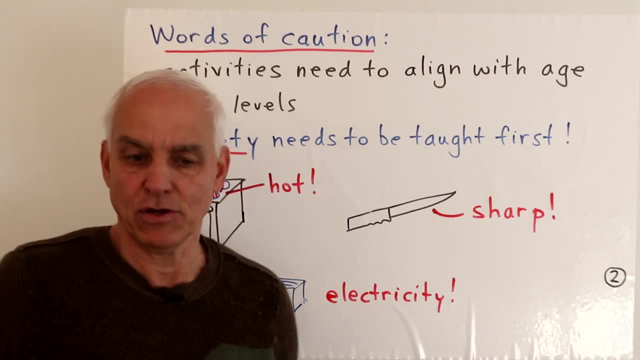 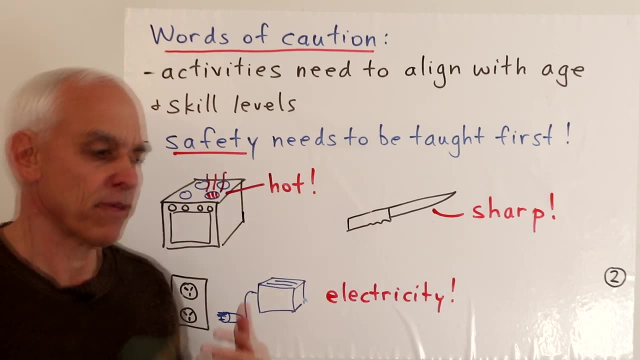 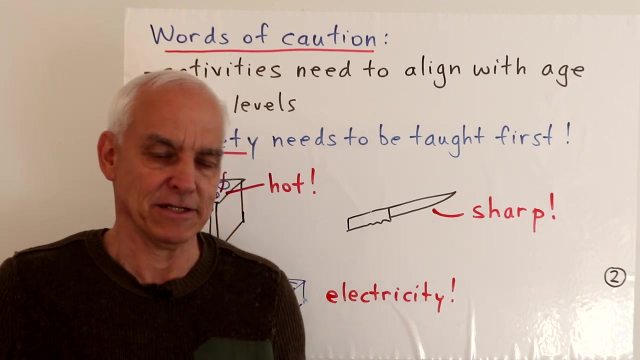 we have to be just generally aware of the potential dangers in using electrical implements. So it's probably a good idea just to make sure that your child is aware of these three kind of issues- maybe others that you can think of- so that everything that we do is in a safe and 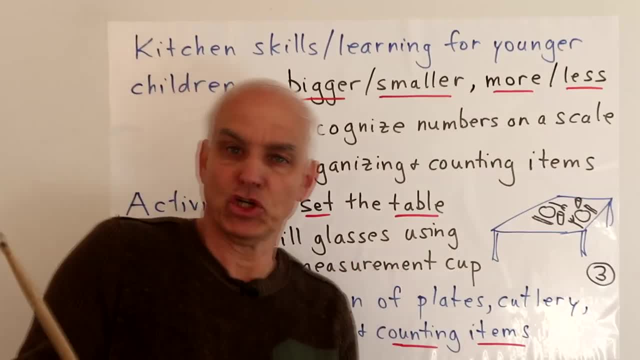 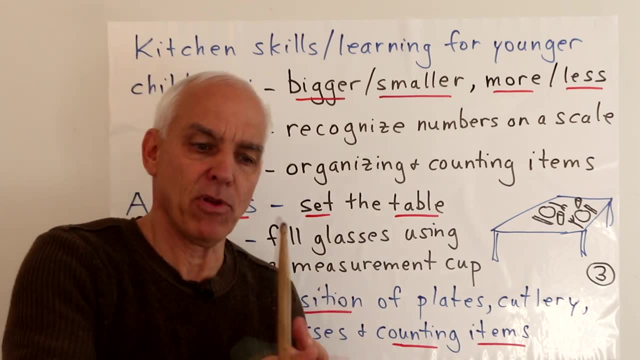 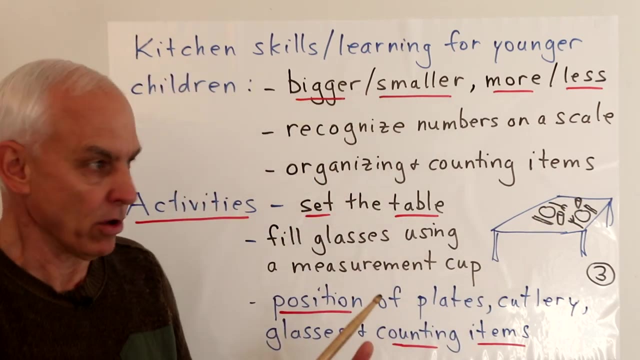 careful context. So let's start with sort of younger children, maybe K, first year, second year. These kinds of children can be introduced to very simple kinds of concepts in the context of the kitchen, For example, notions like bigger and smaller, more or less. These are easily. 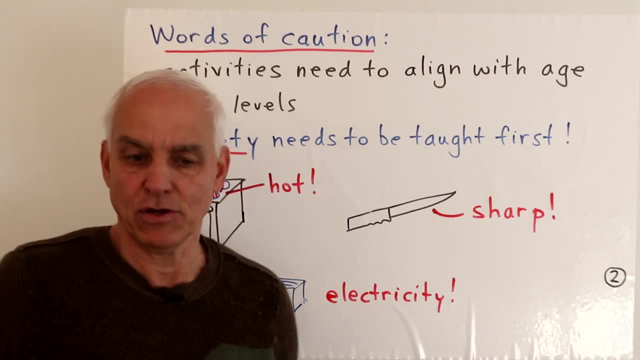 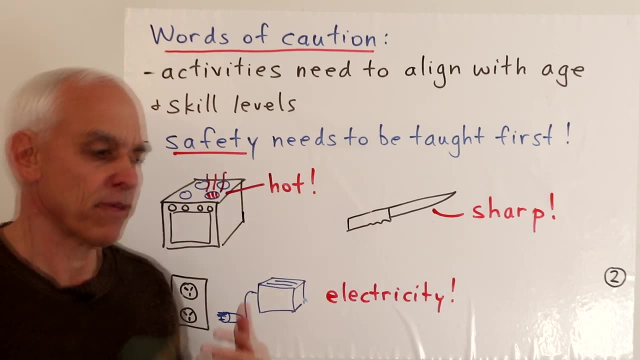 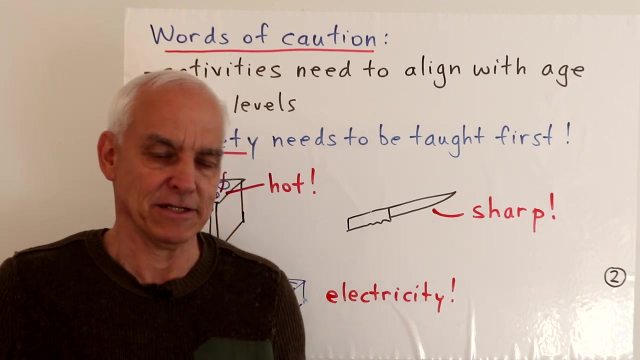 we have to be just generally aware of the potential dangers in using electrical implements. So it's probably a good idea just to make sure that your child is aware of these three kind of issues- maybe others that you can think of- so that everything that we do is in a safe and 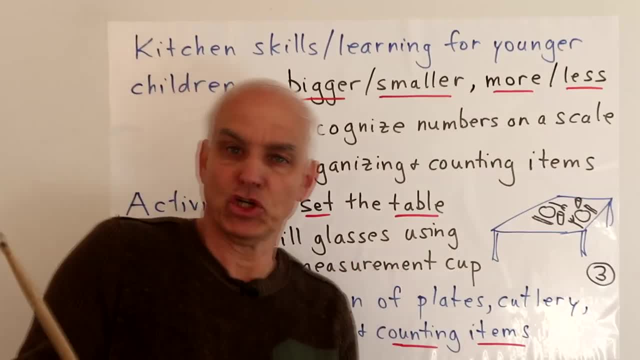 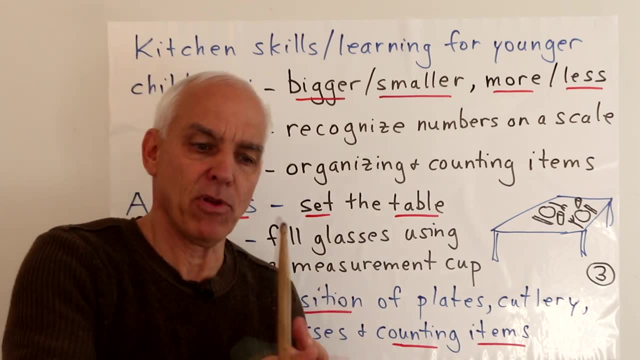 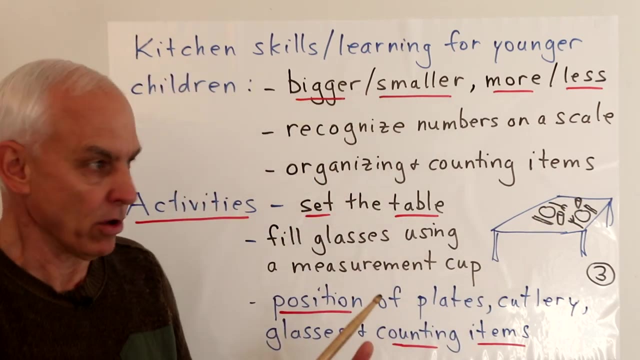 careful context. So let's start with sort of younger children, maybe K, first year, second year. These kinds of children can be introduced to very simple kinds of concepts in the context of the kitchen, For example, notions like bigger and smaller, more or less. These are easily. 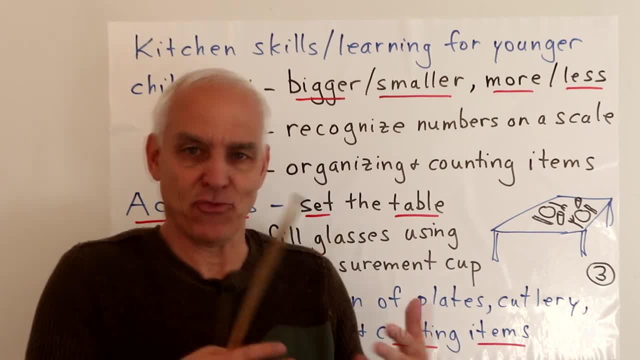 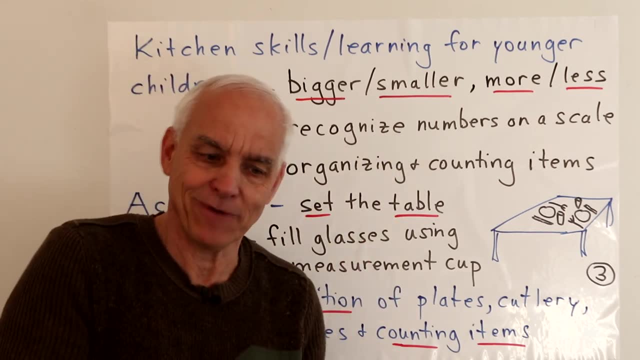 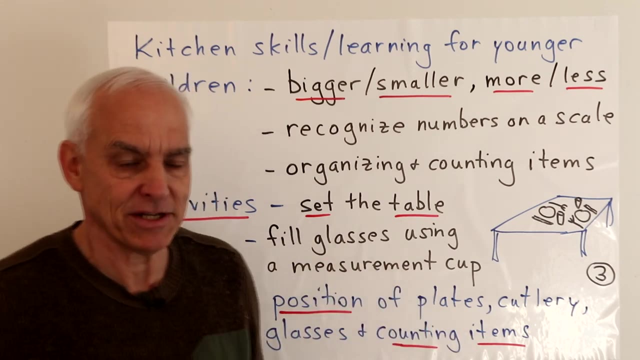 illustrated with the objects, the ingredients of various recipes and so on, that you're manipulating The ability to recognize numbers on a scale. That's something that you can get kids to do: to read scales. how much of this weigh? how many ounces in this container? what's the weight of this item? 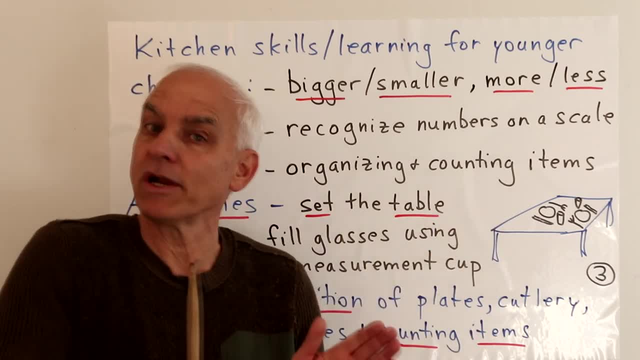 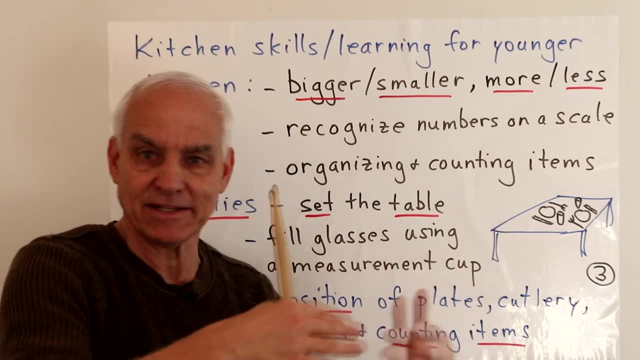 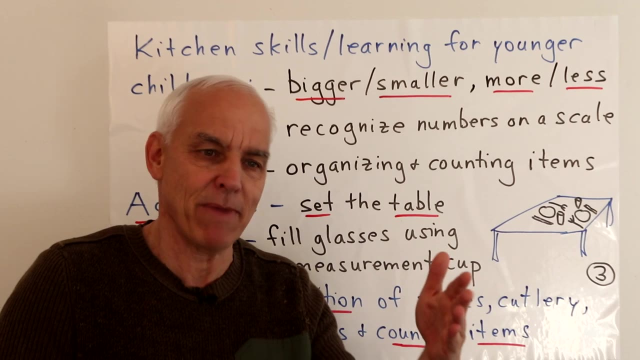 And organizing and counting items, Maybe organizing a pantry. That could be kind of a preliminary activity. Organize your pantry so that similar things are organized the same way, so that there's a kind of a structure, a pattern associated to things. Patterns are important in mathematics and instilling in kids the idea that it's nice. 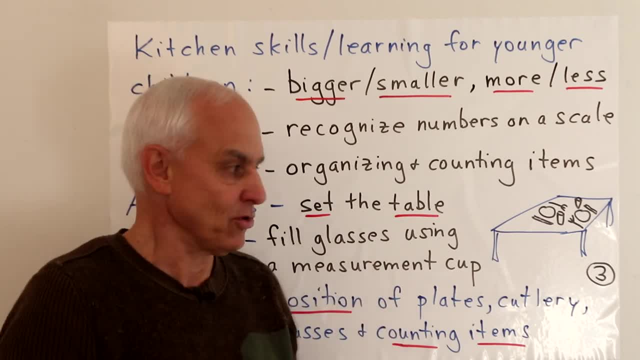 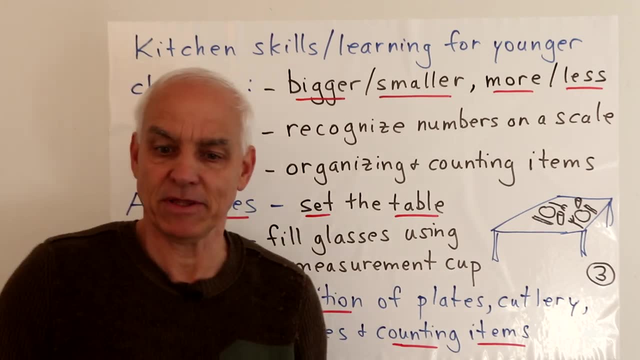 to organize things in a systematic and methodical way. That's a good one In terms of activities. otherwise, I think a nice activity is to set a table. That's something that younger children can naturally do. So there's a table and there's some plates and knives and forks. 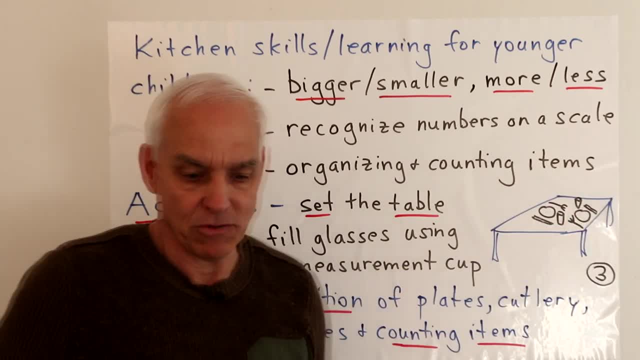 and spoons and maybe some glasses, And so maybe you have a certain number of people. So the child is asked to set the table. So they have to learn the configuration. There's a bit of geometry. Where does the plate go? Where? 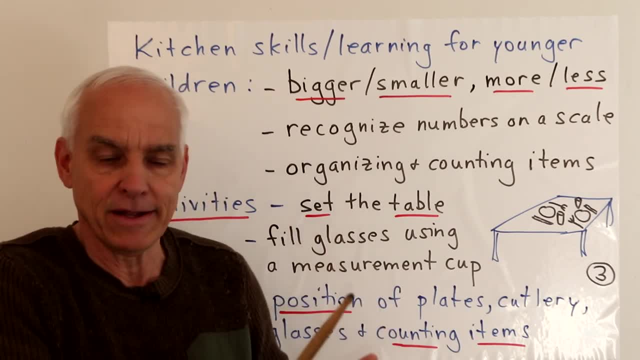 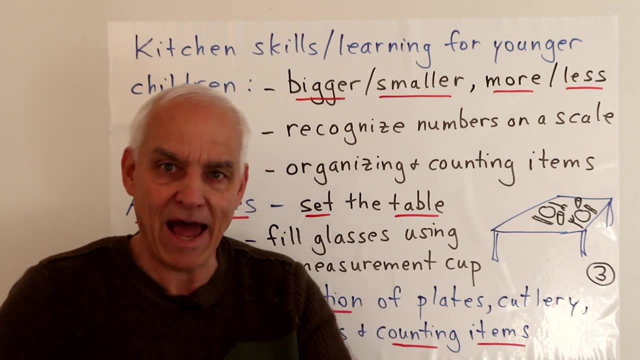 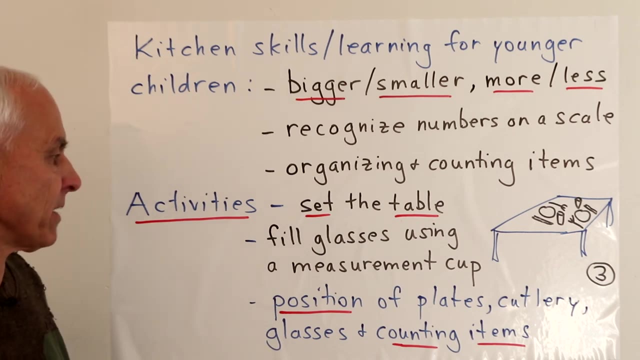 does the knife and fork and spoon go with relation to the plate? Can they then replicate that three or four or five times? whatever it is around the table? Can they put glasses in the right spots? Okay, so they can set the table. That's a mathematical kind of geometrical activity. 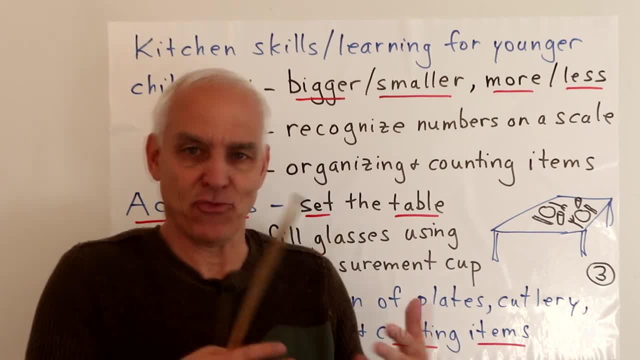 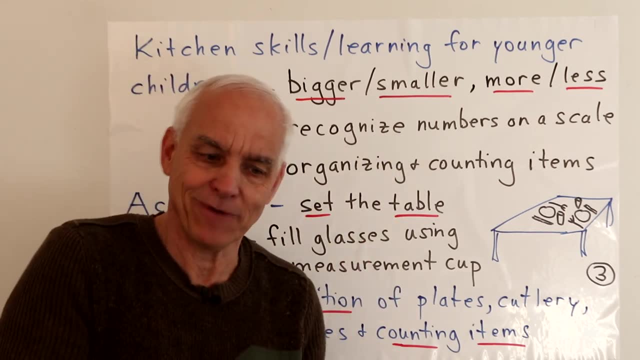 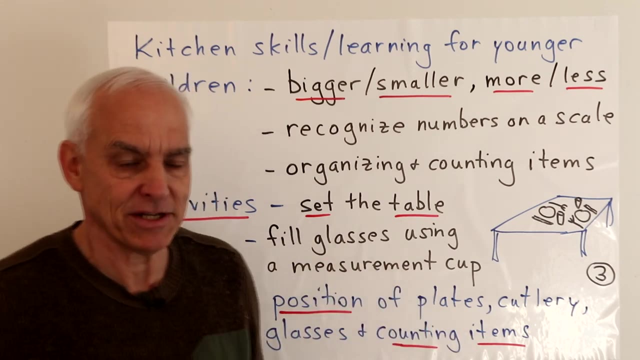 illustrated with the objects, the ingredients of various recipes and so on, that you're manipulating The ability to recognize numbers on a scale. That's something that you can get kids to do: to read scales. how much of this weigh? how many ounces in this container? what's the weight of this item? 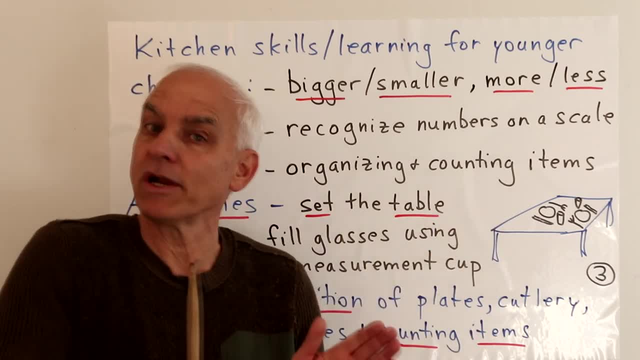 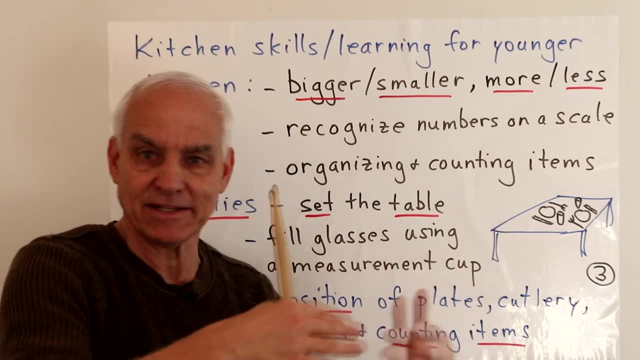 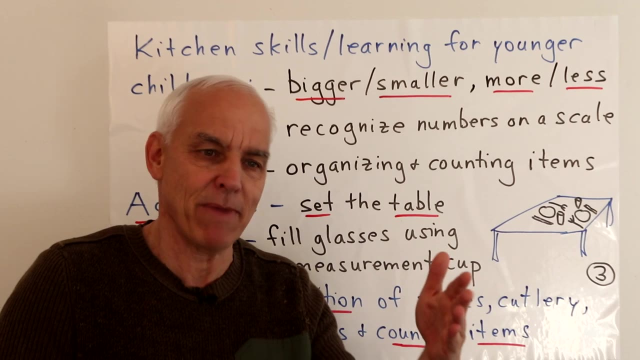 And organizing and counting items, Maybe organizing a pantry. That could be kind of a preliminary activity. Organize your pantry so that similar things are organized the same way, so that there's a kind of a structure, a pattern associated to things. Patterns are important in mathematics and instilling in kids the idea that it's nice. 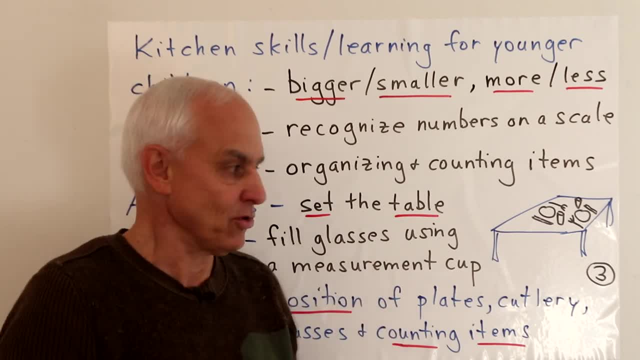 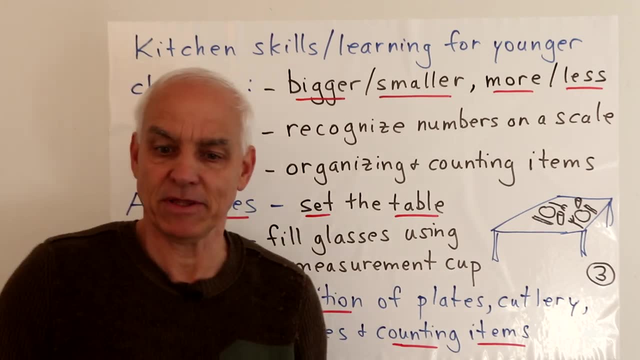 to organize things in a systematic and methodical way. That's a good one In terms of activities. otherwise, I think a nice activity is to set a table. That's something that younger children can naturally do. So there's a table and there's some plates and knives and forks. 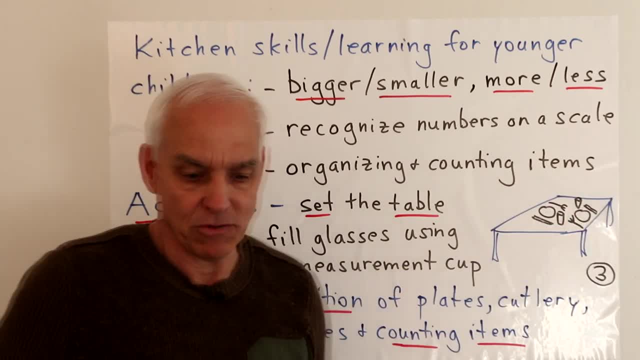 and spoons and maybe some glasses, And so maybe you have a certain number of people. So the child is asked to set the table. So they have to learn the configuration. There's a bit of geometry. Where does the plate go? Where? 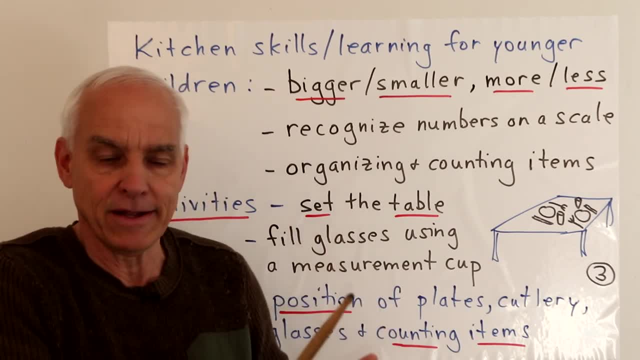 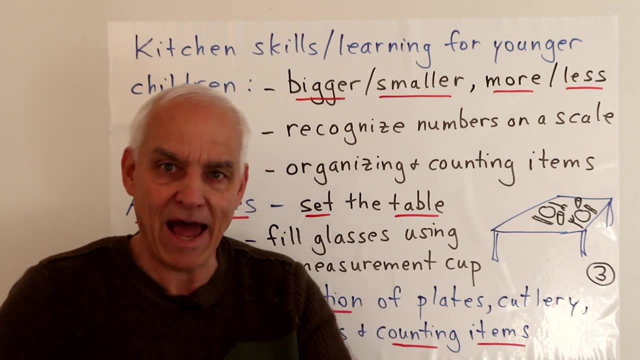 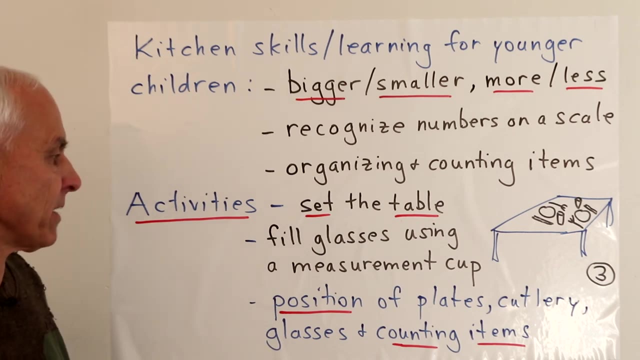 does the knife and fork and spoon go with relation to the plate? Can they then replicate that three or four or five times? whatever it is around the table? Can they put glasses in the right spots? Okay, so they can set the table. That's a mathematical kind of geometrical activity. 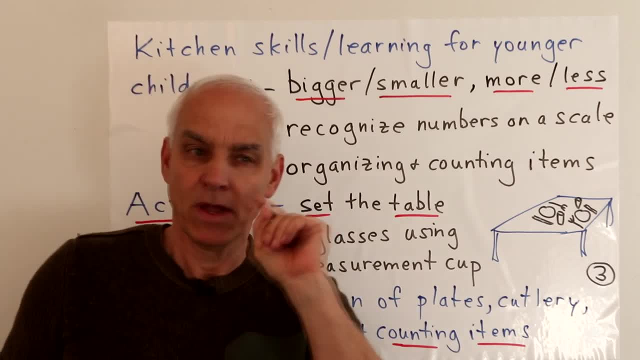 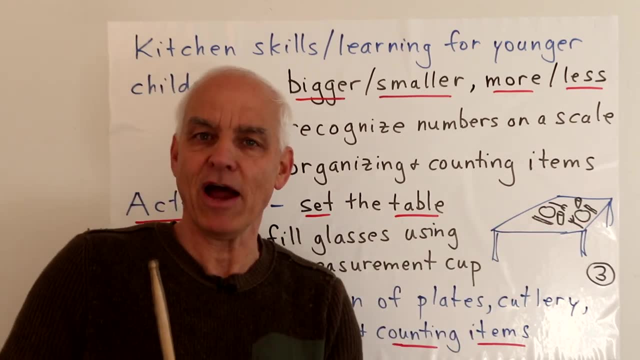 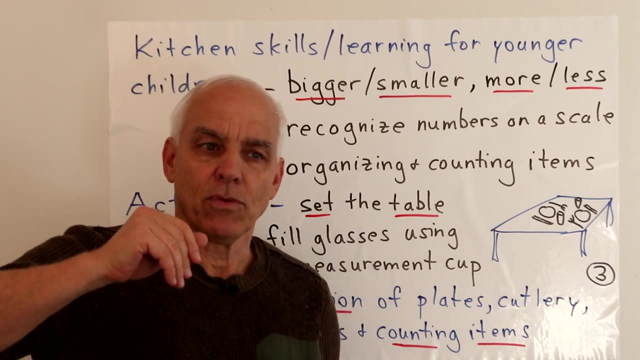 Then maybe we might want to fill the glasses Now. for this it's perhaps interesting to use glasses which are not necessarily all the same size. You have some tall skinny glasses, some shorter, wider ones, and so on, And you could ask the child to try to fill all the glasses with. 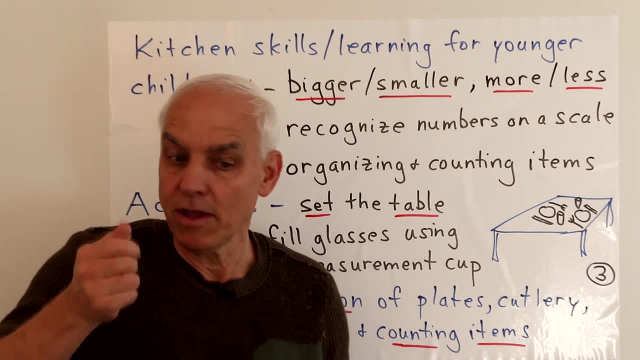 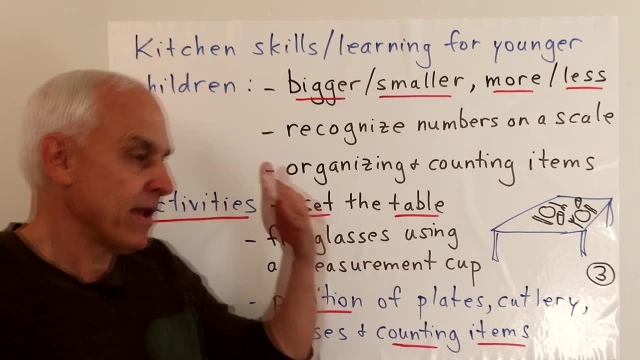 the same amount of water, maybe one cup of water, So they could use a measuring cup for that. Okay, so one cup of water in each of the glasses, And then they get the appreciation that, even though the glasses may have different sizes, you know, they can still put. 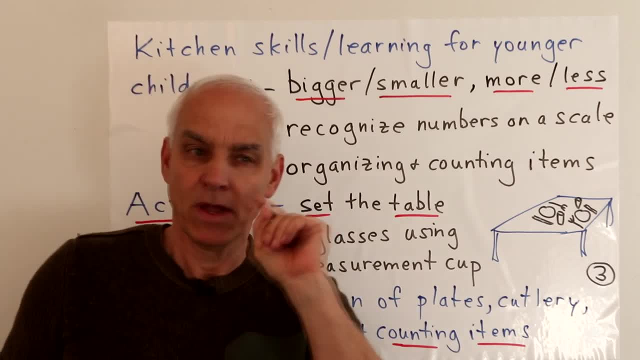 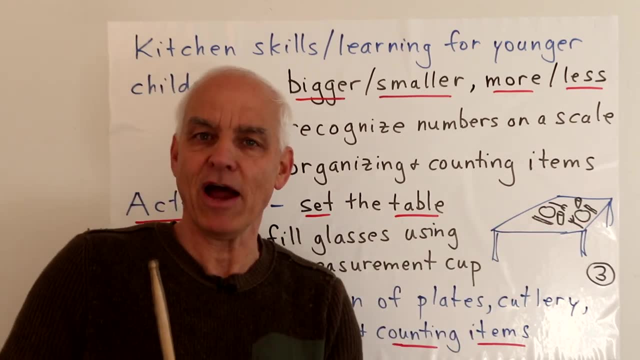 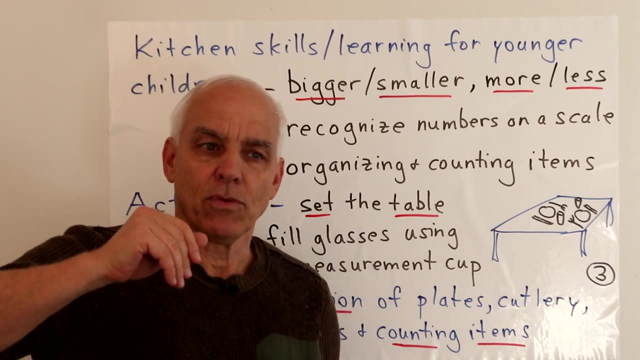 Then maybe we might want to fill the glasses Now. for this it's perhaps interesting to use glasses which are not necessarily all the same size. You have some tall skinny glasses, some shorter, wider ones, and so on, And you could ask the child to try to fill all the glasses with. 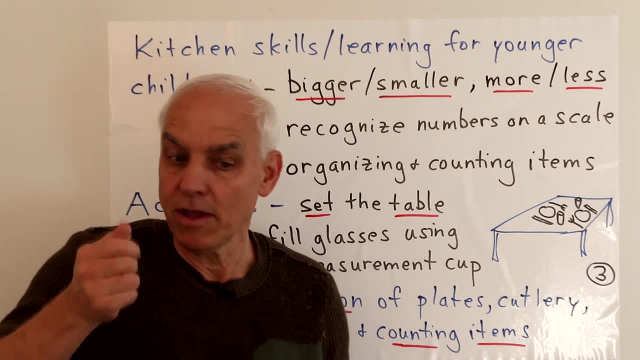 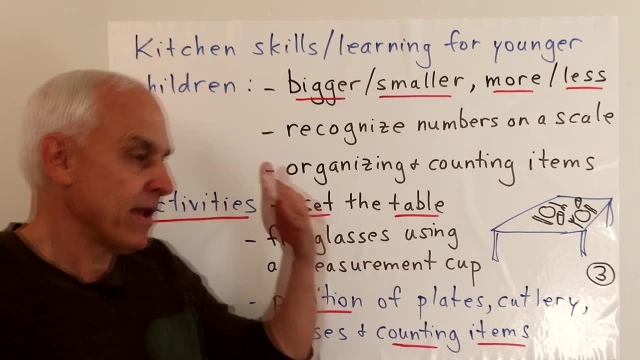 the same amount of water, maybe one cup of water, So they could use a measuring cup for that. Okay, so one cup of water in each of the glasses, And then they get the appreciation that, even though the glasses may have different sizes, you know, they can still put. 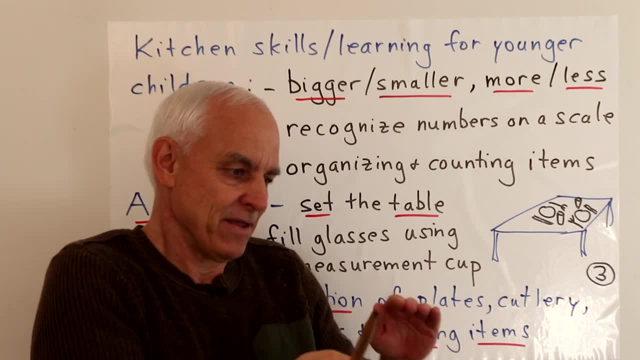 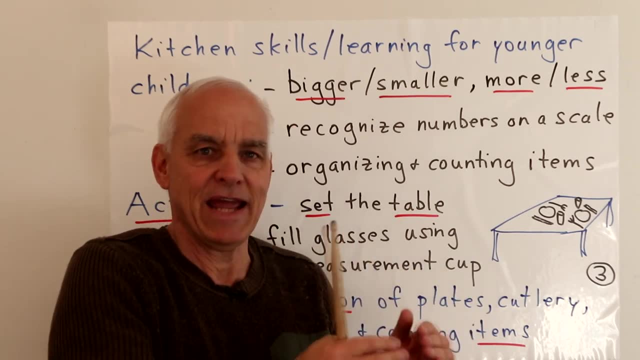 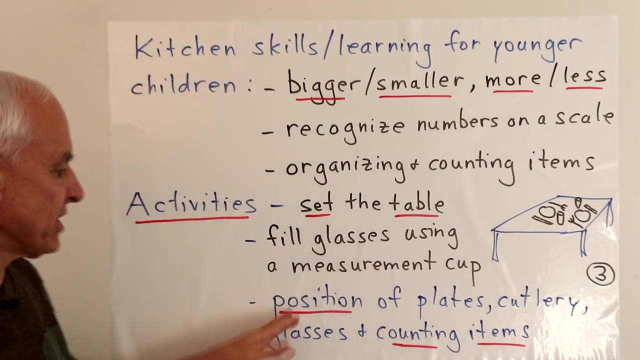 the same amount of water in these various glasses and the actual amount look is different. So they get a sense that you know the shape of the container affects how much water appears in it. Okay, and then the position of the plates, cutlery glasses and counting items. You can. 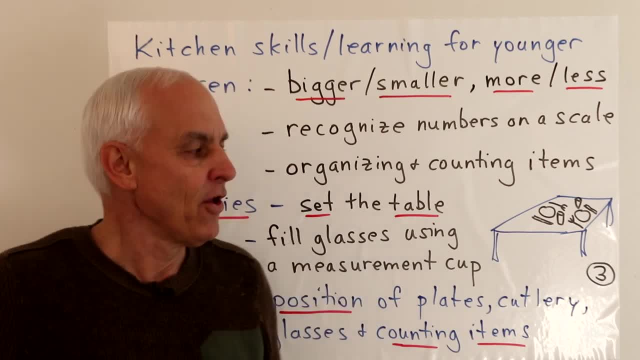 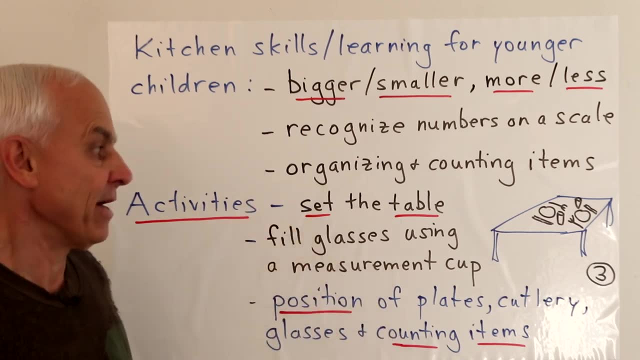 ask them: how many objects are there all together on the table, that kind of thing. So there's some sort of simple arithmetical and geometrical aspects Involved in sort of setting up even the table. So these are simple things that even young children 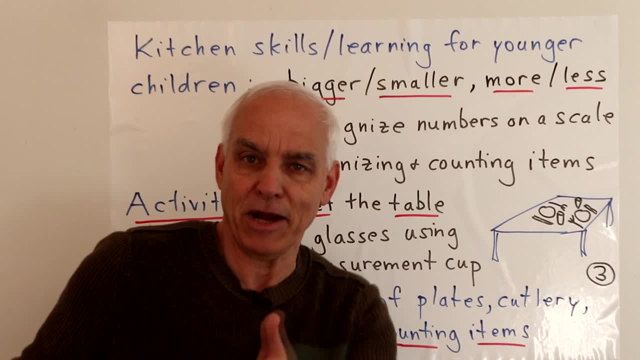 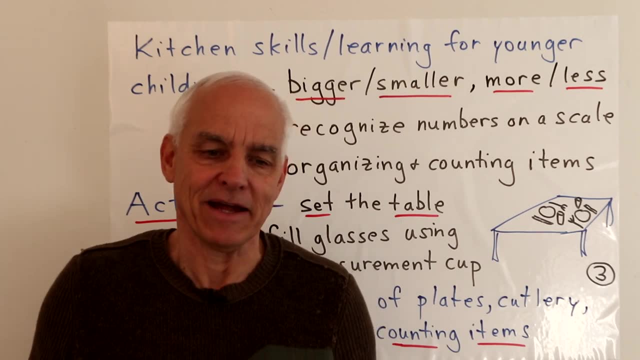 can help you with, And so if you introduce a mathematical or arithmetical aspect to it, then you can be encouraging the children numerically at the same time as actually doing something functionally useful Now, when motivating children to help you cook, 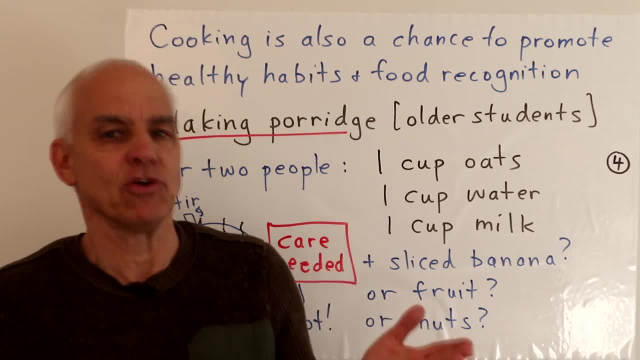 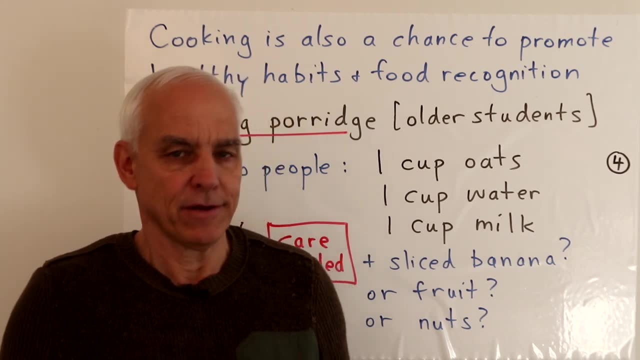 I think a lot of examples tend to steer towards things which are sweet and enticing for young People, usually containing lots of sugar, And although that's well and good, in small quantities, it's also good to think about the time in the kitchen as an opportunity of teaching children. 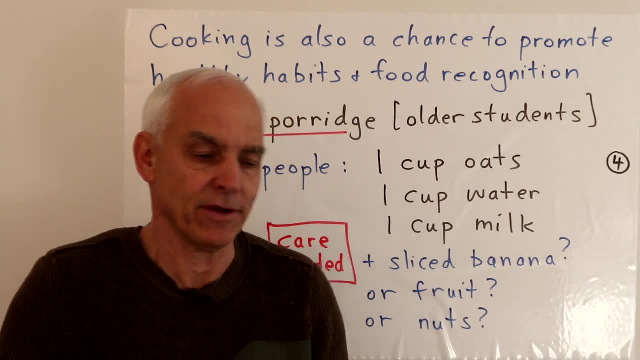 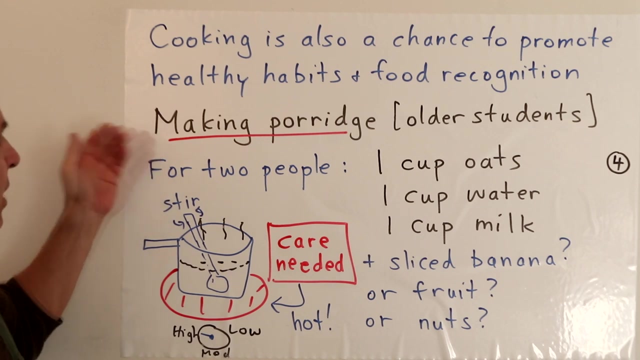 about healthy eating habits and sort of good foods, and you know healthy foods. So that's maybe something else that we can think about. So I'm going to use at least a few examples which are sort of healthy kind of examples, So we will have a cake to end the story. Okay, so an activity that's quite good is making porridge. 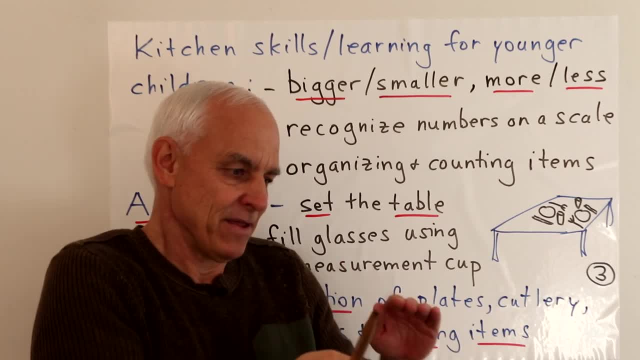 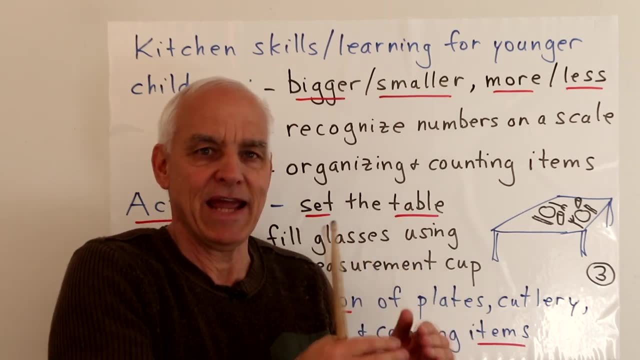 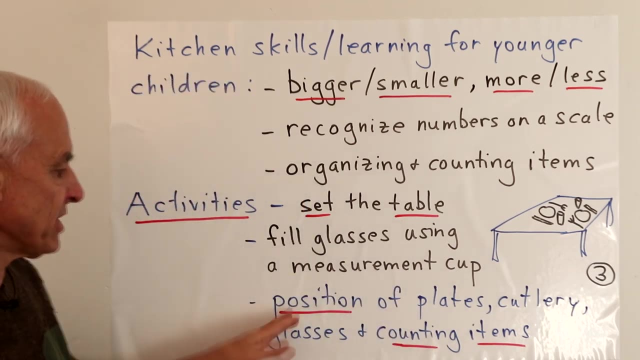 the same amount of water in these various glasses And the actual amount look is different. So they get a sense that you know the shape of the container affects how much water appears in it. Okay, and then the position of the plates, cutlery glasses and counting items. You 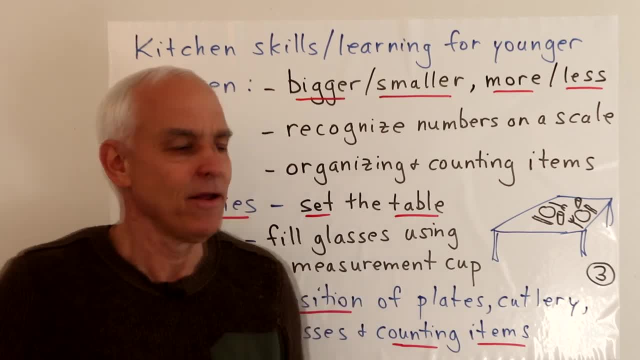 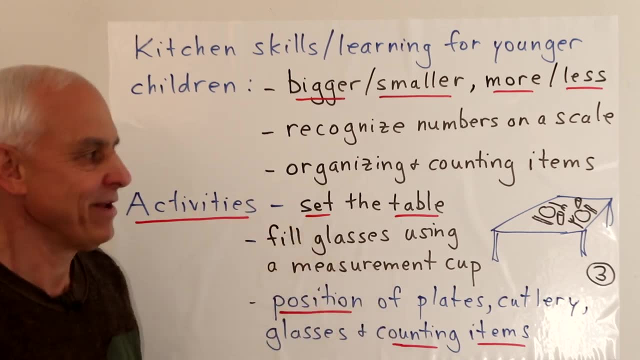 can ask them: how many objects are there all together on the table, that kind of thing. So there's some sort of simple arithmetical and geometrical aspects And so you can be involved in sort of setting up even the table. So these are simple things that 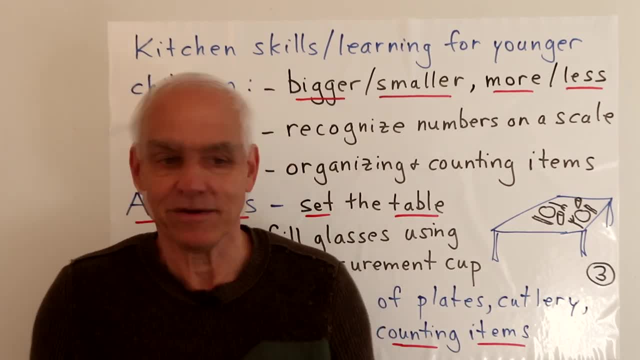 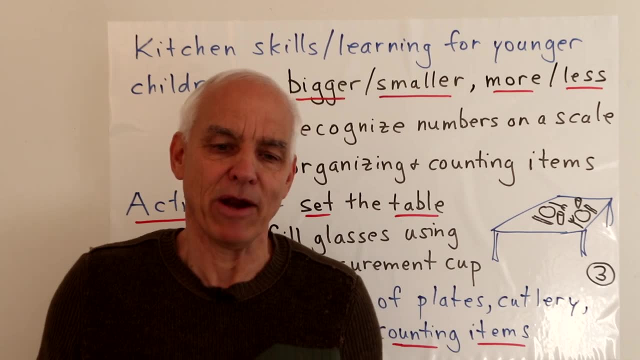 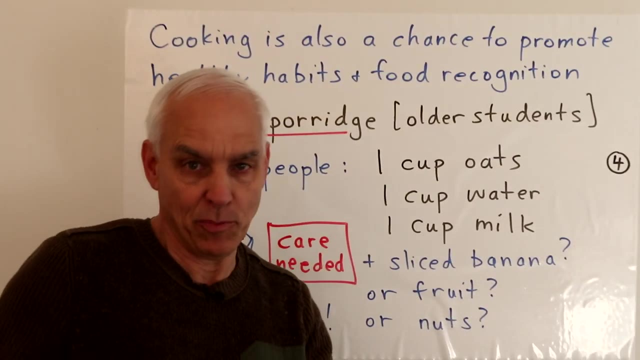 even young children can help you with, And so if you introduce a mathematical or arithmetical aspect to it, then you can be encouraging the children numerically at the same time as actually doing something functionally useful. Now, when motivating children to help you cook, I think a 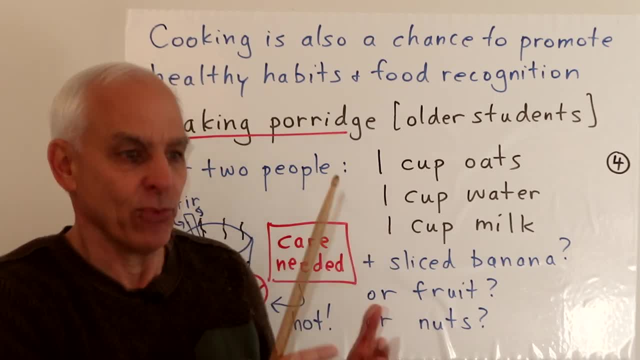 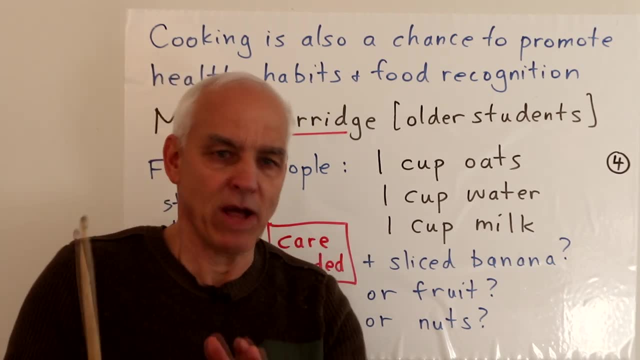 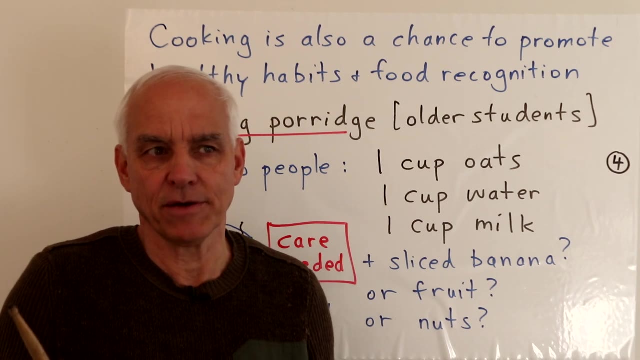 lot of examples tend to steer towards things which are sweet and enticing for young people, Usually containing lots of sugar, And although that's well and good in small quantities, it's also good to think about the time in the kitchen as an opportunity of teaching children. 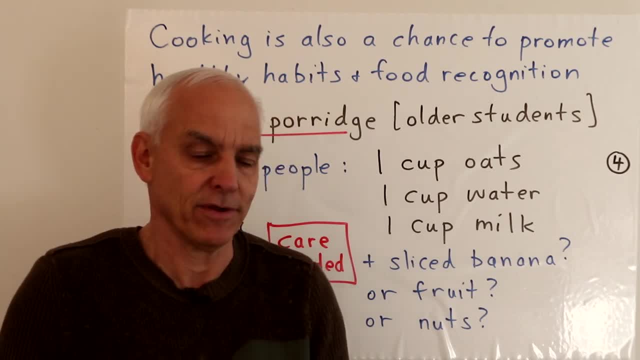 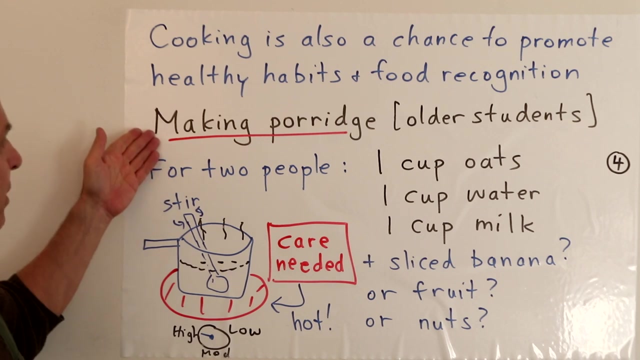 about healthy eating habits and sort of good foods, and you know healthy foods, So that's maybe something else that we can think about. So I'm going to use at least a few examples which are sort of healthy kind of examples. will have a cake to end the story, okay. so an activity that's, uh, quite good is making porridge. 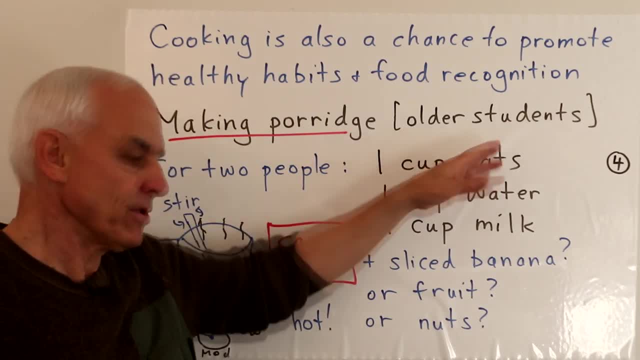 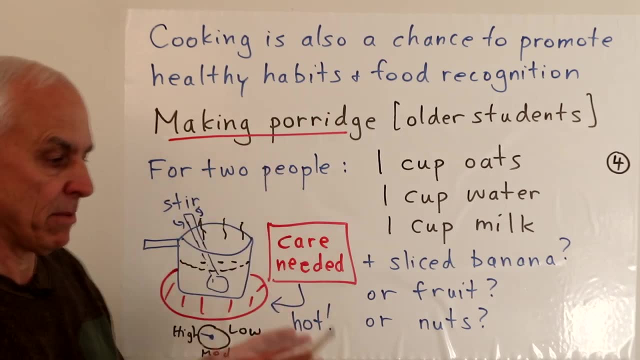 it's relatively simple, but older students can- can actually physically attempt this. it's not too hard, and so, basically, what you need is a recipe. so maybe you have oats, and perhaps for two people one cup of oats suffices, especially if they're young people, and maybe the recipes you combine. 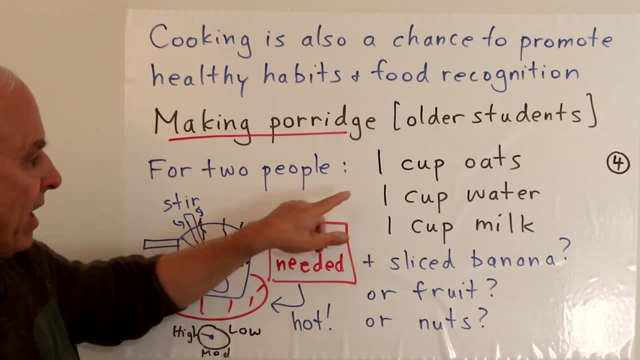 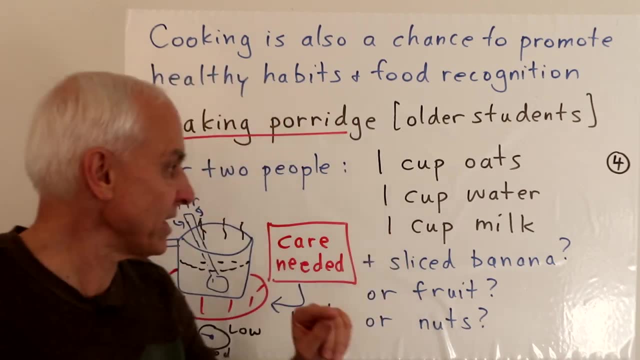 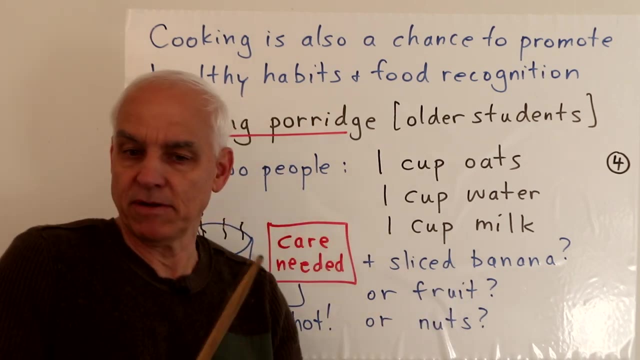 one cup of oats in a pot, along with one cup of water and one cup of milk. that's the recipe that i happen to use and it seems to work okay. okay, so that's very simple: one cup oats, one cup water, one cup milk, and then maybe you can add some further things, maybe slice a banana or put in. 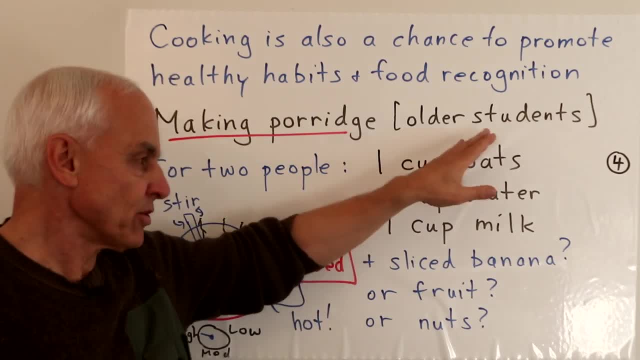 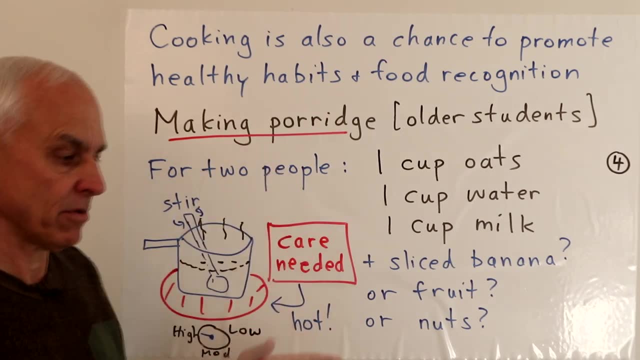 It's relatively simple, but older students can actually physically attempt this. It's not too hard, And so, basically, what you need is a recipe. So maybe you have oats, and perhaps for two people a one cup of oats suffices, especially if they're young people, And maybe the recipes you combine 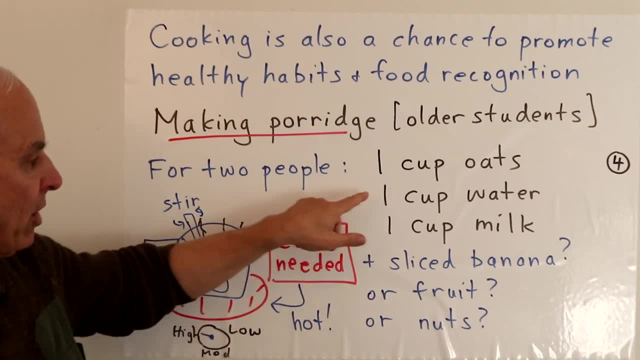 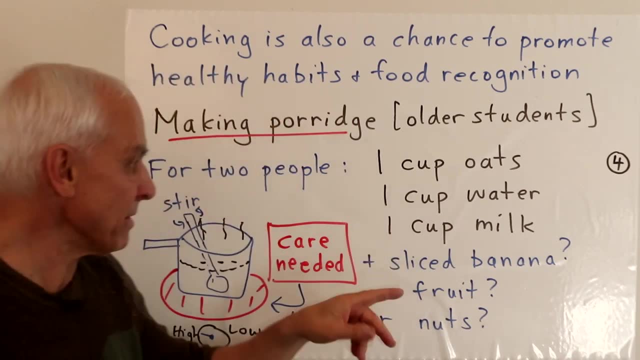 one cup of oats in a pot, along with one cup of water and one cup of milk. That's the recipe that I happen to use And it seems to work Okay, Okay. So that's very simple: One cup oats, one cup water, one cup milk. 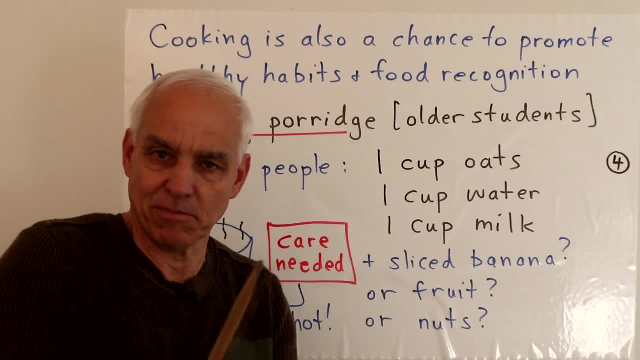 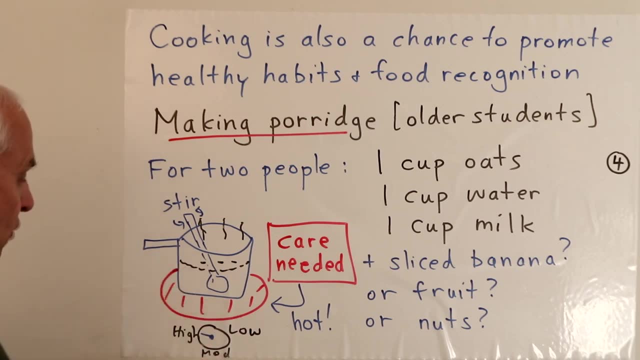 And then maybe you can add some further things, maybe slice a banana or put in some fruit, or maybe a sprinkle of nuts or something like that. So you're going to put that in pan on the stove and then you're going to turn up the um, the temperature. Okay, 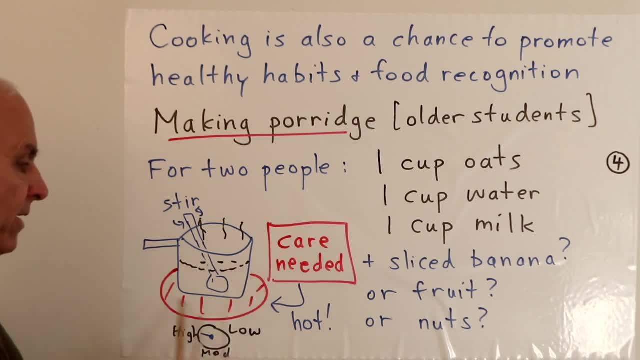 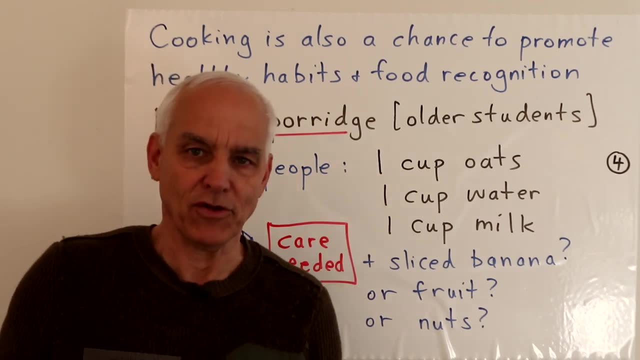 So this is a situation where care is needed because we are involving a hot plate and there's a stir, So the porridge typically has to be stirred while it's not cooking, All right. So if we have that basic recipe for porridge down, you can ask the child. okay, what happens if we're trying to cook. 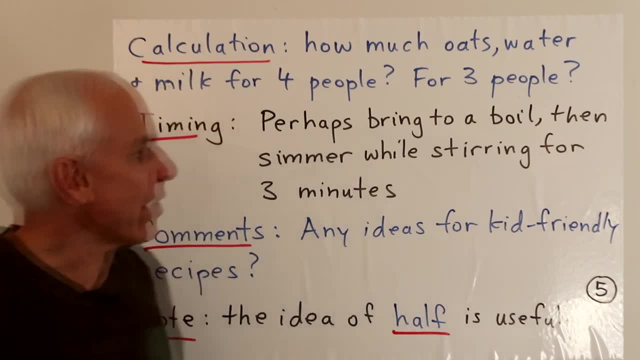 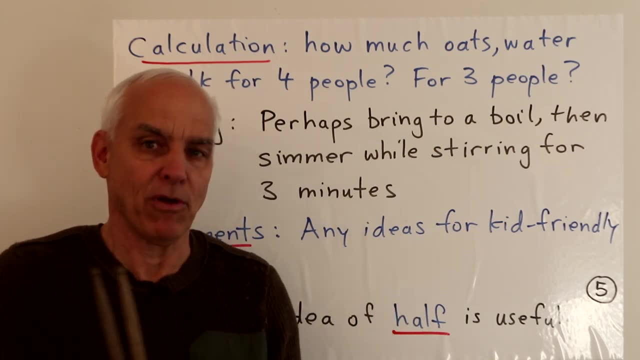 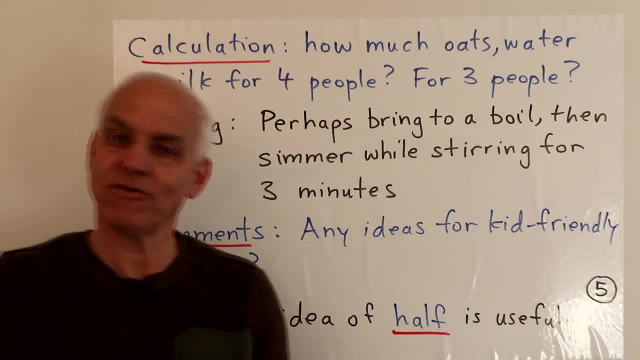 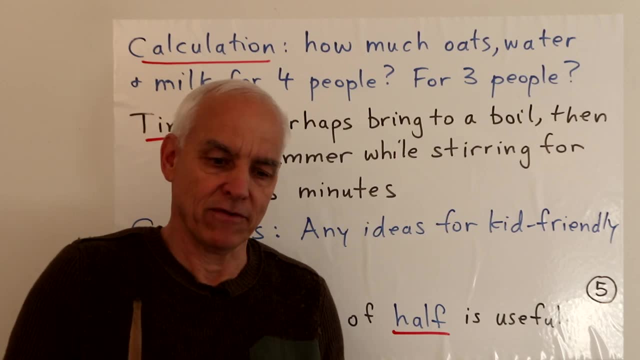 two cups water and two cups of milk and two cups of oats. but that makes sense. so we're proportionally multiplying everything by two to account for the fact that there's twice as many people. a more subtle question is: what do we do when we're cooking for three people? 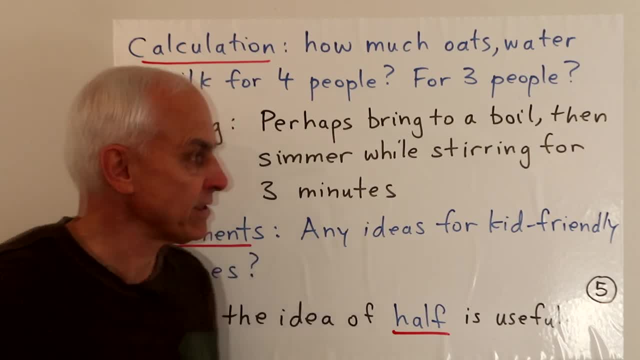 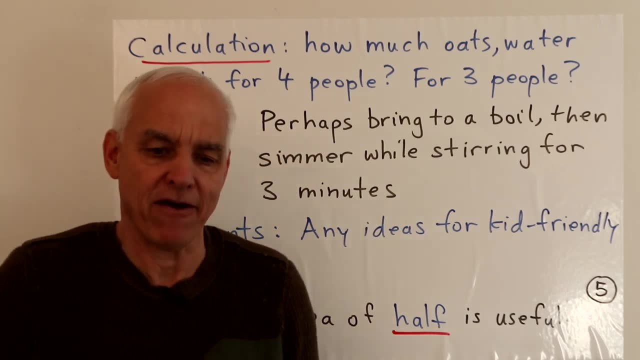 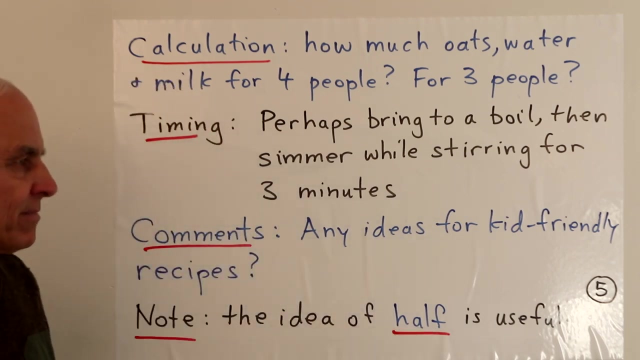 sort of between the two people case and the four person case, and so that's maybe a little bit more involved. it actually, uh really lends itself to talking a little bit about a half. you're gonna have to talk about one and a half cups of oats and so on, so that's, that's a good place to uh to. 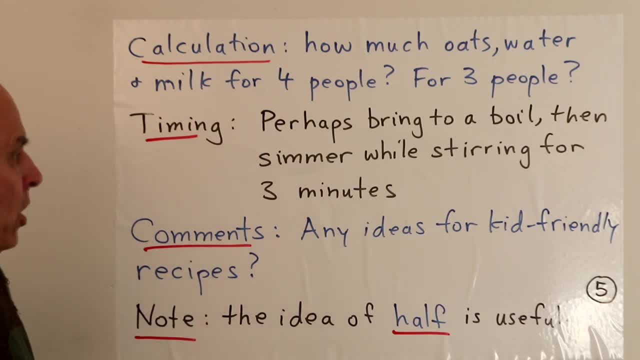 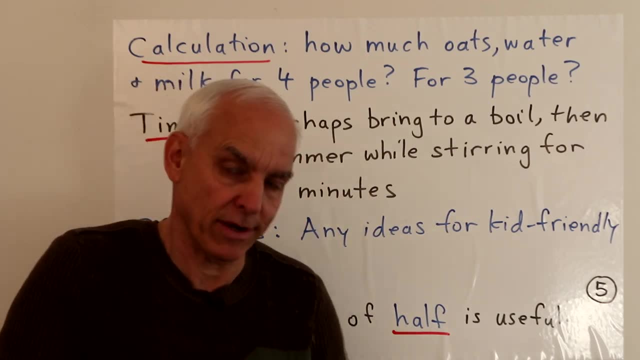 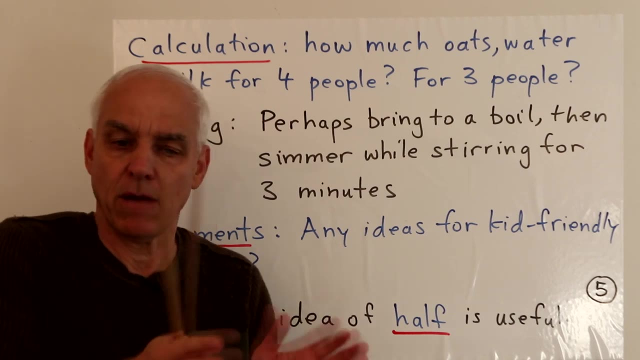 see the usefulness of that concept of a half. okay, what about timing? so when we're cooking the porridge we have to have a sense of how long are we going to cook it and sort of what, what temperature. so maybe one strategy is to perhaps first bring the combination to a boil, stirring it. 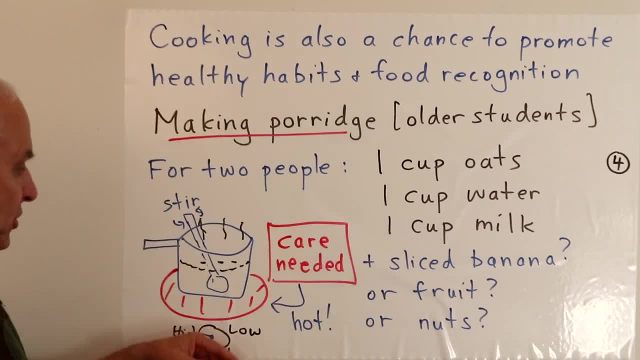 some fruit, or maybe a sprinkle of nuts or something like that. so you're going to put that in the pan on the stove and then you're going to turn up the the temperature, okay. so this is a situation where care is needed, because we are involving a hot plate and there's a 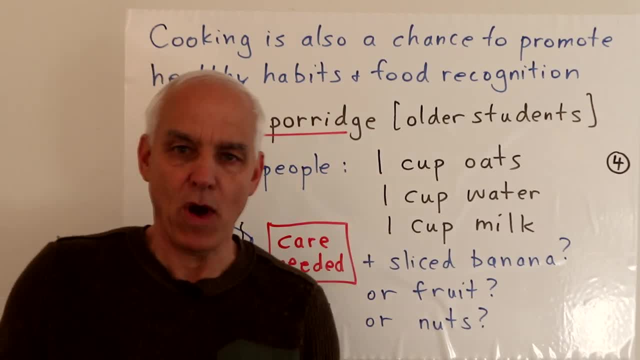 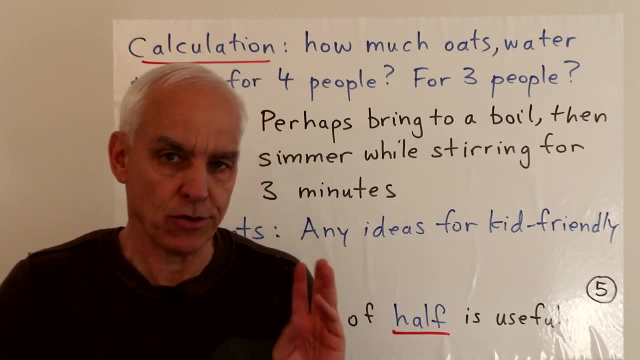 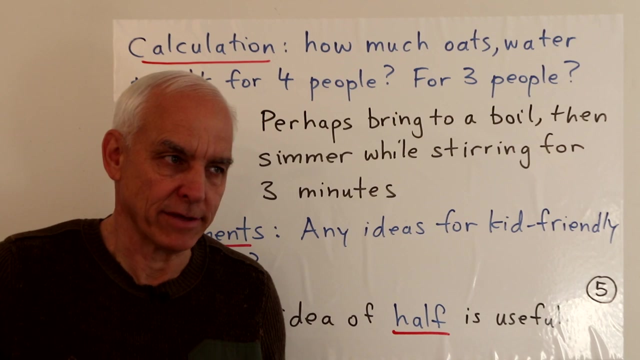 stir. so the porridge typically has to be stirred while it's not cooking. all right. so if we have that basic recipe for porridge down, you can ask the child. okay, what happens if we're trying to cook for four people instead of for two? okay, so the child hopefully will be able to figure out that. 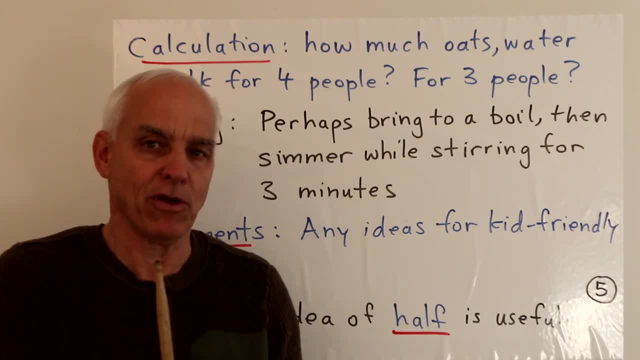 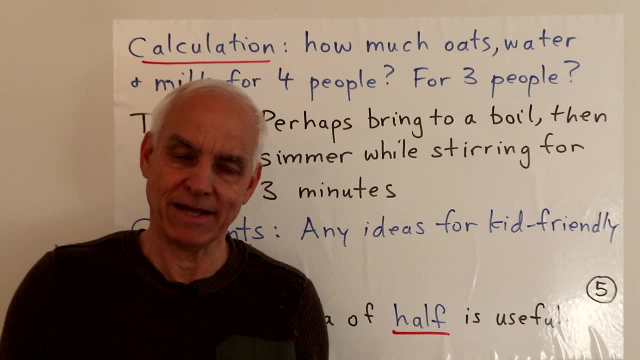 because four is twice two. we should double all the ingredients, so we should have two cups of water and two cups of milk and two cups of oats. but that makes sense. so we're proportionally multiplying everything by two to account for the fact there's twice as many people. a more subtle question is: what do we do when we're cooking for three people? 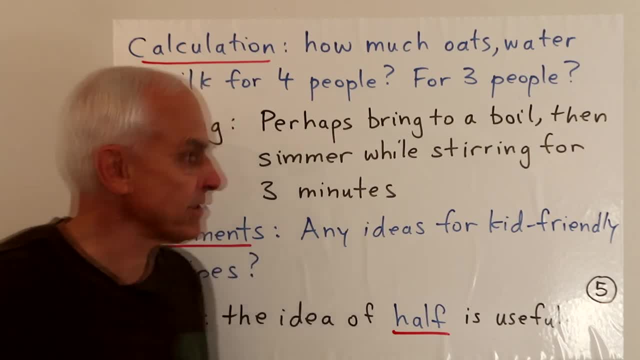 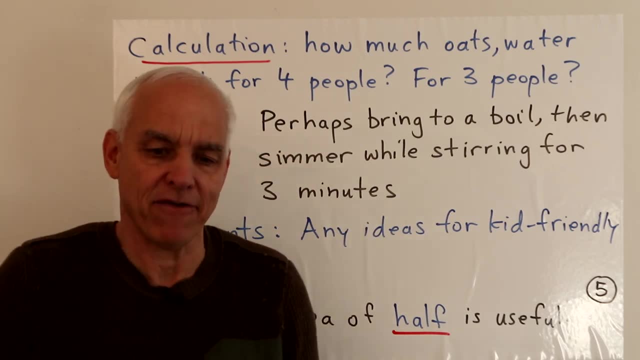 sort of between the two people case and the four person case, and so that's maybe a little bit more involved. it actually, uh, really lends itself to talking a little bit about a half. you're gonna have to talk about one and a half cups of oats and so on, so that's. 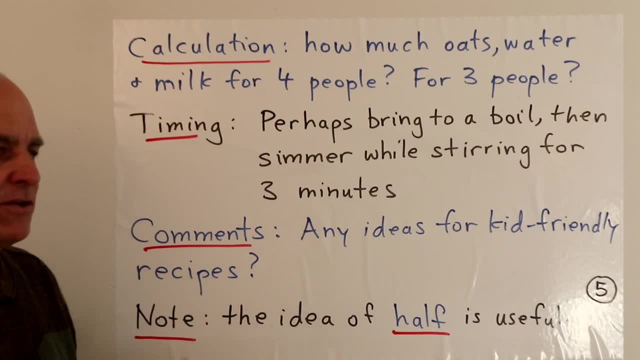 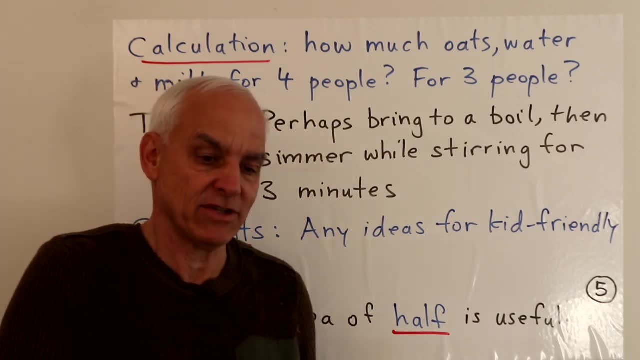 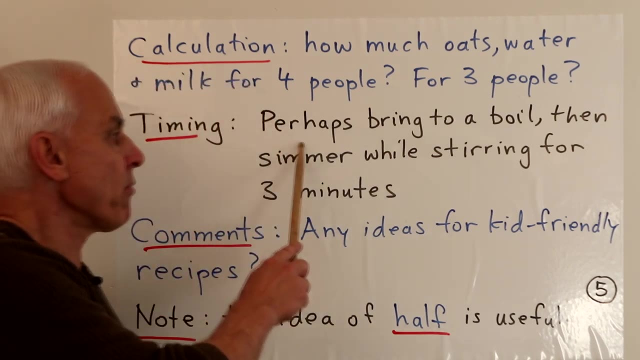 that's a good place to uh to see the usefulness of that concept of a half. okay, what about timing? so when we're cooking the porridge we have to have a sense of how long are we going to cook it and sort of what temperature. so maybe one strategy is to perhaps first bring 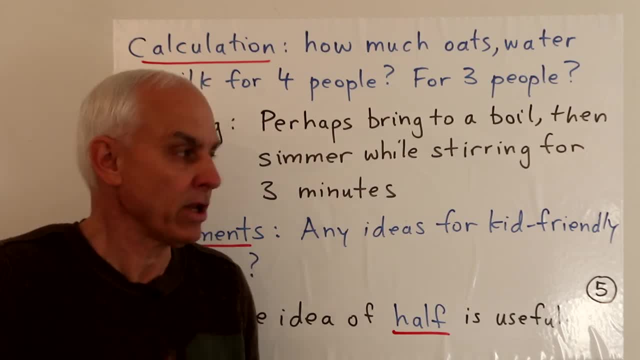 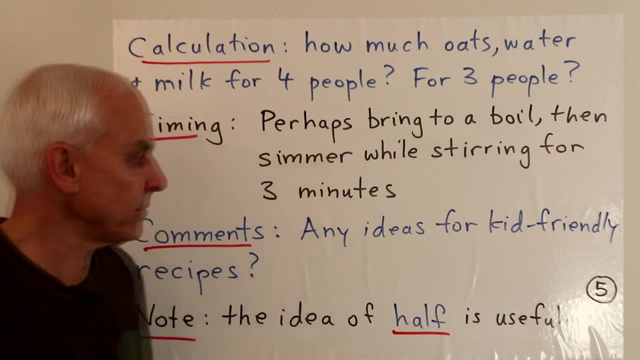 the combination to a boil, stirring it. then we have it boiling and then we can turn it down and simmer it while stirring for another three minutes or something like that. okay, so then we get some porridge and that's great. that's a relatively simple thing, but 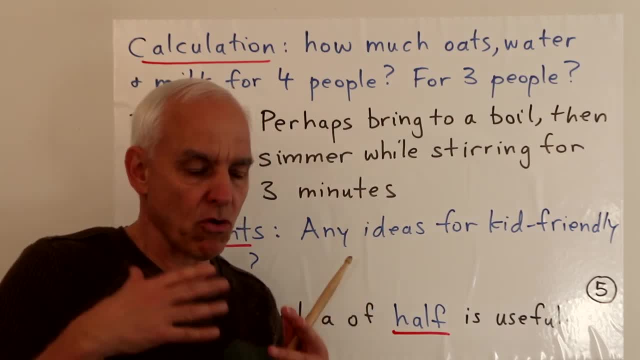 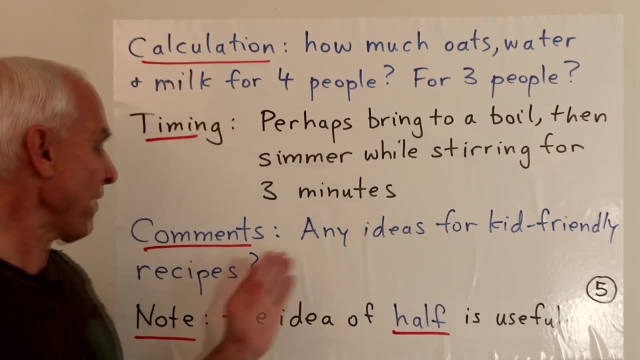 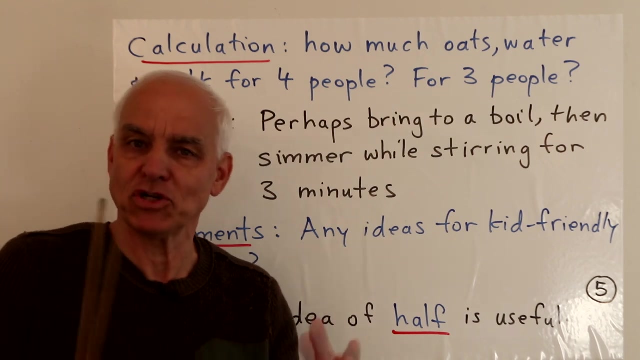 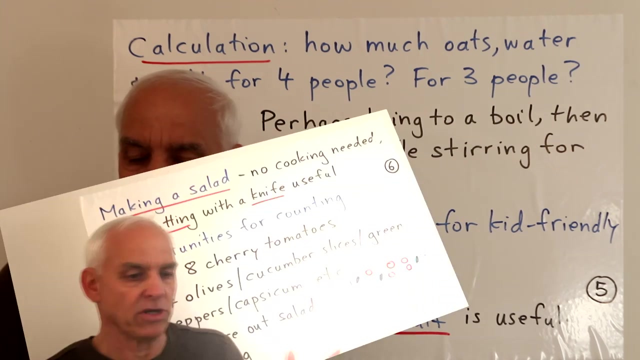 there has been an aspect of arithmetic or proportion or quantity involved there. comments please: do you have any ideas for sort of kid friendly recipes or things that you can easily cook or bake that you might want to share with us? so in the comments please give us your ideas and maybe experiences. all right, so you've had your yummy porridge for. 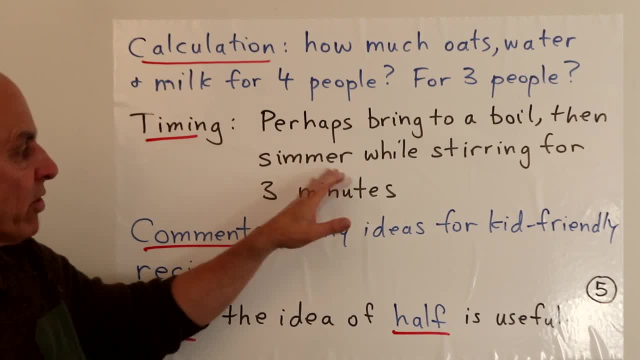 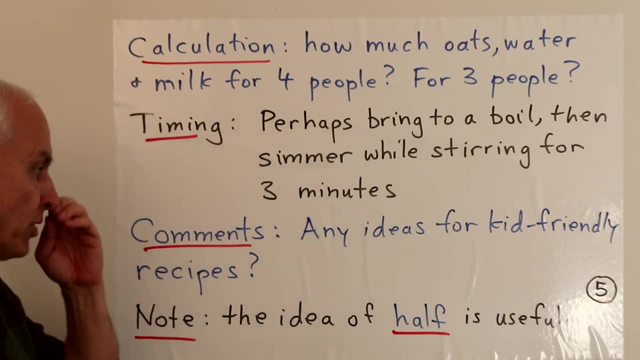 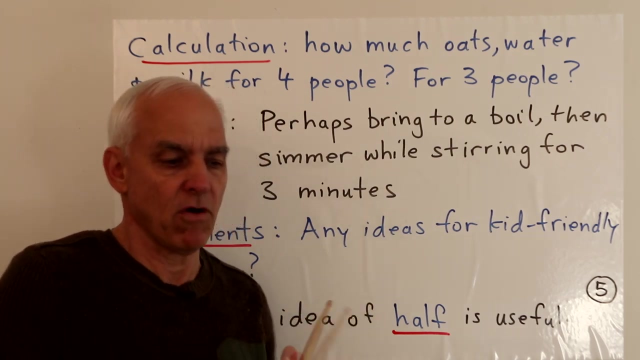 then we have it boiling and then we can turn it down and simmer it while stirring for another three minutes or something like that. okay, so then we get some porridge and that's great. that's a relatively simple thing, but there has been an aspect of arithmetic or proportion or quantity involved there. 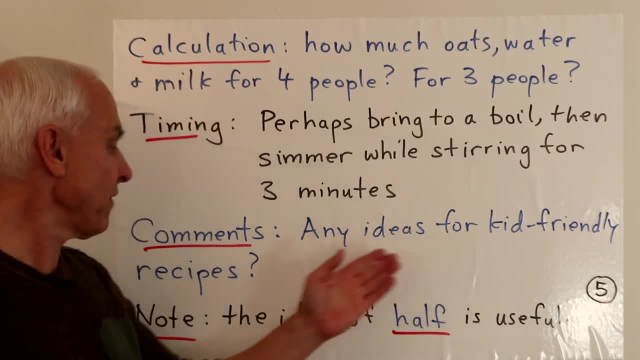 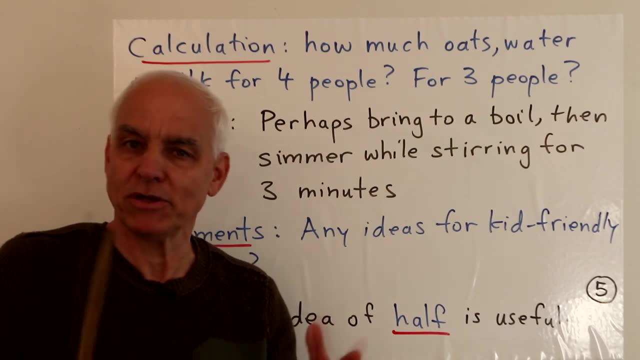 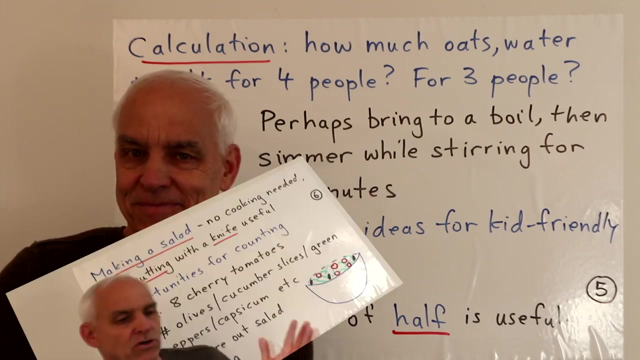 comments please do you have any ideas for sort of kid friendly recipes or things that you can easily cook or bake that you might want to share with us? so in the comments please give us your ideas and maybe experiences. all right, so you've had your yummy porridge for breakfast. 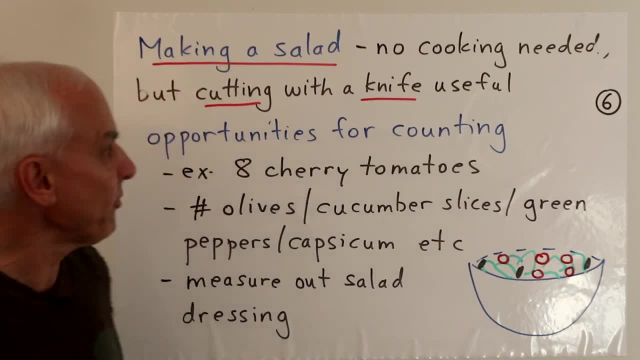 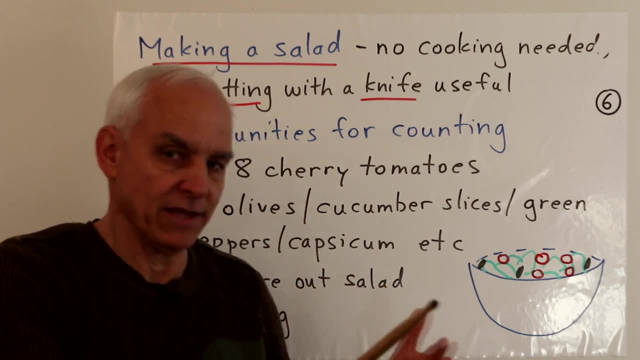 and then a few hours later, it's time for lunch, so perhaps we could make a salad. that's an activity that doesn't involve any cooking, so we don't need the stove or the oven, but some cutting with a knife is useful, and so we have to be careful about, you know, safety with. 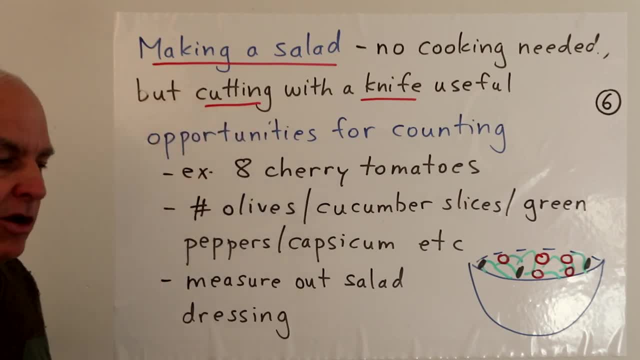 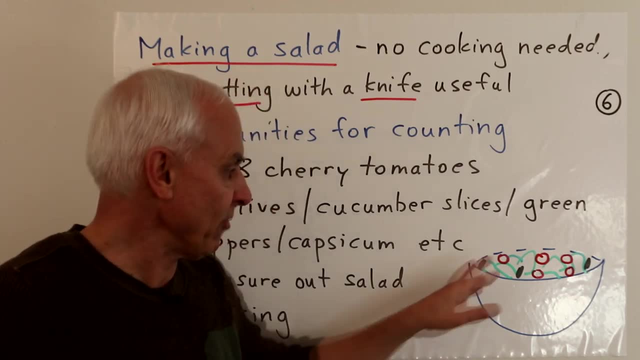 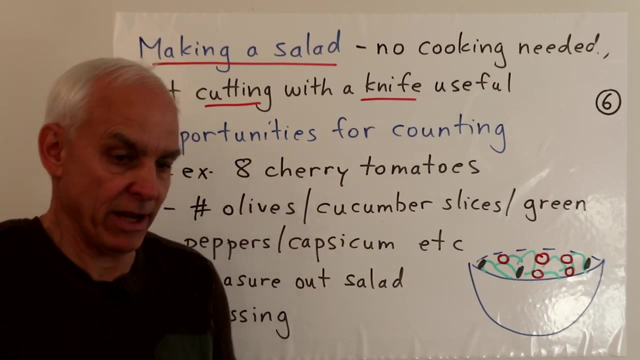 knives so. but there's opportunities for counting here. we're going to put a certain amount of ingredients into our salad, a wide range of possibilities: some lettuce, some greens, and maybe various other things. perhaps you might have eight cherry tomatoes. so i say, okay, we need eight cherry tomatoes, you know. so the your child can can get out those eight tomatoes maybe. 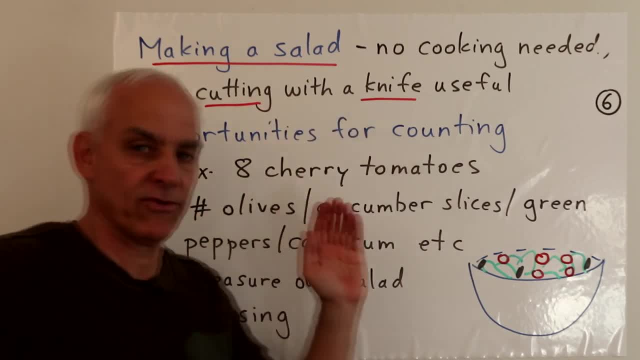 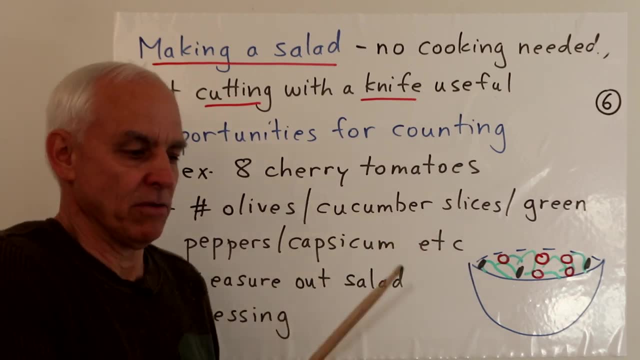 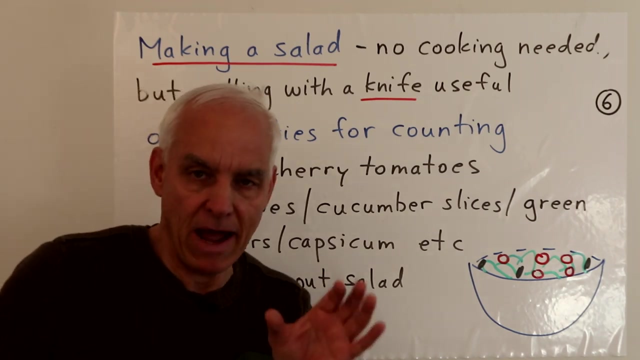 a certain number of olives or cucumber slices or green peppers called capsicum in australia. so you know there's. there's a counting aspect in making a salad. perhaps you can make it kind of fun, and then finally we might measure out some salad dressing. you know, maybe a certain amount, maybe a. 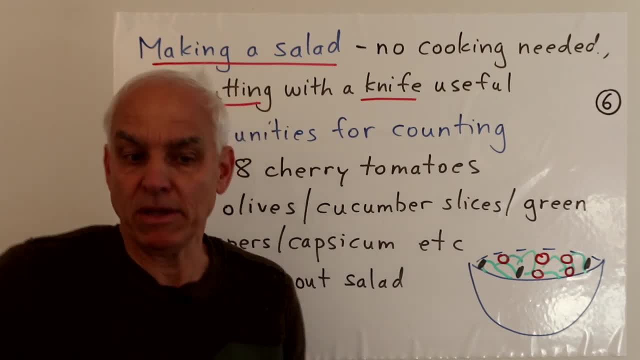 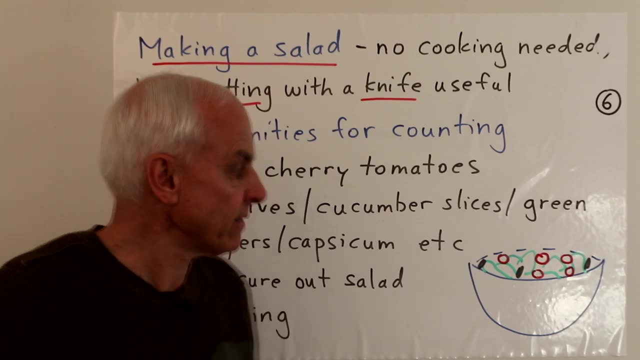 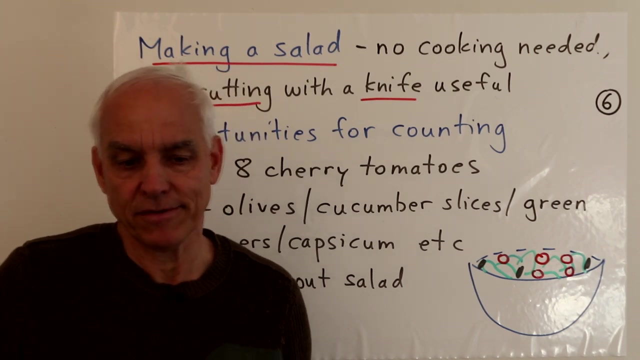 tablespoon of salad dressing, or maybe even some, some small volume of, uh, salad dressing. if you have a small, you know, a quarter cup or something like that, and then you have a salad and then you can divvy it up amongst the people at the table, and their child has contributed a. 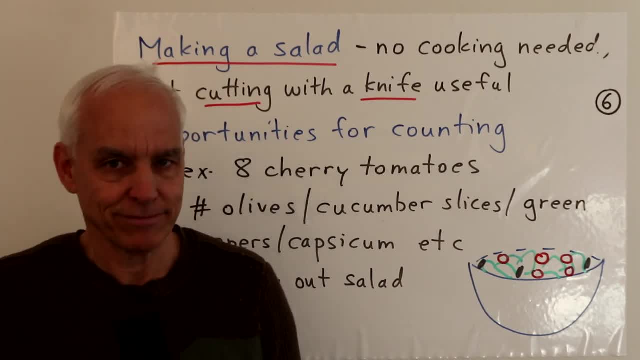 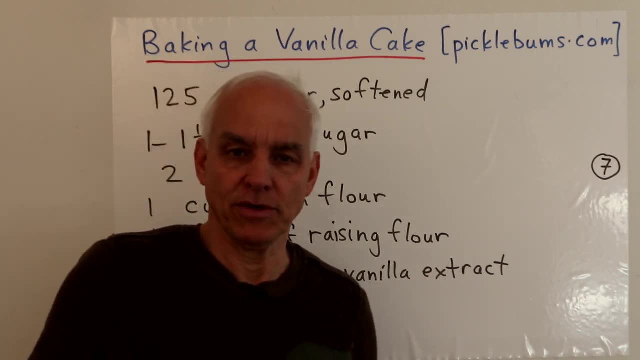 little bit of arithmetic into making a healthy lunch. okay, so great, we've done some breading, we're stuff some lunch stuff and then at some point we might want an afternoon snack and let's bake a cake. okay, traditional, great thing for kids to do because there's an obvious enticing outcome for it. so I've taken of the many possible. 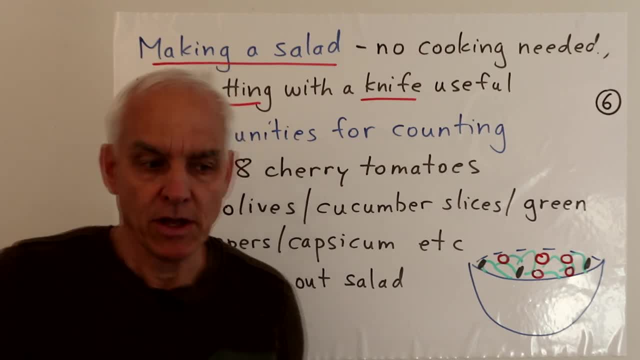 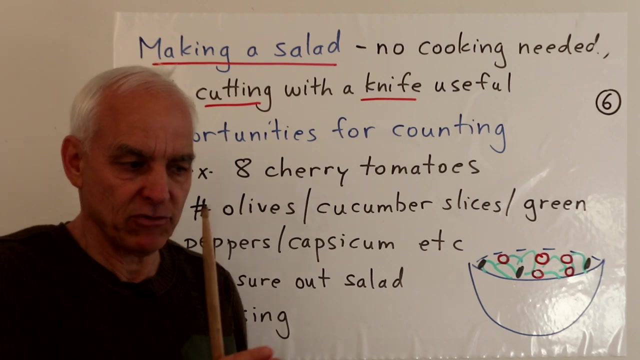 breakfast, and then a few hours later it's time for lunch, so perhaps we could make a salad. that's an activity that doesn't involve any cooking, so we don't need the stove or the oven, but some cutting with a knife is useful, and so we have to be careful about, you know, safety with. 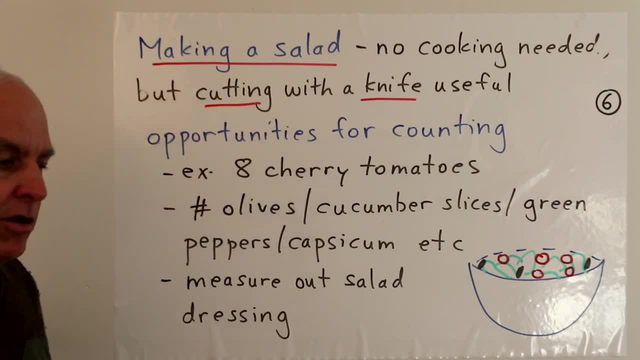 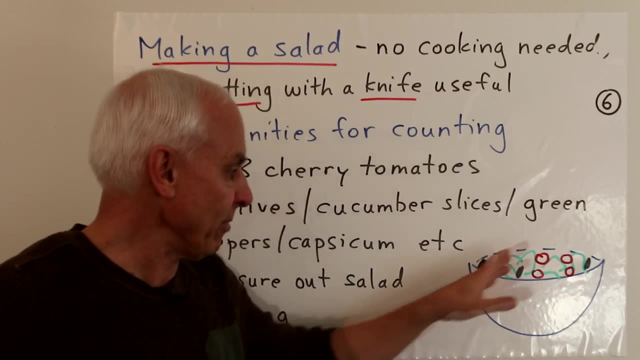 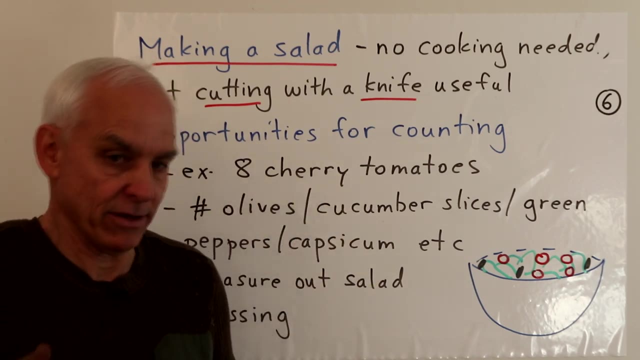 knives, so. but there's opportunities for counting here. we're going to put a certain amount of ingredients into our salad, of course. wide range of possibilities: some lettuce, some greens, and maybe various other things. perhaps you might have eight cherry tomatoes. so i say, okay, we need eight cherry tomatoes, you know. so the your child can can get out those eight. 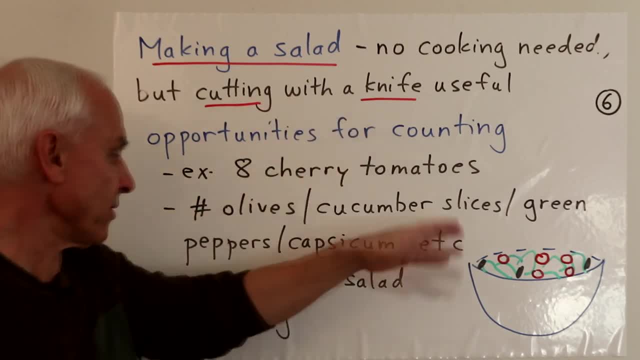 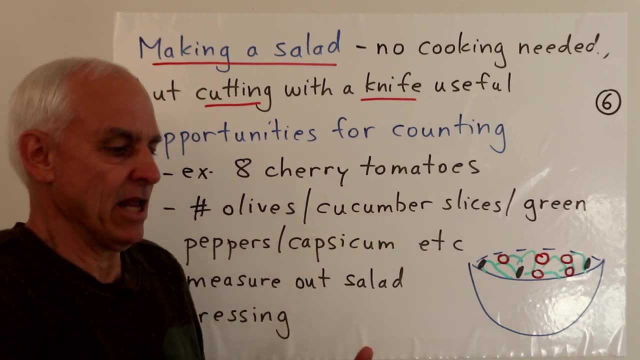 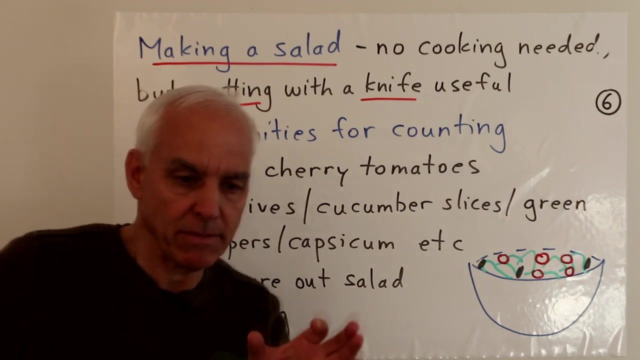 tomatoes, maybe a certain number of olives, or cucumber slices or green peppers called capsicum in australia. so you know there's. there's a counting aspect in making a salad. perhaps you can make it kind of fun, and then finally we might measure out some salad dressing. you know, maybe a certain amount. 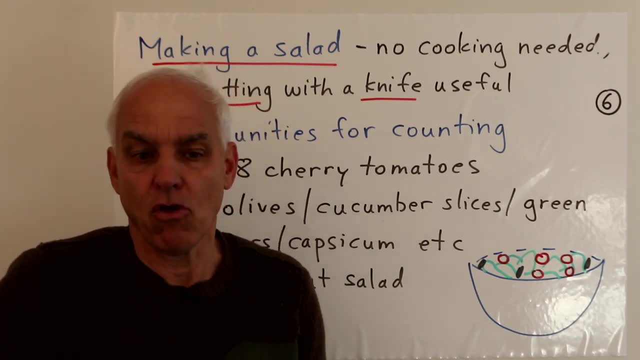 maybe a tablespoon of salad dressing or maybe even some some small volume of salad dressing. if you have a small, you know, a quarter cup or something like that, and then you have a salad and then you can divvy it up amongst the people at the table and there. 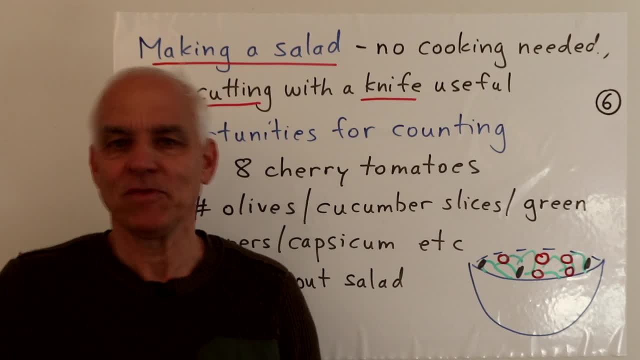 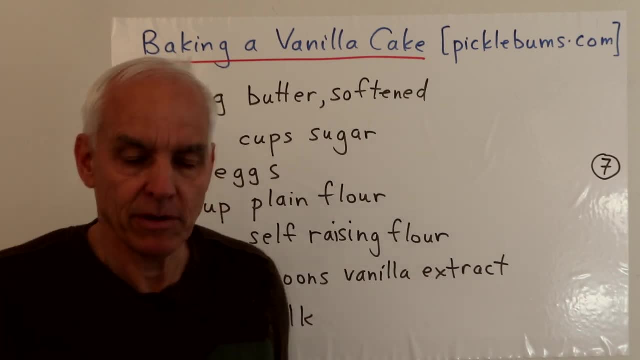 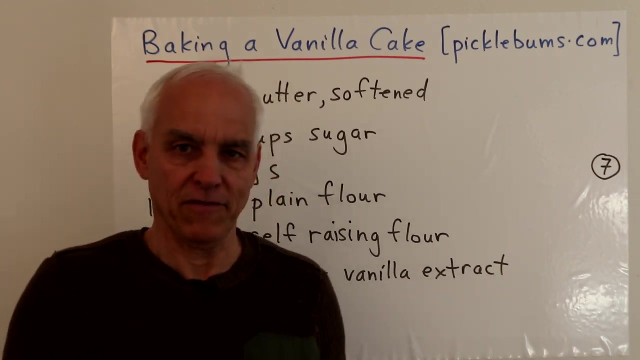 the child has contributed a little bit of arithmetic into making a healthy lunch. okay, basically, maybe, as an yeti, the dear acordia grated first they'll be making ainenkuh, and then you thought, hey, i've got another piece. i'll set up a new box in front of me to eat. 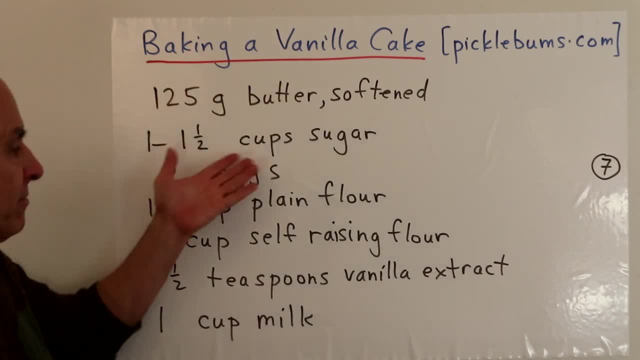 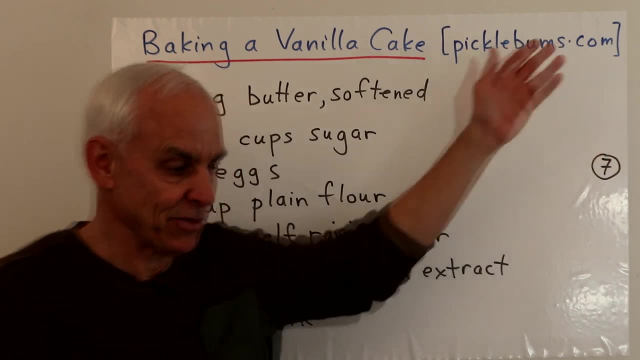 let's take a look around out. so let's see what lunch looks like. here we have our vegetables, here we have cancelled loss, fi, eap, and then if we switch to apples, it's like these little little endure pertinent. already bird got immediately plank. have a lot better milk餌. 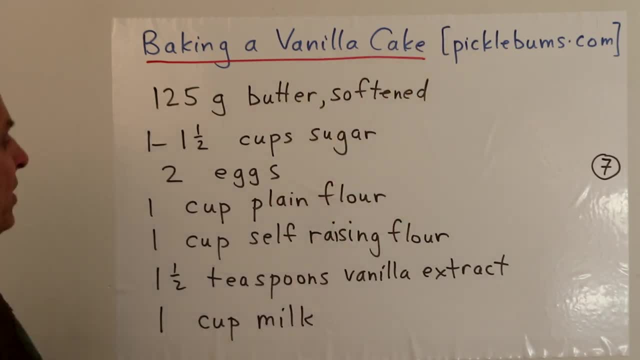 baking a vanilla cake that she, she gives us. okay, so have a look. these are the ingredients and they're listed. okay, so there's 125 grams of butter which are softened, so we've left it out a little bit. one to one and a half cups sugar: i would air towards the lesser amount, because sugar. 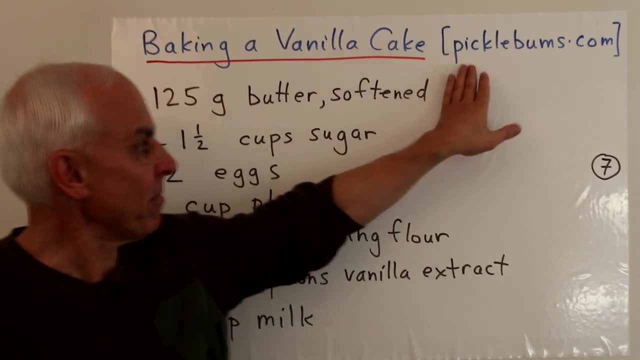 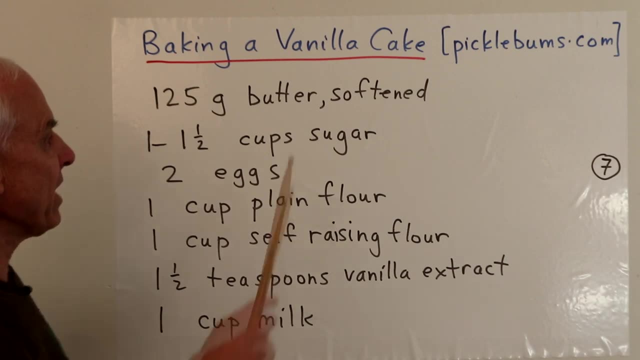 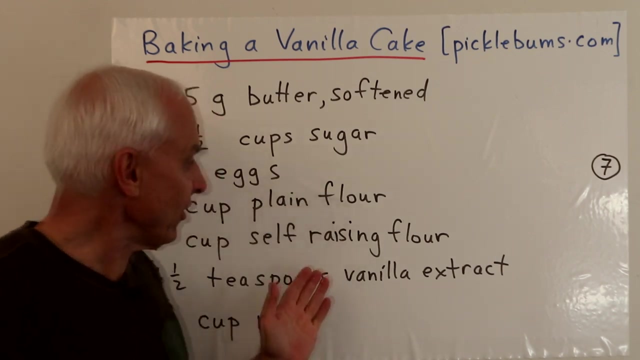 recipes, taking a recipe from the internet, from pickle bums calm place, where they discuss fun things like this, and here is a recipe for baking a vanilla cake that she, she, gives us. okay, so have a look. these are the ingredients and they're listed. okay, so there's a hundred twenty five grams of butter. 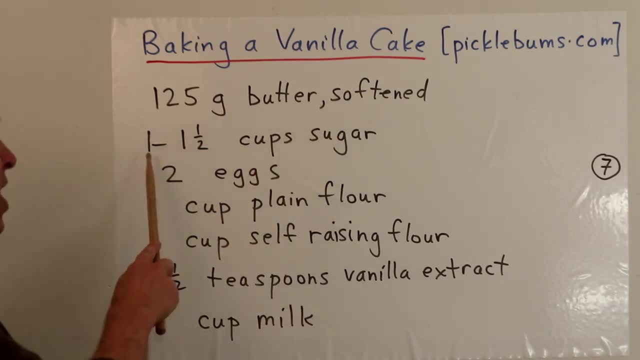 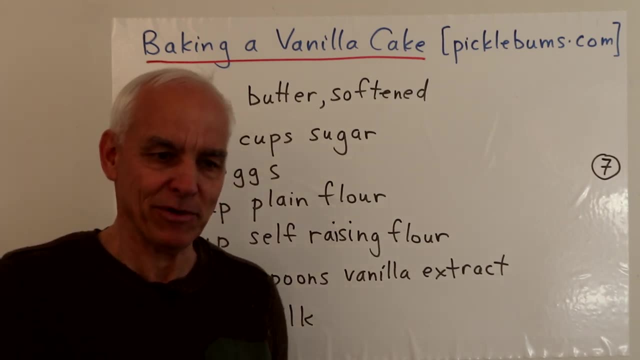 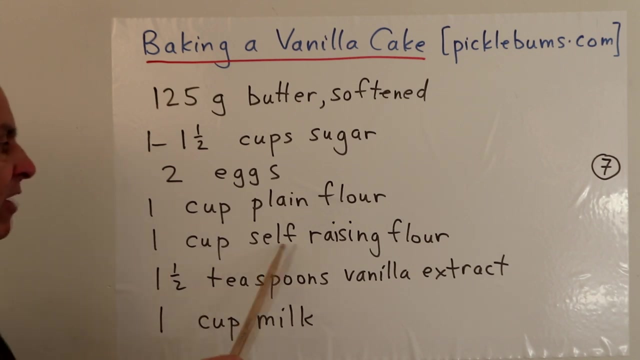 which are softened. so we've left it out a little bit. one to one and a half cups sugar. I would err towards the lesser amount, because sugar should be avoided if possible, or reduced at least, but up to taste. two eggs, one cup of plain flour, one cup of self-raising flour, circumventing. 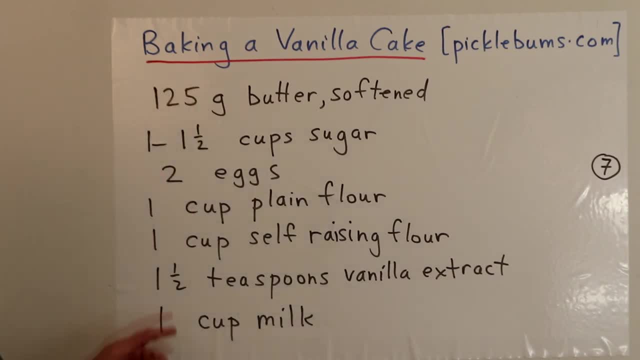 if possible, and one cup of plain flour. one cup of self-raising flour- circumventing if possible- and one cup of plain flour. one cup of self-raising flour, need for baking soda and baking powder, and maybe one and a half teaspoons of vanilla extract, because it's going to be a vanilla cake- and one cup of milk. so 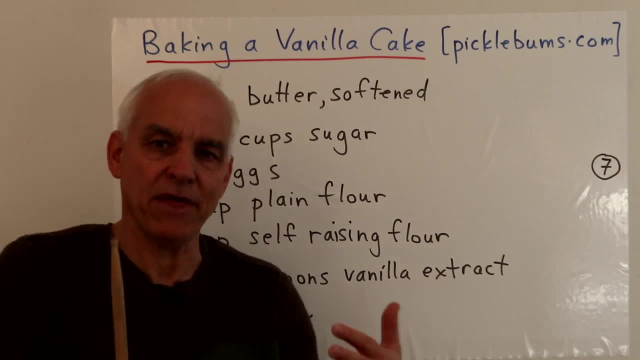 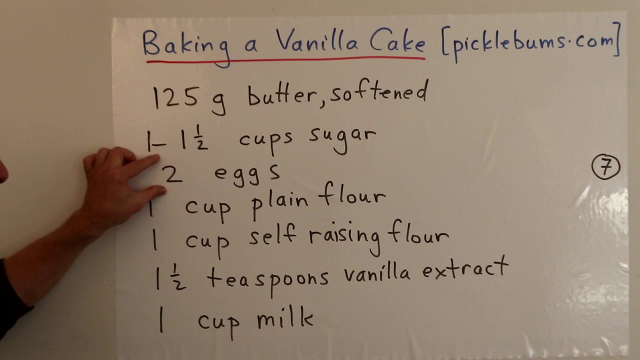 with this. the first order business would be to gather these ingredients, or, before we start, we're going to gather the ingredients and lay them out and make sure that we have the right things, okay. so there's obviously weights involved here, and often also volumes as well as quantities. 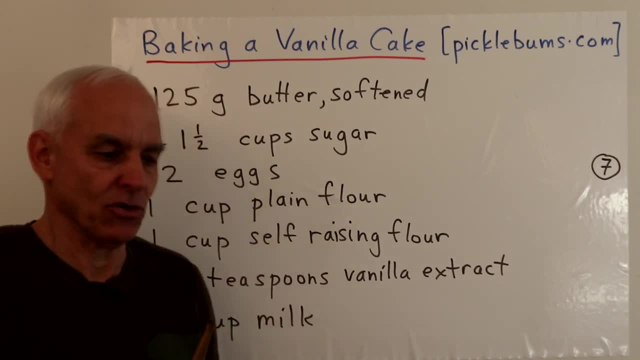 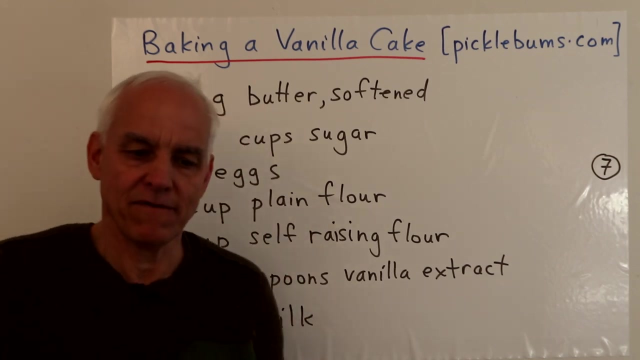 and you know this is a great place to, to be measuring and to, to, to weighing perhaps, and getting a sense of how much does one cup of flour you know actually amount to. so this is a, this is a recipe like. this is actually a very mathematical. they're illustrating the power of the importance of facility with. 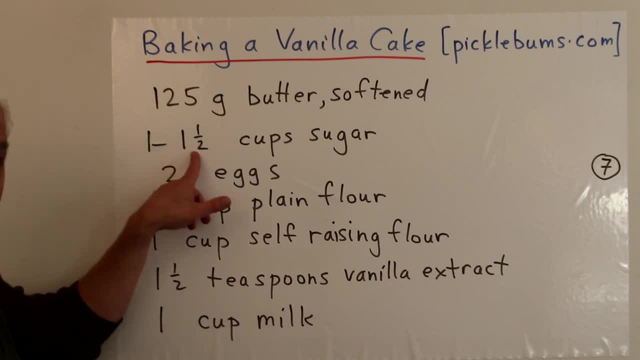 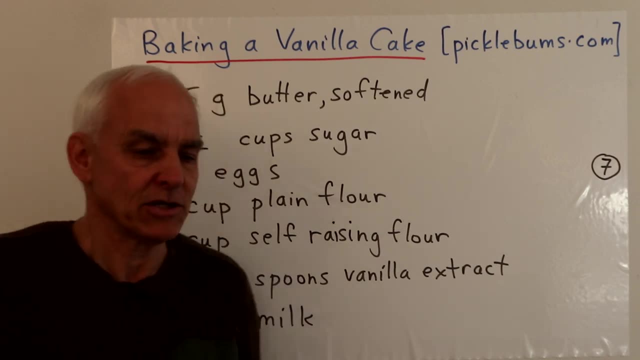 basic arithmetic in particular, there's a one and a half here. okay, we haven't officially talked about that, but you can try to figure that out if you want to try to explain to your, your child, what that means. so we don't need a theory of fractions. this is just a half. it's a very special kind of thing represented by 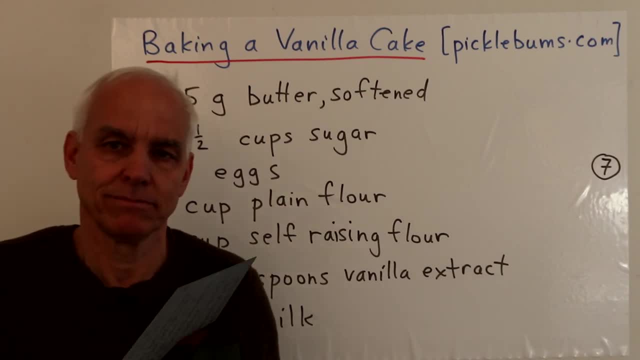 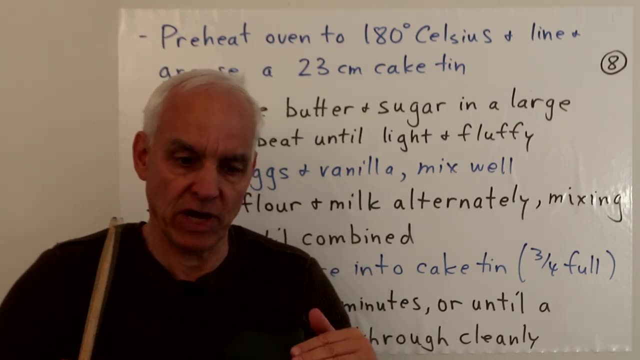 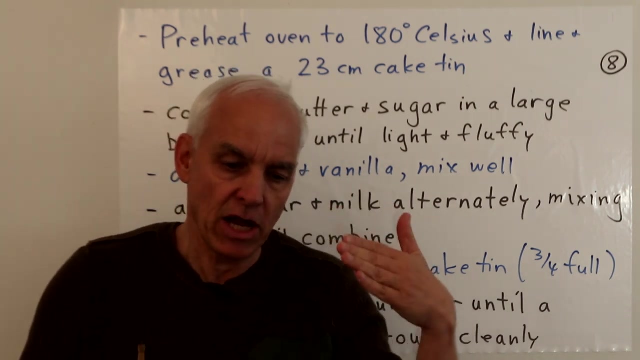 a half a cup, measuring cup. okay, so we have the ingredients for our cake and now we actually have to bake the cake, and for that we have the recipe, which is a series of instructions, step-by-step instructions, and that's very informative and important: that a child recognizes that what we're doing here is we're 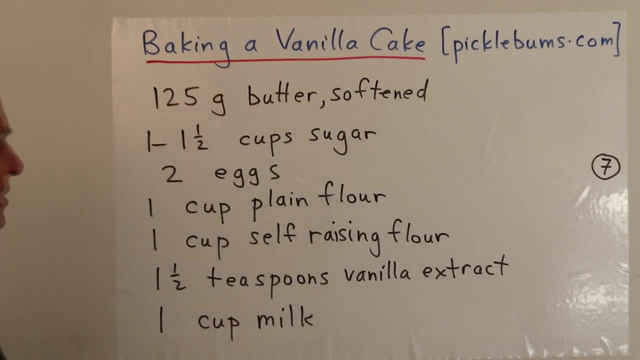 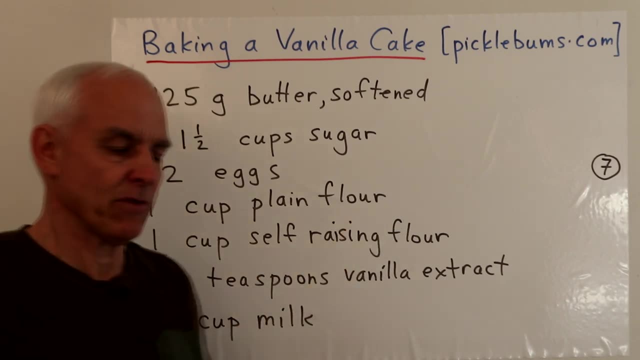 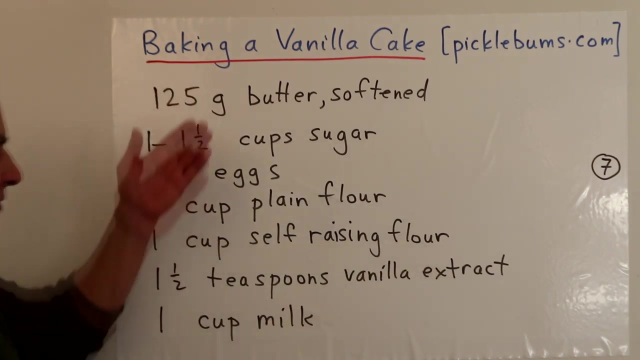 should be avoided if possible, or reduced at least, but up to taste. two eggs, one cup of plain flour, one cup of self-raising flour, circumventing the need for baking soda and baking powder, and maybe one and a half teaspoons of vanilla extract, because it's going to be a vanilla cake. 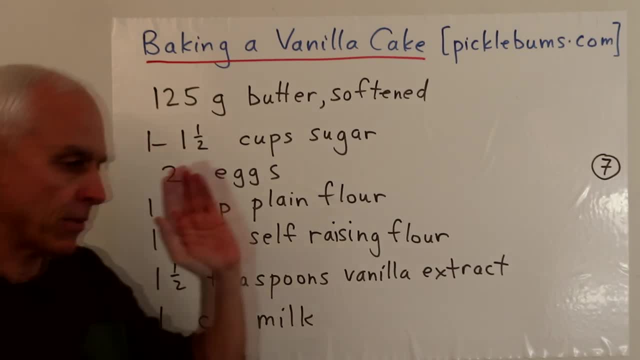 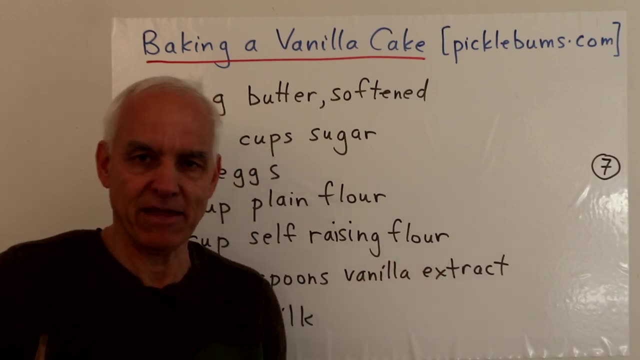 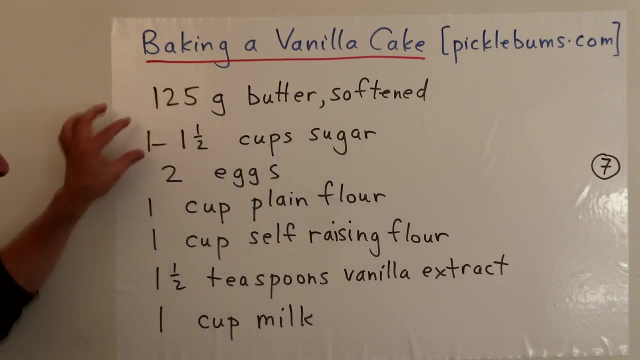 and one cup of milk. so, with this, the first order of business would be to gather these ingredients, or, before we start, we're going to gather the ingredients and lay them out and make sure that we have the right things, okay, so there's obviously weights involved here. 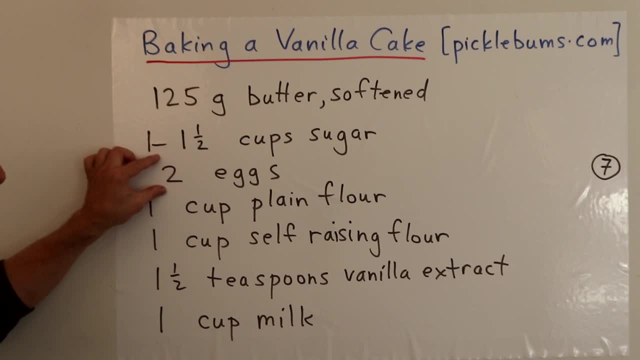 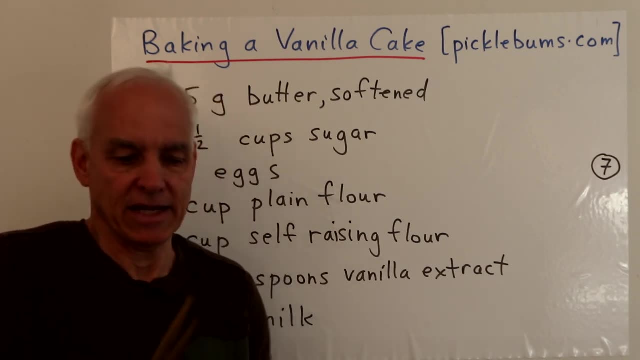 and often also volumes as well as quantities and, uh, you know, this is a great place to, to be measuring and to, to weighing, perhaps, and getting a sense of how much does one cup of flour, you know, actually amount to. so this is a, this is a recipe like. this is actually a very mathematical sort of illustrating. 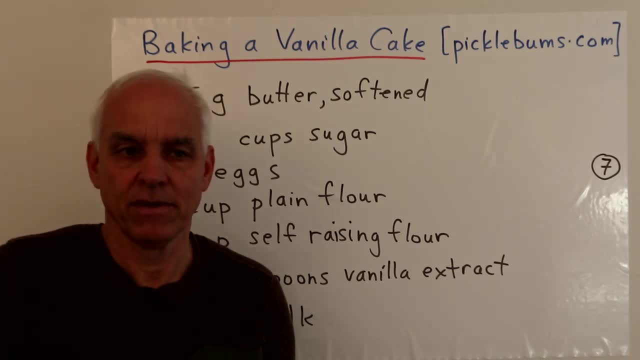 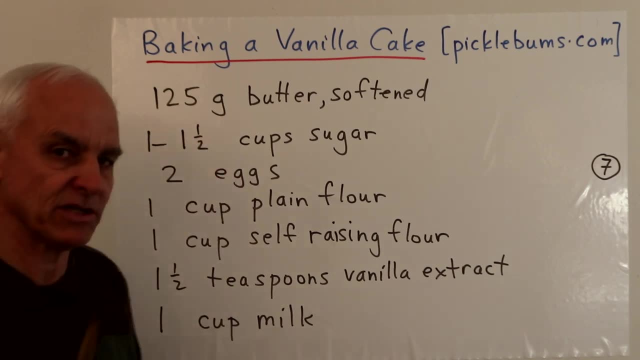 the power of the importance of facility with basic arithmetic in particular. there's a one and a half here. okay, we haven't officially talked about that, but you can try to explain to your, your child, what that means. so we don't need a theory of fractions. this is just a half. it's a very special kind of. 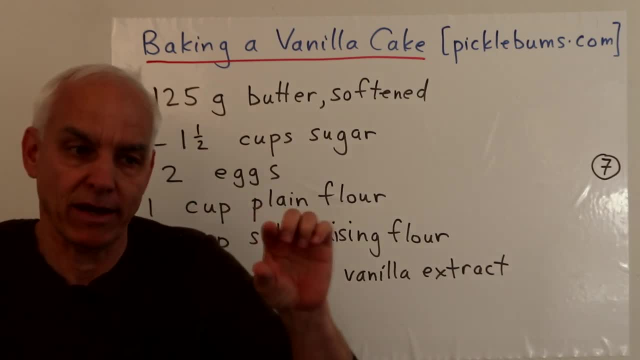 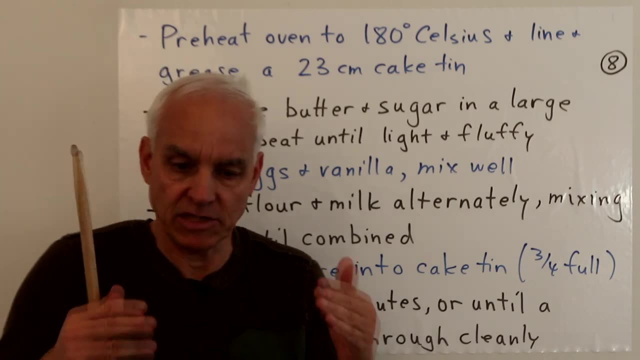 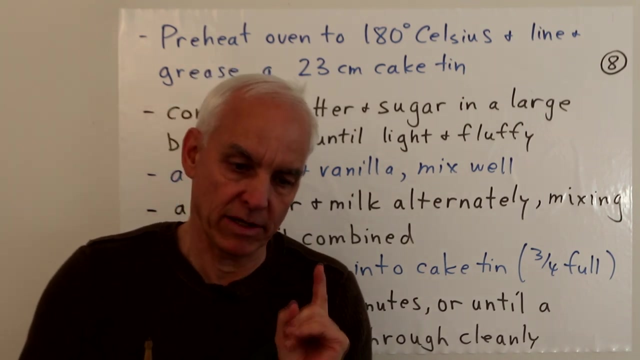 thing represented by a half a cup measuring cup. okay, so we have the ingredients for our cake and now we actually have to bake the cake, and for that we have the recipe, which is a series of instructions, step by step instructions, and that's very informative and important that. 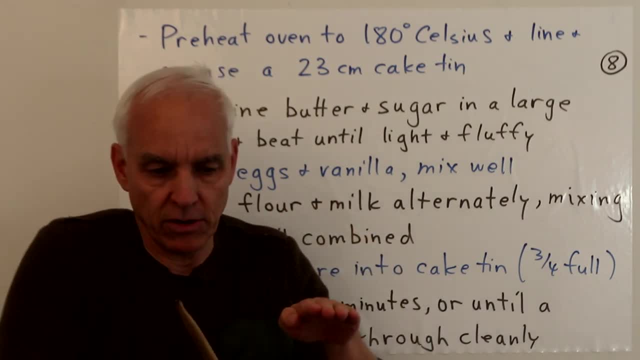 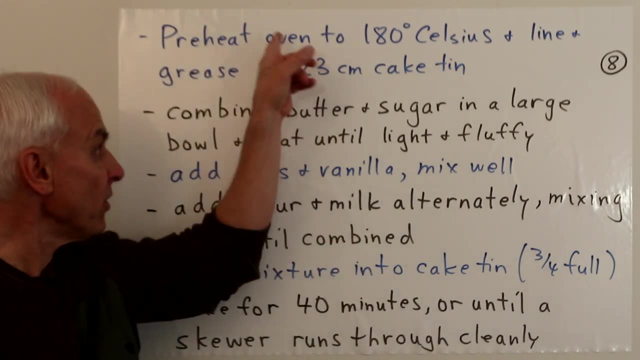 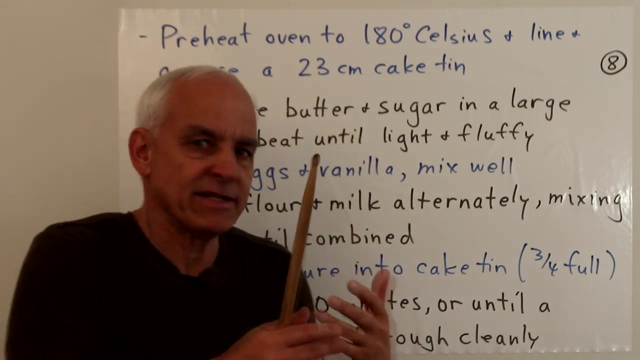 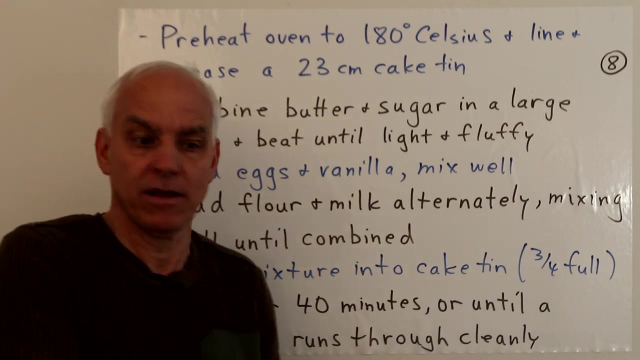 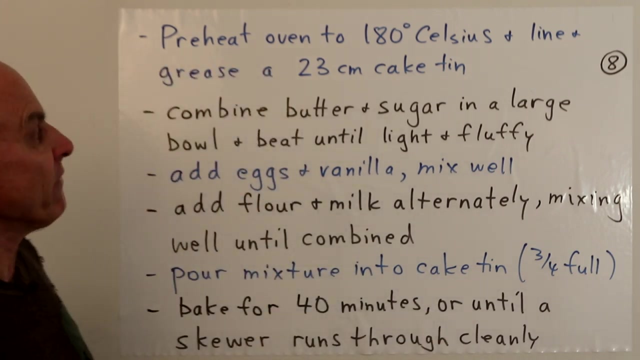 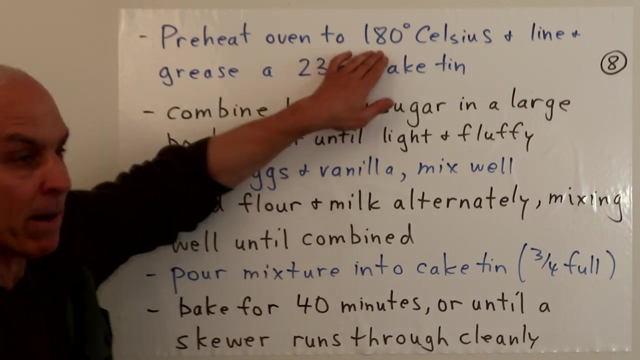 children and lots of speak in our library with this course using. so preheat the oven to 180 degrees celsius and line and grease a 23 centimeter cake tin. so i'm taking this from the internet, from that reference i already gave you. okay, so there is some temperature. 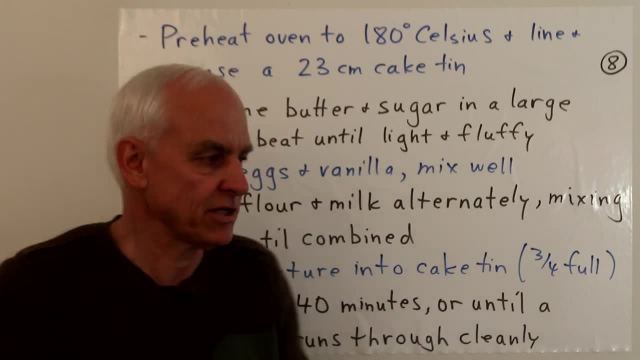 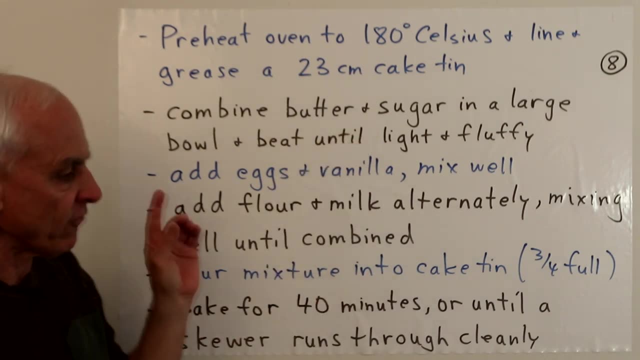 doing a number of things in the correct order. it's not just that we can do all these things willy-nilly. we have to do this one first, and then this one, and then this one, and so on. okay, and we also have to be relatively precise about the 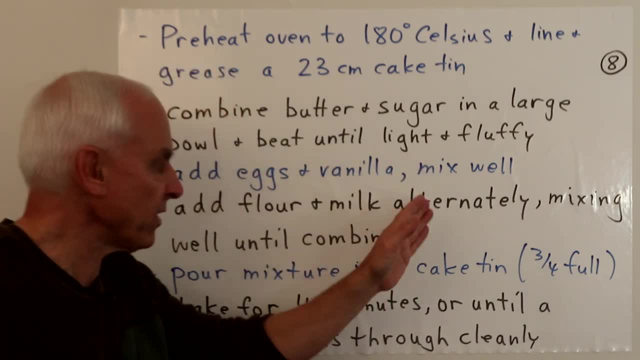 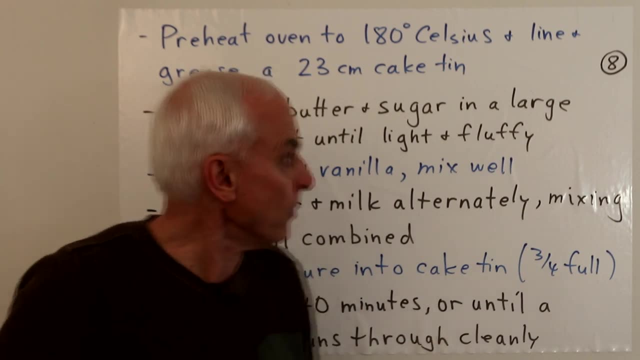 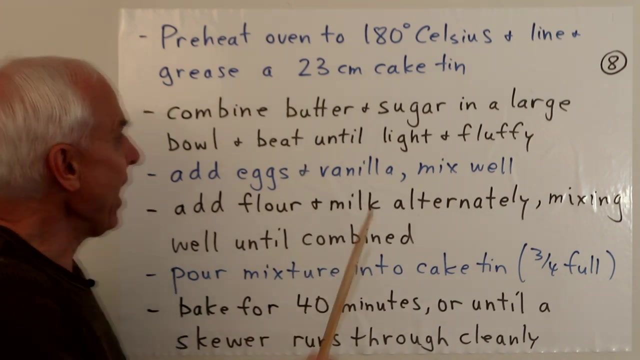 meanings of the words here. right, we have to understand everything that's being said so that we do things correctly, because if we make some crucial mistake, then the cake is not going to taste any good. okay, so preheat the oven to 180 degrees Celsius and line and grease a 23 centimeter cake tin. so I'm taking this from the 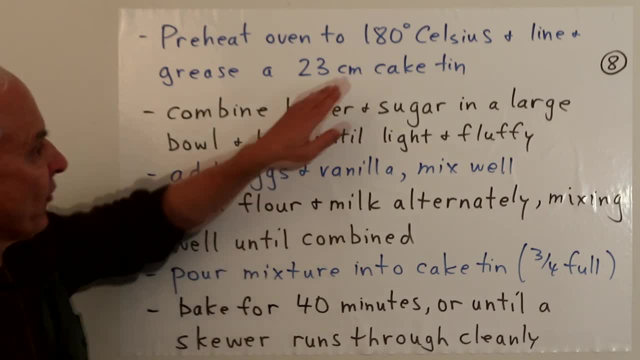 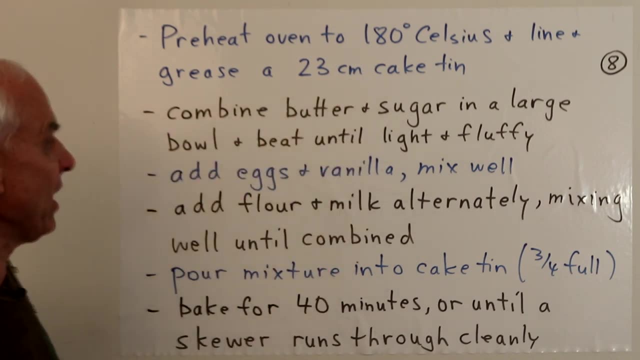 internet from that reference I already gave you. okay. so there is some temperature involved here. we will read something on the oven and there's also a measurement here in terms of the size of the cake tin. okay, now we're going to start using the ingredients that we have laid out in front of us combined: the 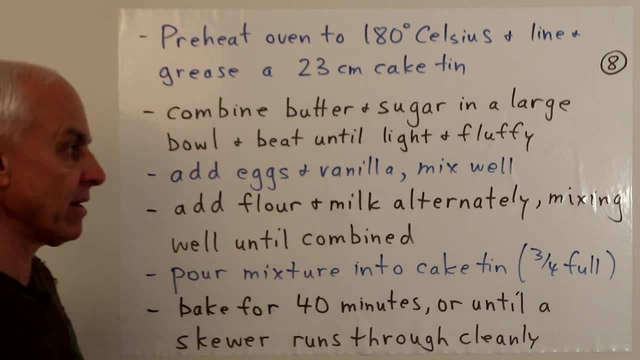 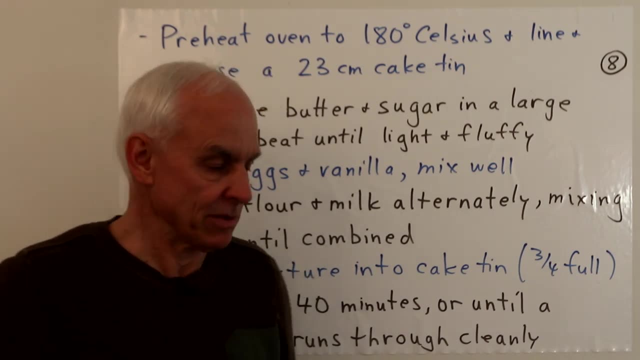 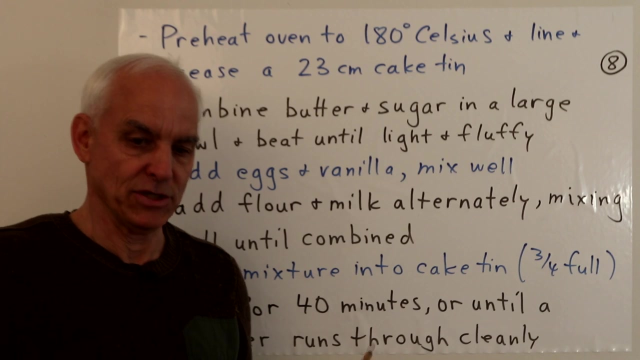 butter and sugar in a large bowl and beat until light and fluffy- in the olden days with a hand beater. these days, with electronic mixer, is a lot easier. then add eggs and vanilla and mix well, okay, so we have to crack the eggs and put them in. so that's kind of fun. the kids like to do that and we mix. 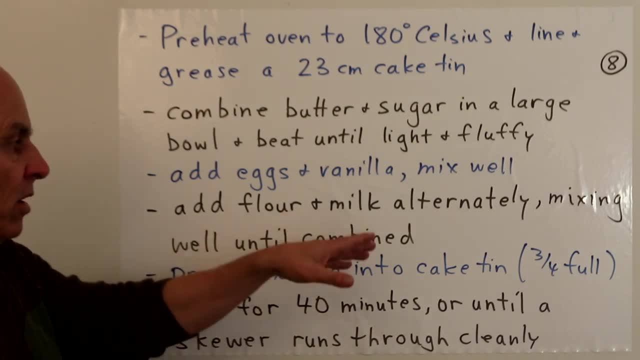 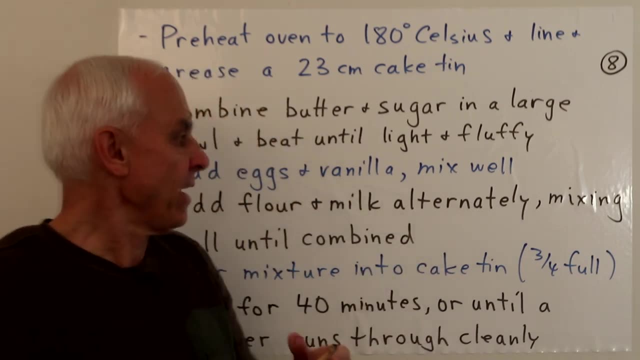 that. well, now we have to add the flour and the milk alternately. so we have this flour and the milk. we add a little bit of flour, a little bit of milk mix that, a little bit more flour, a little bit more milk mix that and so on, until eventually we have all the flour and milk from that side of the pot. 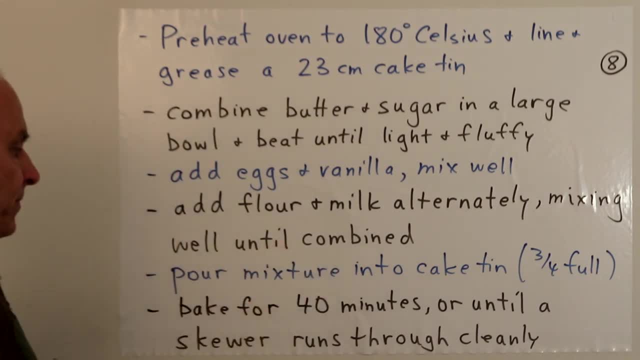 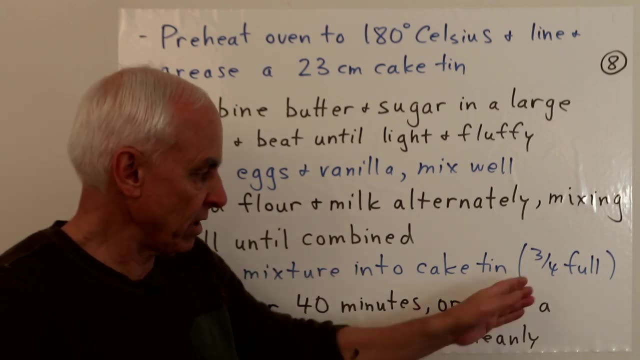 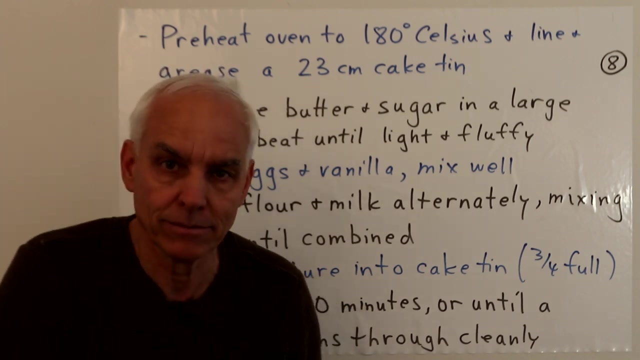 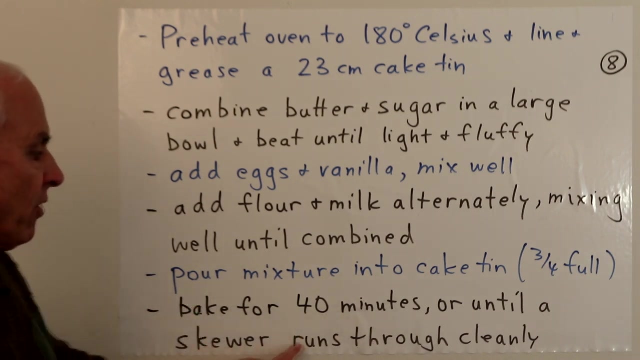 there and it's well mixed, so everything is combined. so we have this well combined mixture which we then pour into the cake tin and it should be perhaps around three quarters full, not all the way up to the top, because the cake is going to rise, hopefully. okay the instruction. then bake for 40 minutes or until a skewer runs through. 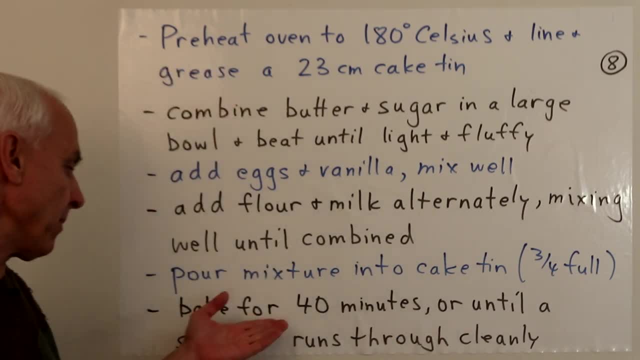 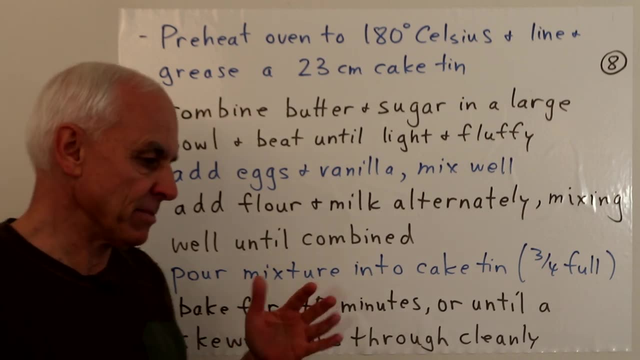 cleanly okay. time for baking is always a little bit of an issue in my limited cooking baking experience, because sometimes it's hard to gauge what the temperature of your oven really is. so maybe some some judgment is required here, and so this test of you know running a skewer through. 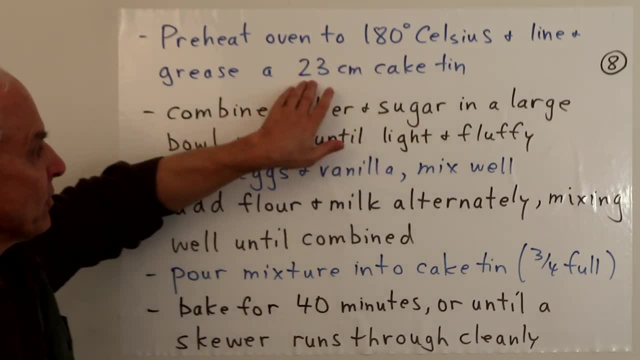 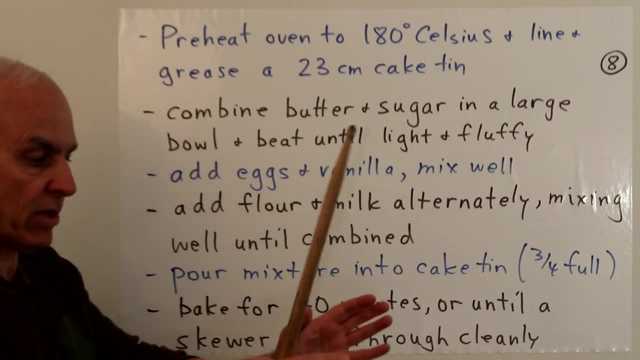 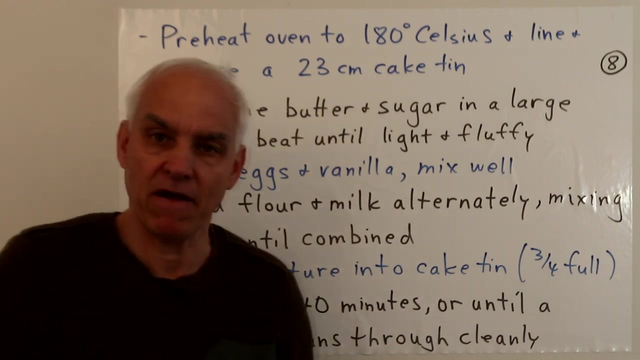 involved here to be able to read something on the oven, and there's also a measurement here in terms of the size of the cake tin. okay, now we're going to start using the ingredients that we have laid out in front of us. combine the butter and sugar in a large bowl and beat until light and fluffy. 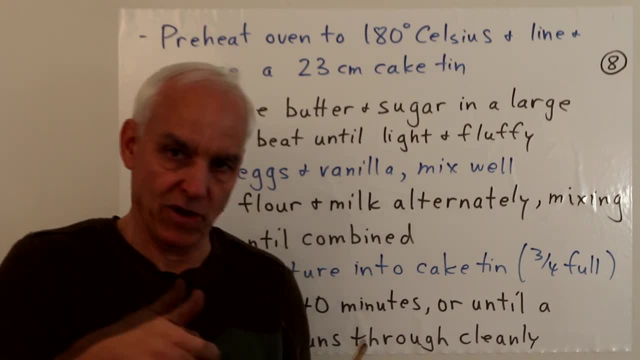 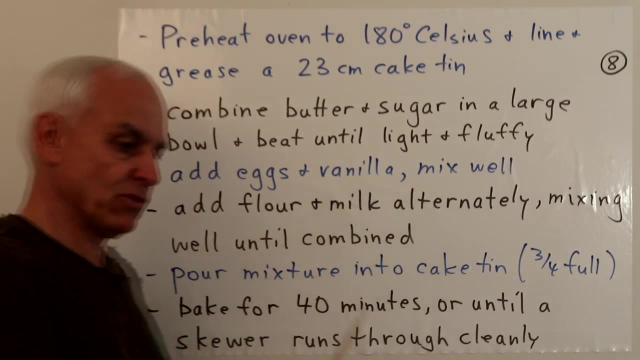 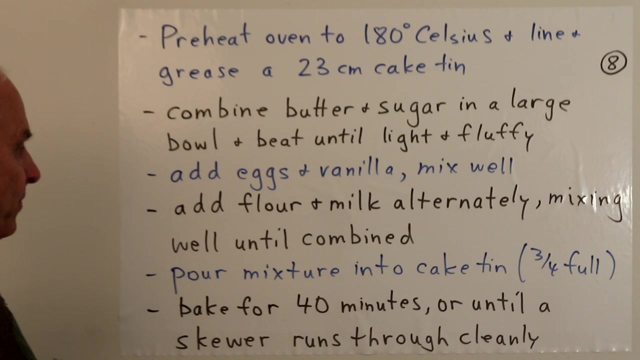 in the olden days with a hand beater. these days, with electronic mixer, is a lot easier. then add eggs and vanilla and mix well. okay, so we have to crack the eggs and put them in. so that's kind of fun. the kids like to do that and we mix that well. now we have to add the flour and the. 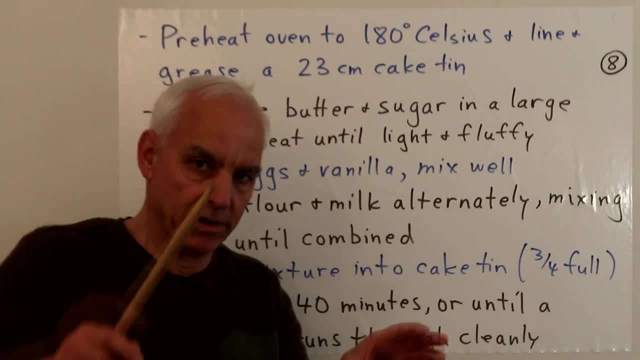 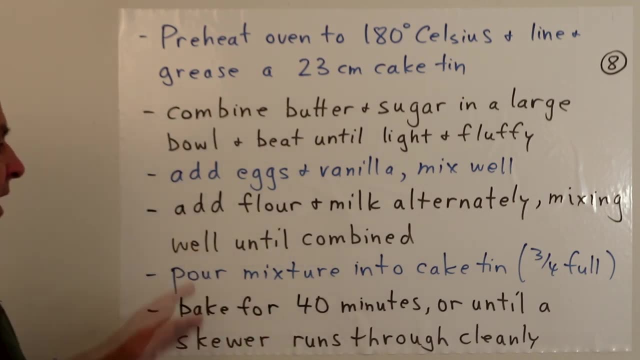 milk alternately. so we have this flour and the milk. we add the flour and the milk and we add a little bit of flour, a little milk- mix that, a little bit more flour, a little bit of more milk- mix that and so on, until eventually we have all the flour and milk in there and it's well mixed. 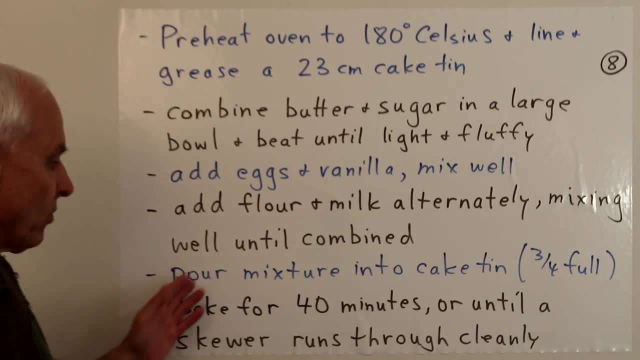 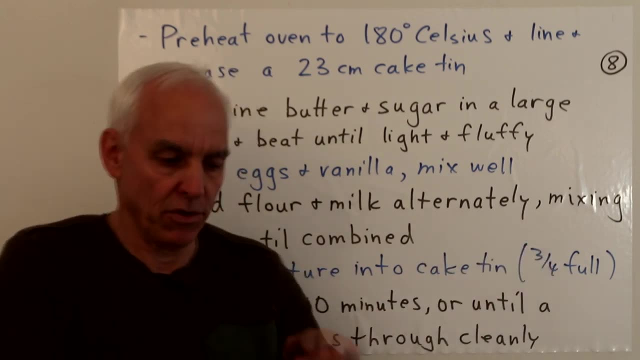 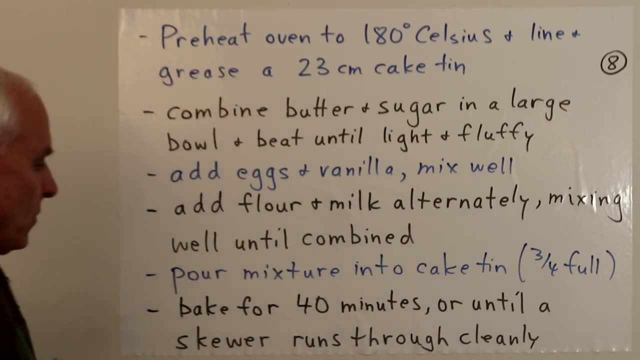 so everything is combined. so we have this well combined mixture which we then pour into the cake tin, and it should be perhaps around three quarters full, not all the way up to the top, because the cake is going to rise, hopefully. okay the instruction then bake for 40 minutes. 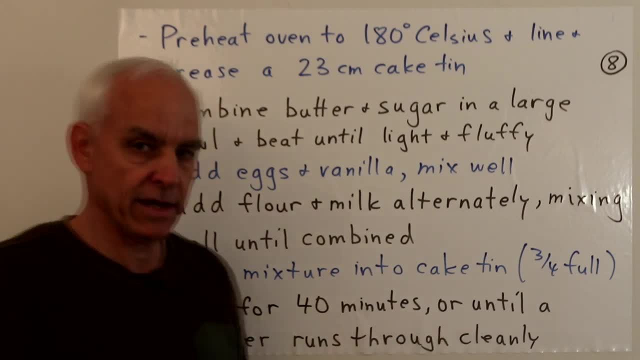 or until a skewer runs through cleanly okay. time for baking is always a little bit of an issue in my limited cooking baking experience, because sometimes it's hard to gauge what the temperature of your oven really is. so maybe some some judgment is required here, and so this test of you know. 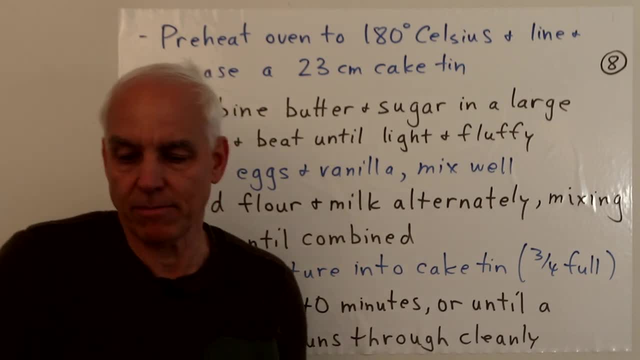 running a skewer through it, and if it comes out cleanly, then it's done. so that might be helping you there again. you have to be concerned with safety issues here, because we're talking about an oven, talking about taking the cake out. you know you need gloves and you have to be very careful, and i would only recommend that. 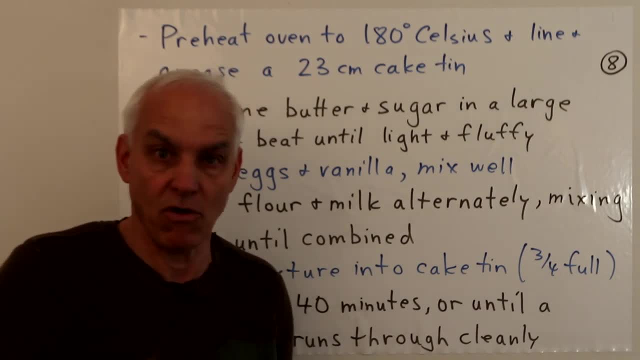 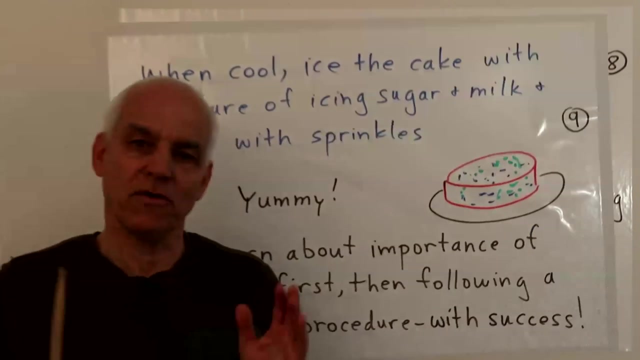 more, more senior students are going to be involved in that aspect of things. okay, but nevertheless, once a student's 12 years old, they're perfectly capable of doing that with some some supervision and uh and care and explanation. all right. so final instruction when cool, so you've. 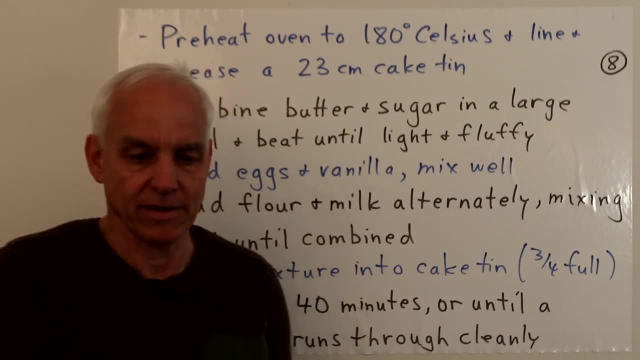 it, and if it comes out cleanly, then it's done. so that might be helping you. there again, you have to be concerned with safety issues here, because we're talking about an oven, talking about oven, so we're talking about oven, so we're talking about ovens. there there are some things. 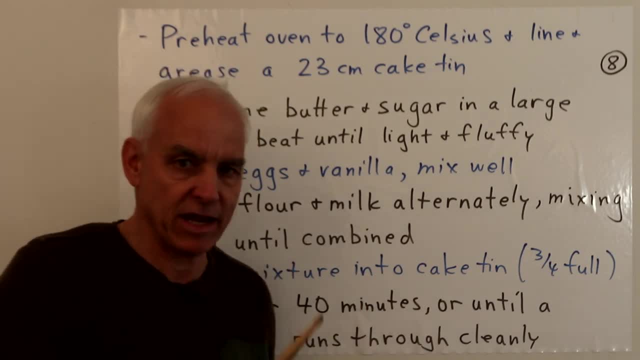 there again. you have to be concerned with safety issues here, because we're talking about an oven, about taking the cake out. you know you need gloves, you have to be very careful and I would only recommend that more more senior students are going to be involved in that aspect of things. okay, but nevertheless, once a student's 12. 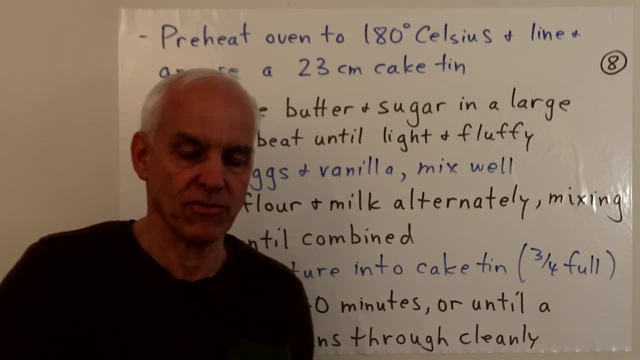 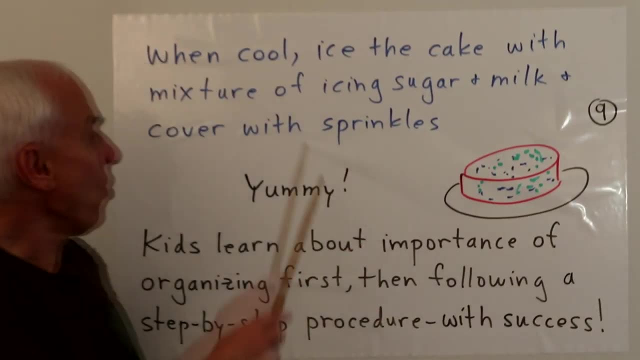 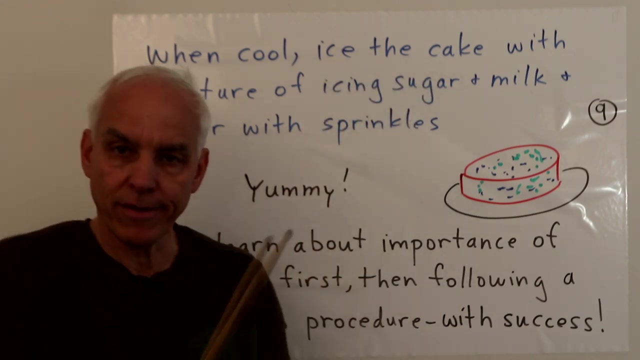 years old. they're perfectly capable of doing that with some some supervision and and care and explanation. alright, so a final instruction: when cool, so you've taken the cake out, let it cool, ice the cake with a mixture of icing sugar and milk and, if you like, cover it with sprinkles and you get a yummy vanilla. 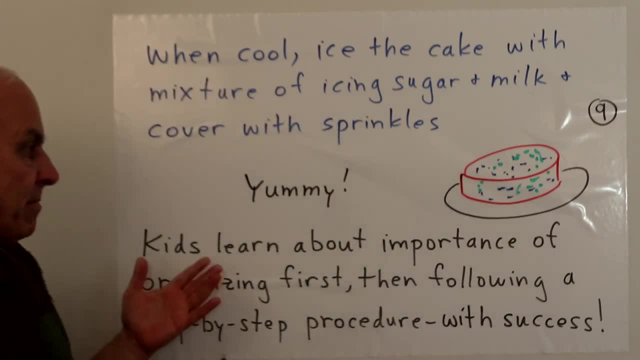 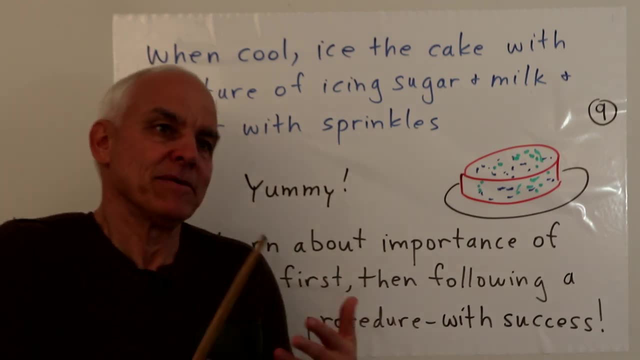 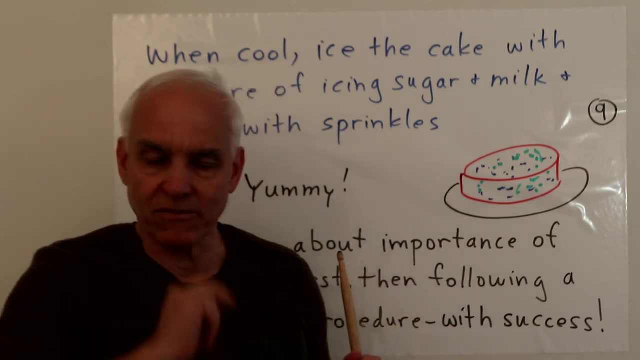 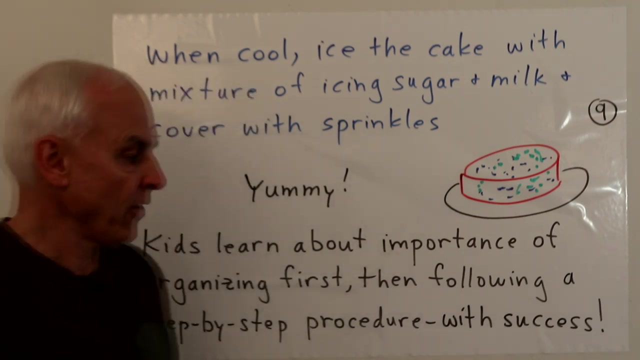 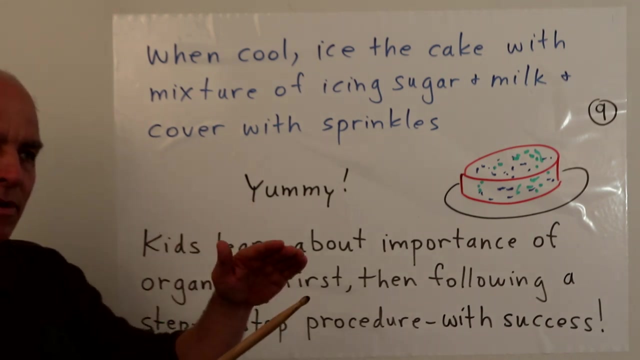 cake. okay. so this illustrates the importance of following instructions, of being careful about ingredients, kind of a simple but important applied mathematics connecting theoretical arithmetic and a little bit of geometry and and and with very practical, important matters- food, food preparation. so this is a also kind of a guide: the importance of being able to follow step-by-step procedure. 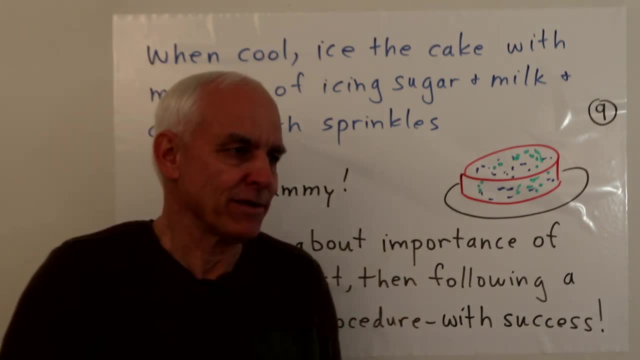 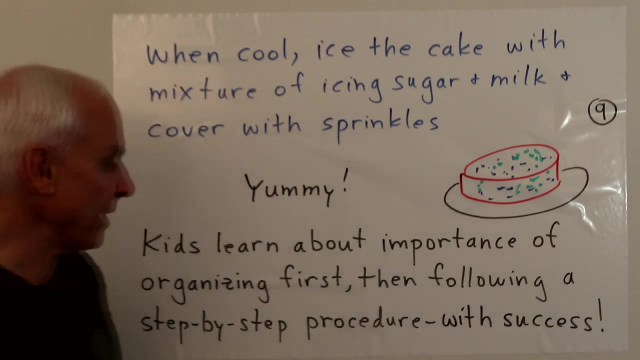 which is actually what we do later on in mathematics. even with like computers, like a computer program, it's really the same kind of thing. we have a step-by-step procedure. we're going to work through it carefully and do everything exactly as it's stated and and then hopefully at the end of it, you've done things correctly. 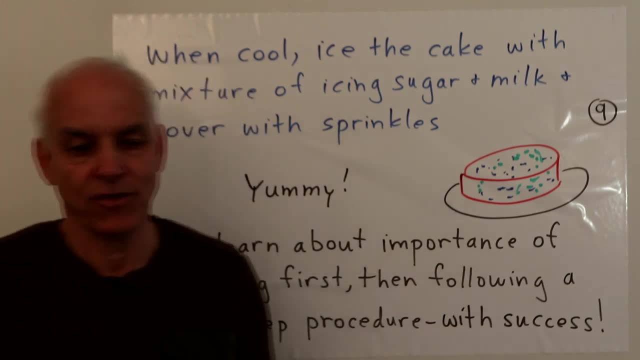 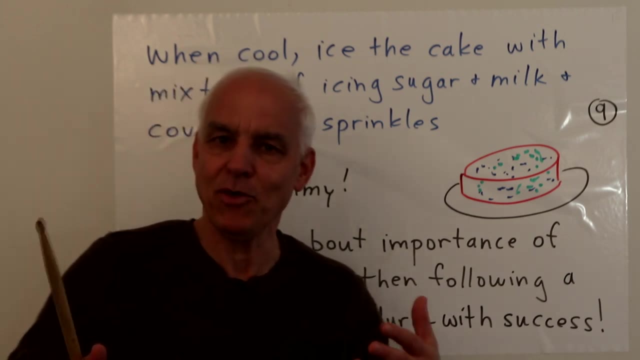 and you're rewarded with success. so this is a very powerful way of getting students happy with their arithmetical skills, making them feel that, yes, mathematics does connect with the real world and it's important to know how to measure things, how to weigh things, how to count things, how to put those things.